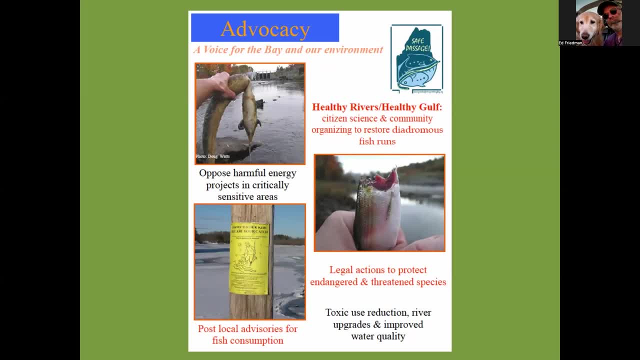 And other things that come along that need a strong voice, really the prime mover years ago in stopping a proposed major hydro tidal generation plant for right smack in the middle of the Chubbs, which is what drains the bay and ends up at the end of Scoggin and kind of back to Detroit Bay. 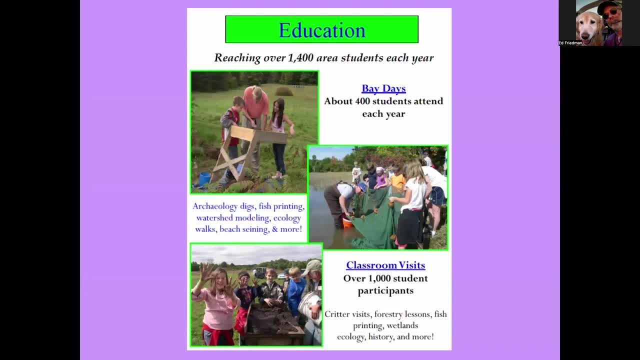 Now that COVID is more or less in the rear view mirror. we're used to it anyway. We're used to it anyway. We're used to it anyway. Back in fairly full swing with our education program and we'll be planning a spring bay day, May 14th. if anyone's interested and wants to help, shoot me an email or give me a call 666-3372,. find that information on the website. but we'll be having a whole lot of kids from all around the bay outside having all kinds of good fun, getting dirty and learning about the bay and the environment. 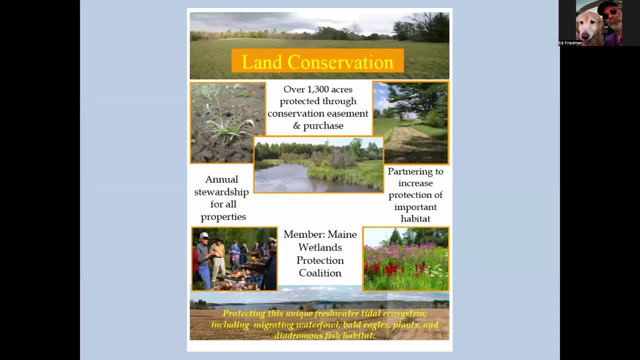 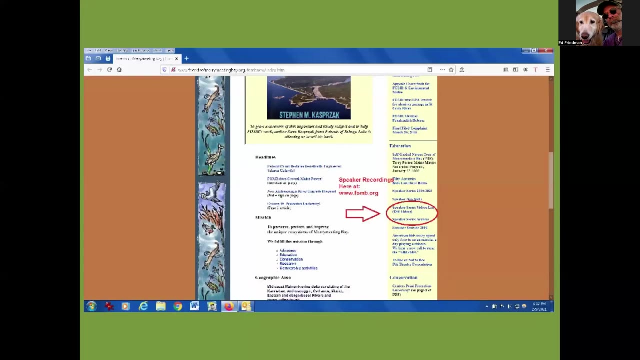 Protected over 1,500 acres of land By now around the bay, mostly wildlife habitat, valuable wildlife habitat. That's our focus, as opposed to trails and such like that. If you think the program is good tonight and you want to watch this one or refer people to it or any other older ones we've recorded which go back about 10 years on our homepage, scroll down on the right under education. you'll see a link to speaker series videos. 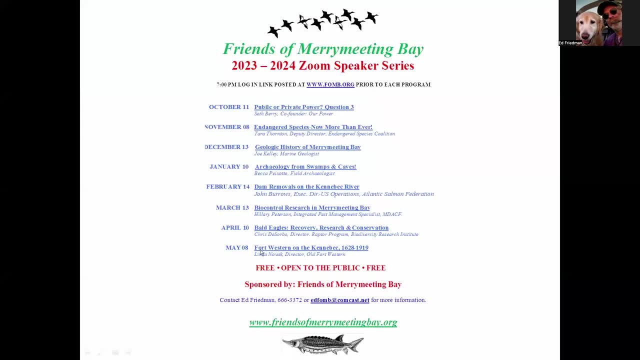 And the season counts, The calendar which we're rapidly running out of next May, and these days are all the second Wednesday of the month. Wednesday evening We- Linda Novak, director of Old Fort Western- will be talking about Fort Western and the Kennebec over quite a spectrum of years, span of years. 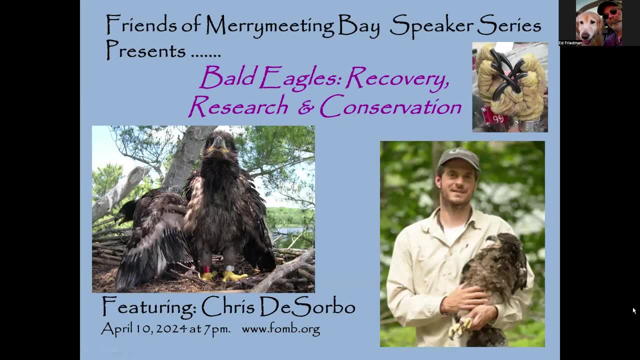 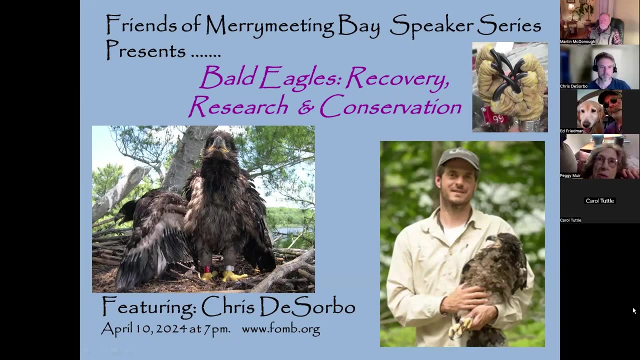 So Chris DeSorbo. Chris joined Biodiversity Research Institute, or BRI, in 1998.. Overseeing a common loon behavior And a major focus of his research is the individual ecology and toxicology study in Maine's Rangeley Lakes region. 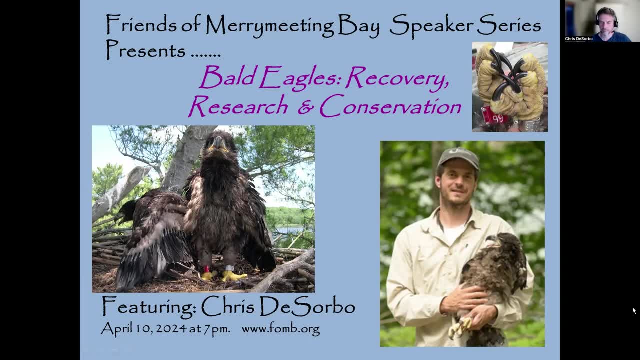 As BRI expanded its mercury research to include other species, the raptor program was born. Through this program, Chris initiated what's now become the most extensive bald eagle sampling and banding effort in Maine's history, And actually I'll throw in that FOMB has probably the most extensive record of eagle nest sampling. 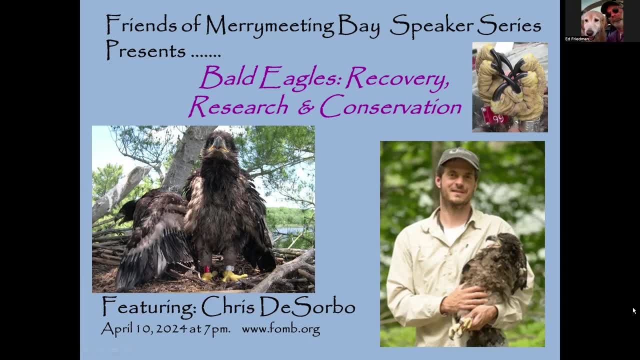 And the FOMB has probably the most extensive record of eagle nest sampling And the FOMB has probably the most extensive record of eagle nest sampling And the FOMB has probably the most extensive record of eagle nest sampling, Eagle nest surveying this area in the state as well. 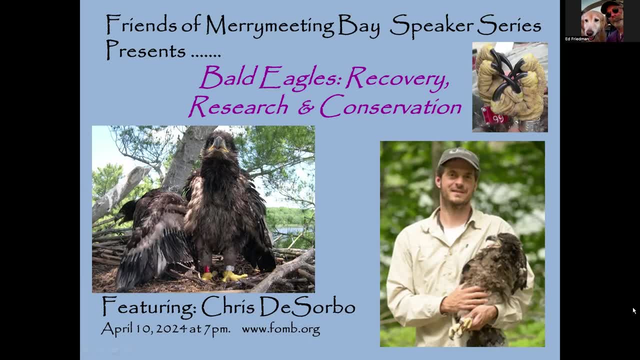 Eagle nesting program. Recent BRI raptor program projects have emphasized various studies of migrating raptors and using individual tracking technologies to inform conservation and management decision-making relevant to bald eagles, peregrine falcons and other raptors. Chris's current projects at BRI include evaluating mercury and lead exposure in adult resident bald eagles. 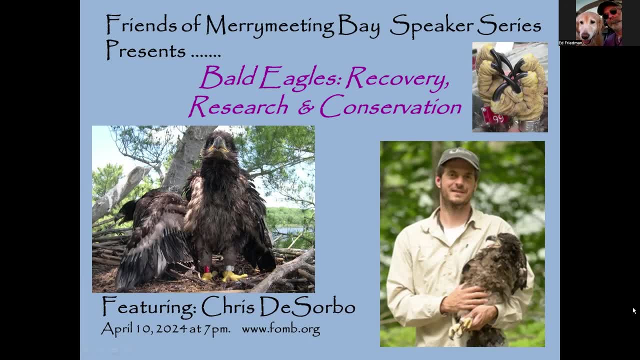 and in the state of Maine And in commonppenes, And assessment mercury exposure and risk with North American migrant raptors. and evaluating the use of offshore wind energy areas along the'mont coast by migrating peregrines and merlins. In addition to raptor work, Chris is overseeing BRI's projects related to wildlife and solar energy development. 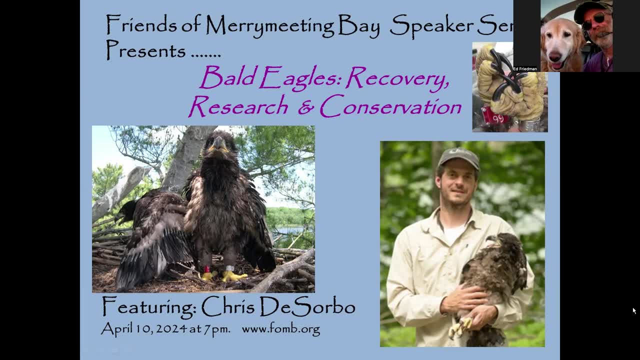 And Chris has a BS in biology from UNH 1996.. uh, and a master's science- environmental studies, conservation biology- from antioch university in 2007.. and with that, uh, i welcome you again, chris. great to finally have you here. 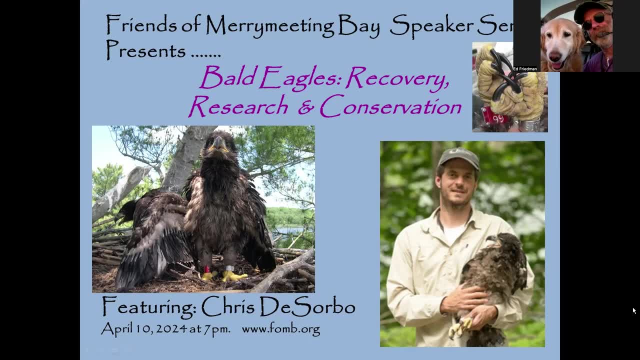 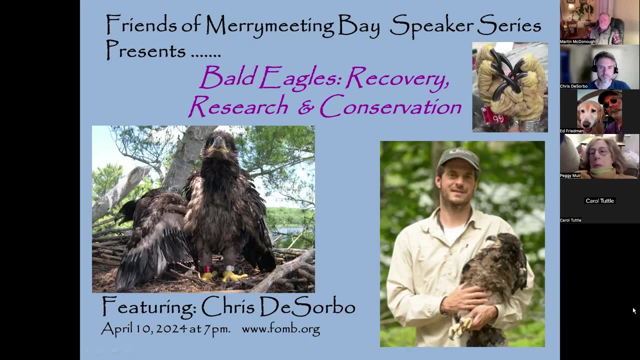 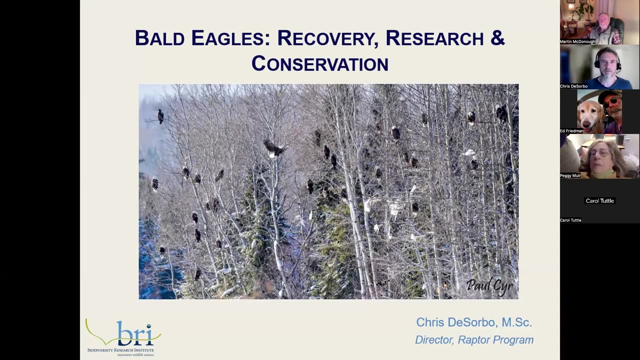 and, uh, you can go ahead and share, share your screen, all right. uh, can you hear me? all right, yep, hear you, okay, and we see your large slides, so you're good to go, friend, okay, good, uh, well, um, yeah, hi everybody. um, so, yeah, i, it's funny, i didn't think. 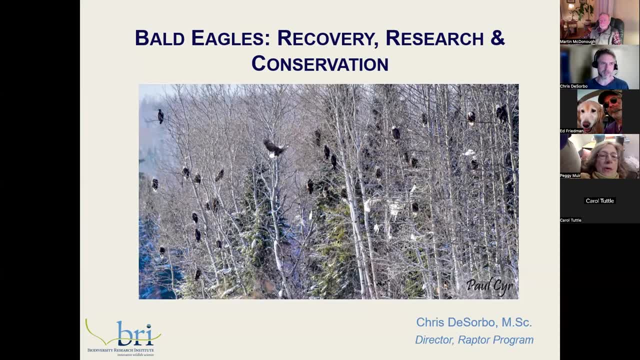 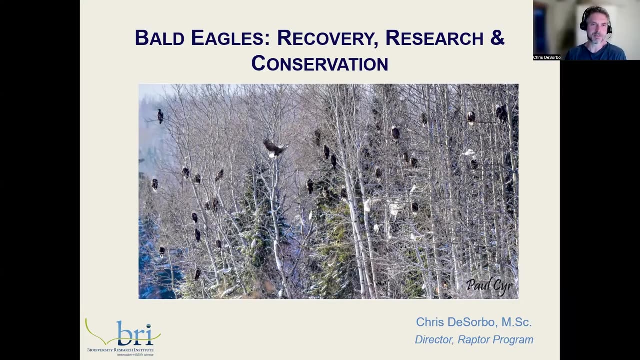 about it till you mentioned it, um, ed. but yeah, i probably met you in like early 2000s doing, uh, bald eagle banding and mercury work and uh, yeah, there's a massive gap in in time between that experience and um us going out again this year. so it's kind of cool to to be talking now um, so let's see here uh. 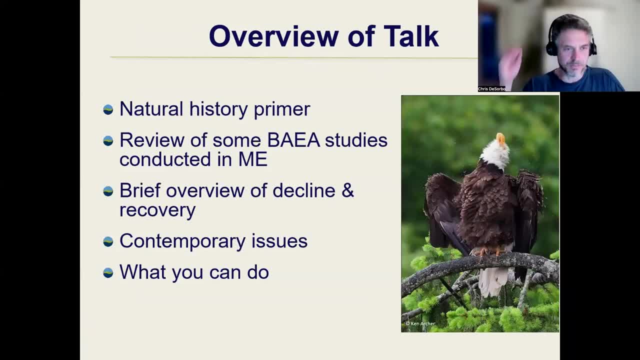 so i'm gonna give you a little overview of what i'm going to talk about here. um, what i thought i'd do is just give your standard textbook natural history primer on eagles. um, but as a part of that, what i'm gonna try to do is work in a summary of some of the different studies that have happened. 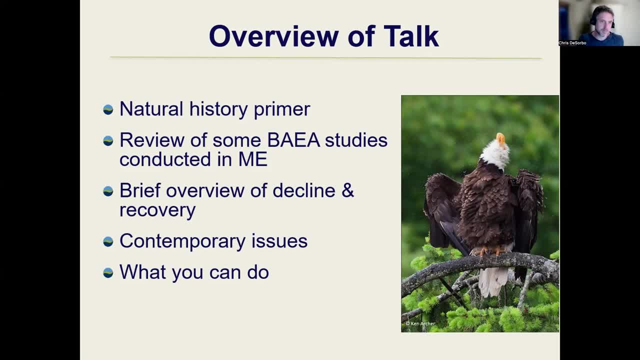 in maine specifically, um, because maine actually is, is unique in the broader um research context, um, and so i'm going to interject some detours to talk about some of the studies that have happened here, um, and then pivot back to a talk about just the decline in recovery of eagles, because it would 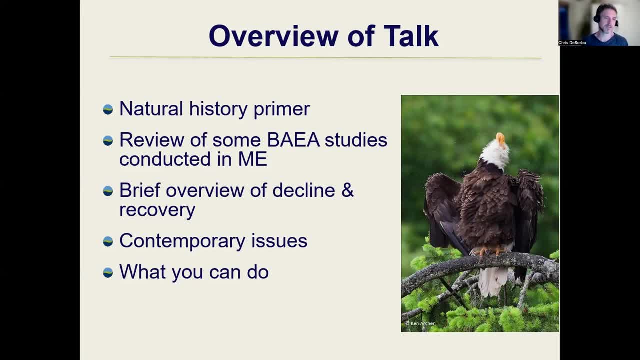 be- uh, you'd be remiss to not do so- and then talk about some of the more, um, kind of contemporary issues that are, uh, that come up in the future. so i'm going to start off with a little bit of a summary of some of the studies that have come up with, related with regard to eagles, and then 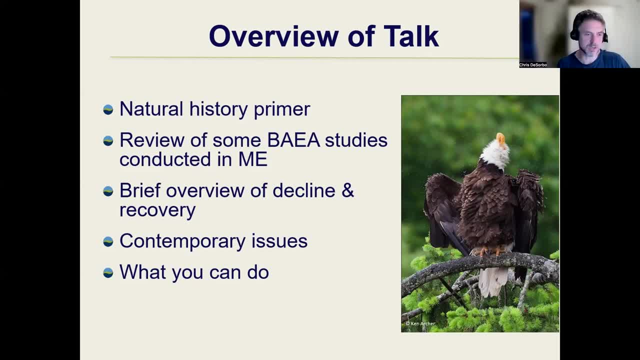 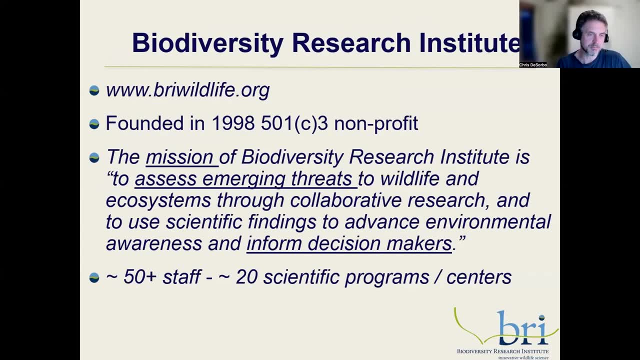 we'll kind of finish up with just some things you can do. um, so, um. that's the plan. so, yeah, i work for bri. um, you can check out that website if you wanted to learn more about us. we're a 501c3 non-profit founded in 1998, and the mission statement of the organization is up there. um to assess emerging threats to wildlife and eagles, and we're going to talk a little bit about some of the studies that have come up with regard to eagles, and we're going to talk a little bit about some of the studies that have come up with regard to eagles and we're going to talk a little bit about. 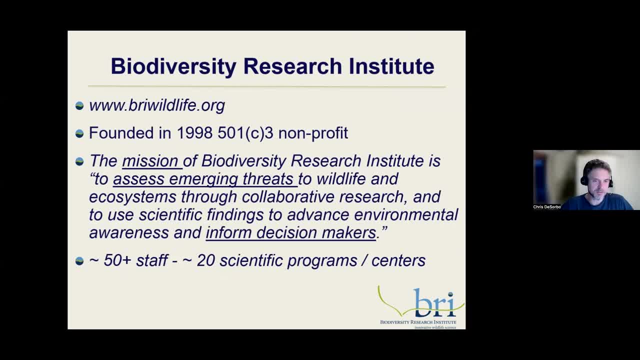 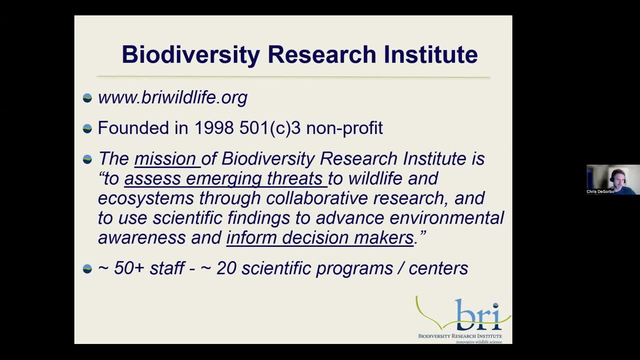 systems through collaborative research and to use scientific findings to advance environmental awareness and inform decision makers. um, and so you know, the focus is really on science, research, uh, policy. we don't really um go into the the world of advocacy like um friends of mirror meeting bay does um, and yeah, our outreach is 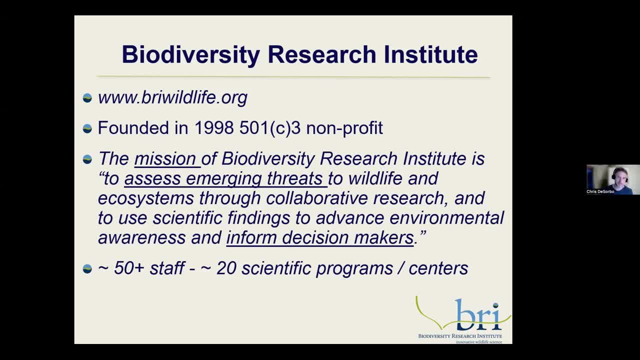 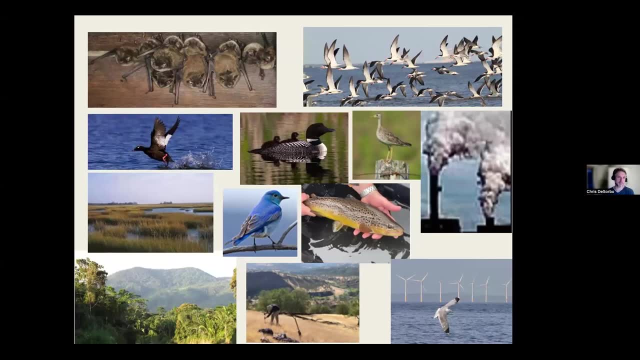 a lot through our website and, you know, just communication pieces. um, we have about 50 staff and about 20 or so scientific programs or centers um ranging across a. it's a pretty wide swath. uh, some of the programs are focused on regions like the tropics or the Arctic. 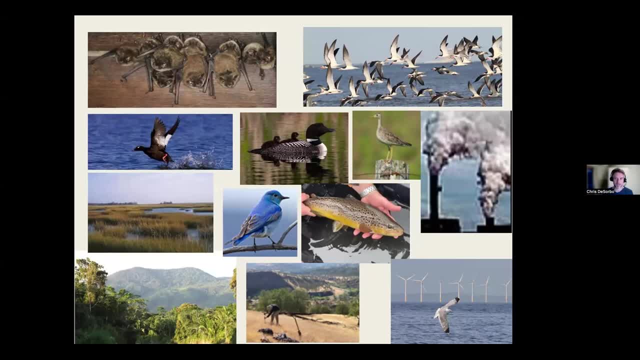 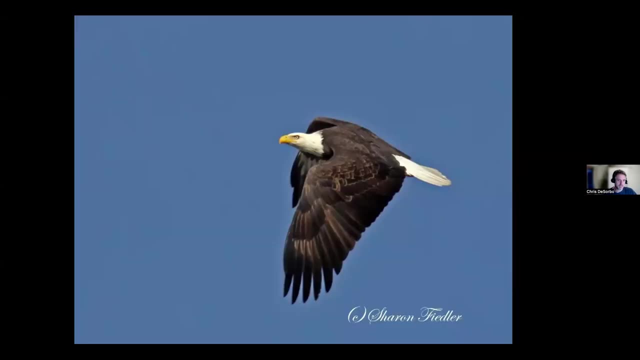 uh, some of them are focused on topics, uh like Mercury change, offshore wind, and some of them are focused on taxa. so things like loons, waterfowl program, mammal program, shorebirds, songbirds, uh, and I focus on Raptors, as Ed mentioned. um, so you know, basically you know of of all the birds in the country. 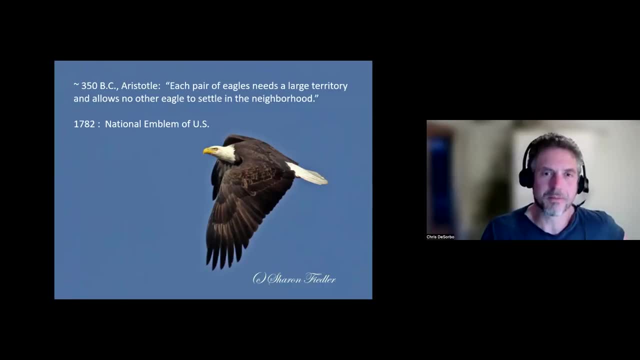 um, eagles have always been noticed. um, you know, it was interesting to me to even find a book from Aristotle about eagles. um, obviously everybody knows, uh, they're the national emblem of the US. um, what some people may not know is that, um, where'd that go there? we go um that. um. 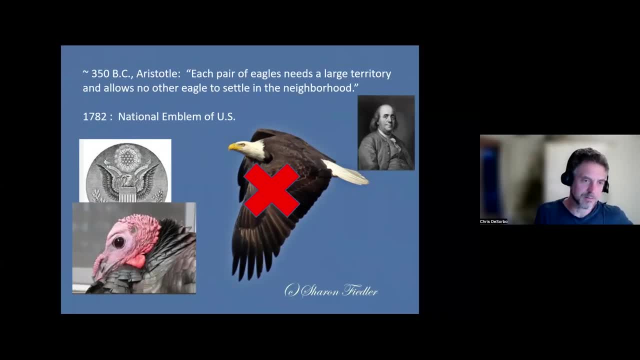 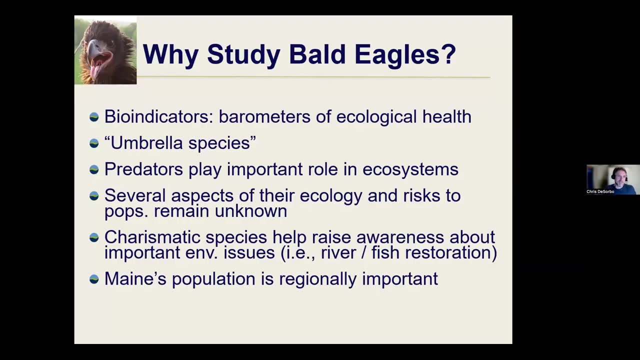 yeah, Ben Franklin actually did not want the eagle to be our national emblem. he was, uh, preferring the, uh, the wild turkey instead. um, and so at this point I always feel like the. the question, um that somebody might pose is: you know, we have sunken so much money. 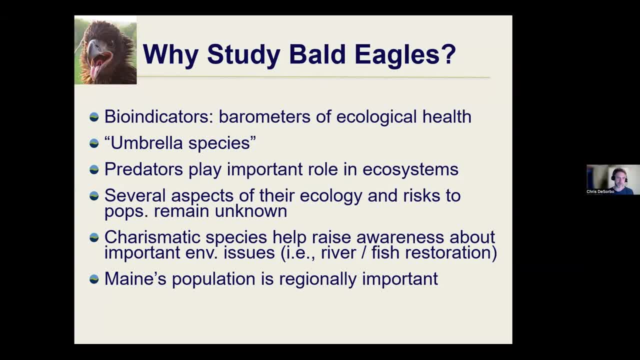 and energy into studying and recovering the species. uh, why, why should we continue to study bald Eagles? and so this is my slide addressing that. um, there are many of them. uh, eagles are great barometers of ecological health. They're the quintessential bioindicator species which many 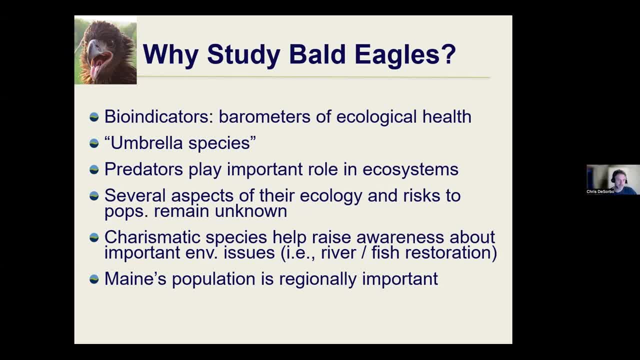 people probably already know about. There's also this concept of umbrella species. So if you do conservation work on a wide-roaming species like eagles, you're protecting a lot of other species that are within that home range. Another factor is just the important role that predators. 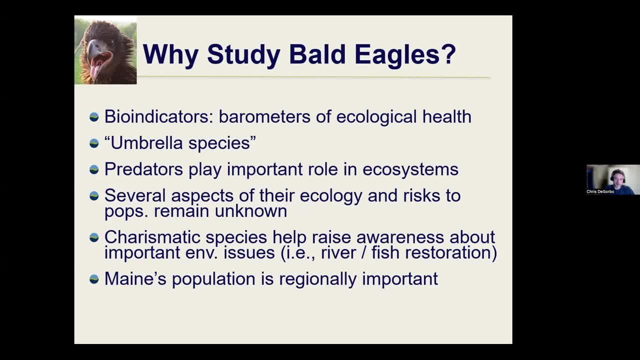 play in ecosystems. If you remove predators from systems, everything gets out of whack, and people can probably think of examples of that. And there are still, despite a tremendous amount of research on the species, a lot of things. we still don't really know about them. 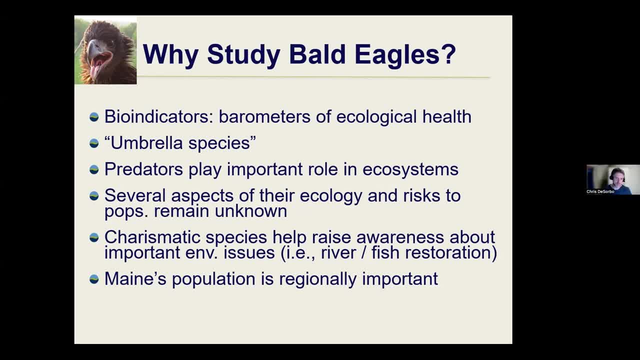 And you know, one thing that I like to do is use the charismatic nature of eagles to protect the environment, And I think that's a really important factor To raise awareness about important environmental issues. So river and fish restoration- People really care about eagles. Some of those people might not care as much about fish, but if it, 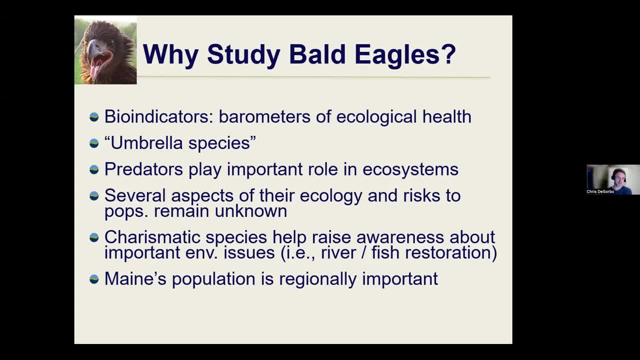 affects eagles, it'll turn some heads And I think that's an important role that you know we can play here And just in the broader scheme of the population. Maine's population, specifically, is regionally important. For example, we have a very large하는데 of eagles in the state of Kentucky and we have this. 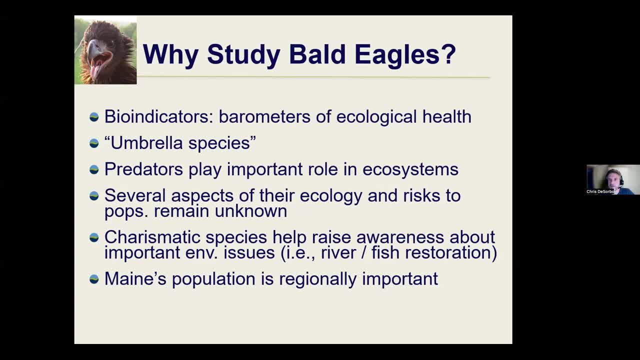 large handler of eagles there, which is a really unique environment, And so we'll have to see how we can adapt to that, And so they may not be there for the rest of their lives, but it's just as important to know how to take care of them, And we're hoping that what we're doing will help. 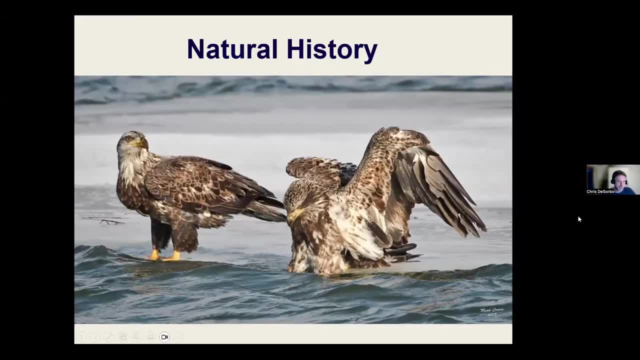 better and better protect them. I'm going to adjust something here. Well, I guess I don't know how to. Okay, So natural history. Sorry guys, I really just need to adjust something that's better. So most people notice that we have a huge lack of natural resources that are close to us. 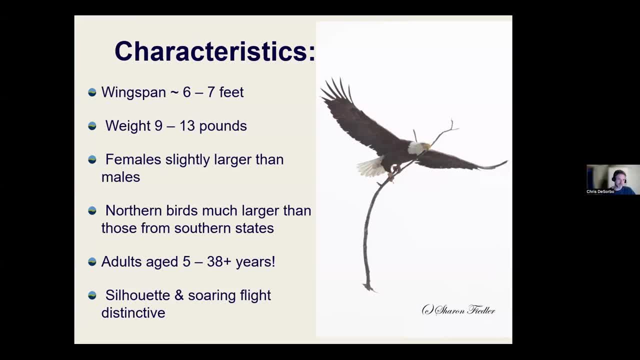 people know the the kind of cookie cutter things about Eagles. uh, six or seven foot wingspan. they're relatively heavy, for nine to 13 pounds. like a lot of the Raptors, females are slightly larger than males. um Northern birds um are tend to be larger than birds from southern states, so you know if we 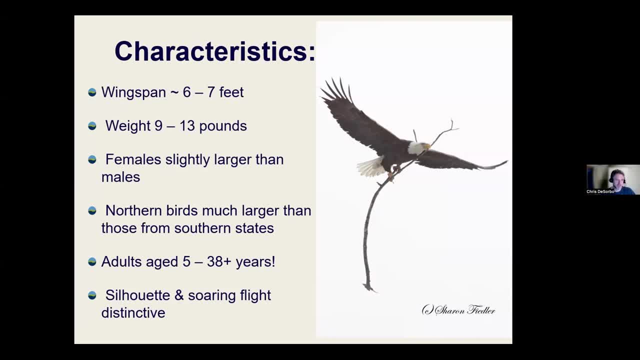 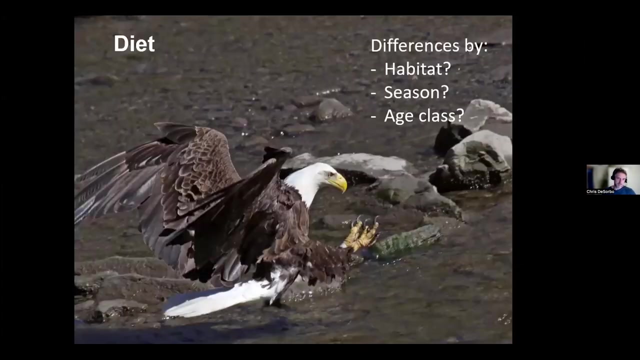 have a Florida Eagle up here. they're noticeably smaller, um than Maine Eagles. uh, they, you know, can be aged, you know, adults, 5 to 38 plus years, um, and a lot of people, you know, compared to a lot of the other Raptors, uh, that you have a relatively distinct silhouette and flight pattern, um. 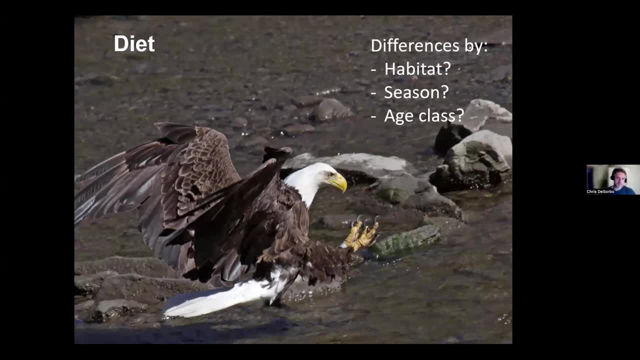 the diet of Eagles. most people have a pretty sense, pretty good sense of what, what the Eagles are eating, um, but one question that I- I think people don't tend to think about is: how do you answer, how would you study some of these questions? uh, you know, we're also interested in differences in diet by habitat or season or age. 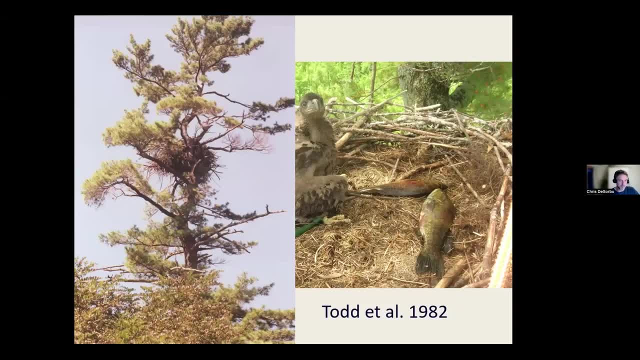 class um. and so back in the 80s, uh, Charlie Todd- who's now um retired um biologist from the Maine Department of Indian fisheries and wildlife, conducted a study just to figure out what Eagles were eating in Maine. and this is, you know, during the, the crux of 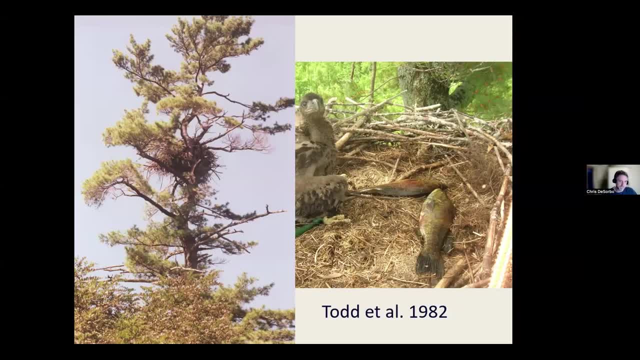 you know the recovery still um, and so the way, one of the ways you can conduct such a study, is to go out and just collect, basically, what's on their dinner plate. so, uh, you can climb a tree, see their nest- um, we did not put these fish here, um. or you can collect- prey remains on the ground. 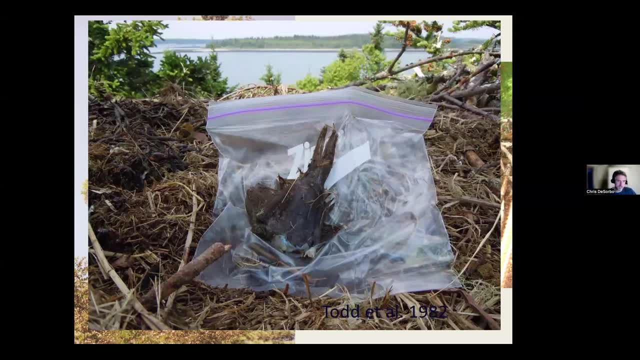 um, and so that's what he did: went out collected prey remains. so if you have two chain pickerel left Jaws, you know there were at least two chain pickerel there, if they're about the same size, um, and then you can start to quantify that information. 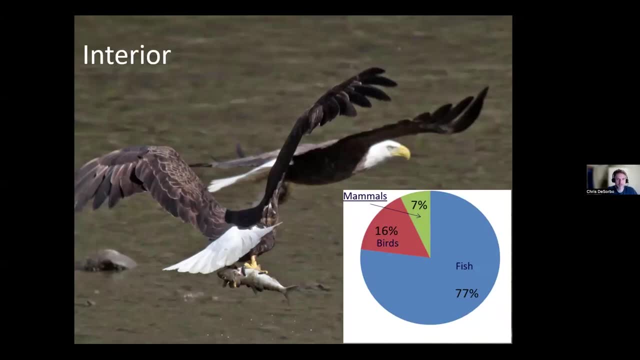 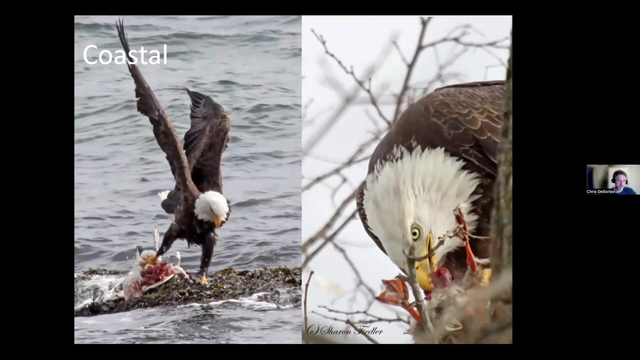 um and so um interior. the findings of that study basically showed: in interior Maine it's three-quarters fish, about 16 percent birds and about seven percent mammals. if you go over to the coast, any seabird biologist will be quick to tell you that they're obviously not just focusing on. 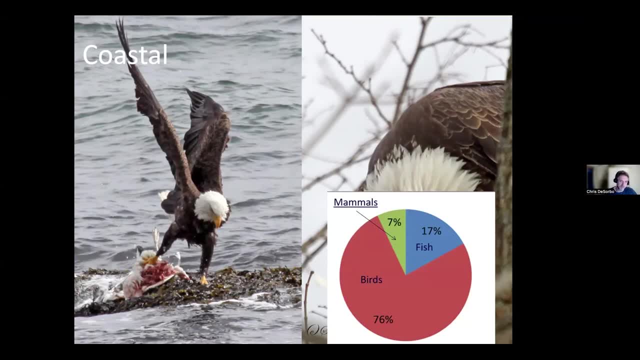 uh fish as much in that environment. there's a real emphasis on seabirds, which has a lot of uh ramifications for things like contaminant exposure, not to mention the seabirds themselves, and so, yeah, you have about a flip here where you know 76 percent of their diet is birds, and then 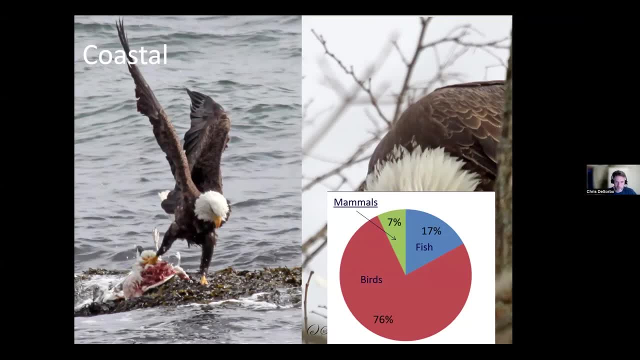 a smaller portion of fish and mammals. I will say that you know there's other groups, we, we have a ton of prey remains that we're still going through with some help from volunteers and you know there's turtles in there, there's um, there's a few other items, but that basically captures it and I guess I will say this is a. 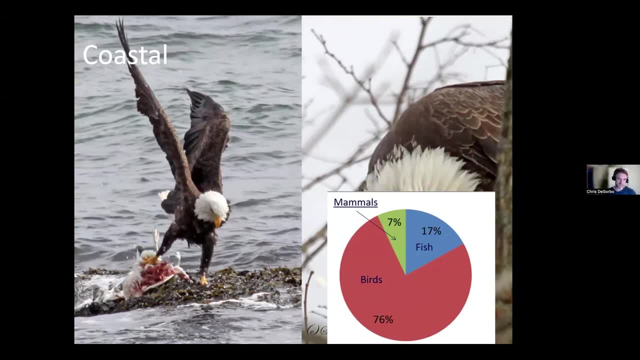 seasonal. um, this is a seasonal representation. in the winter time you have a whole shift to uh, scavenging ungulates, for example, um eagles in interior Maine. as soon as their prey is all locked in with ice, they're going to have to pivot to something else. 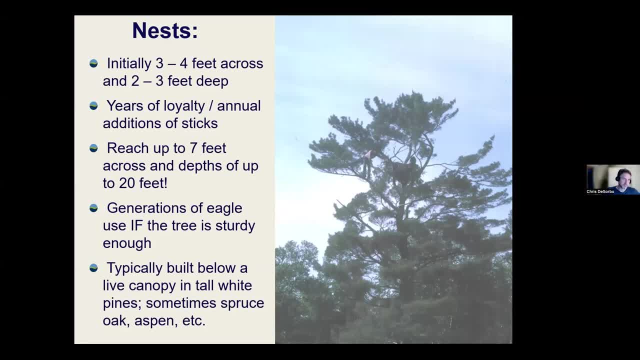 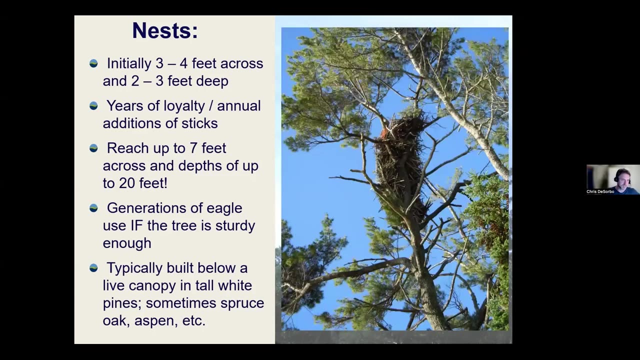 um, nests are giant um, they're three to four feet across, usually two to three feet deep. um, and they will add sticks to those nests for many years. and you know, eventually those piles of sticks will become so massive that they might just take the top of the tree down, or 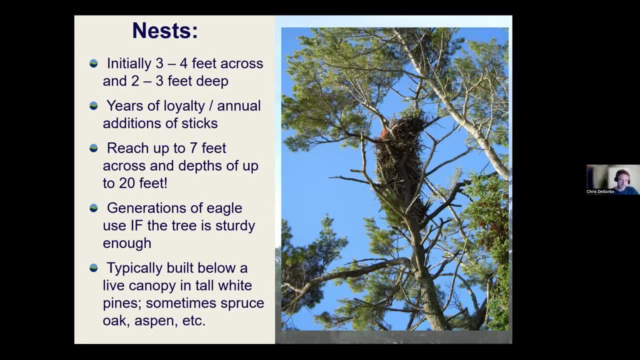 just fall out um, and you can actually see these layers of different years of material on these um Eagle nests. unlike ospreys, who tend to nest at the very tippy top of trees, Eagles like to build their nest below the canopy, usually kind of more in the crotch of the tree. 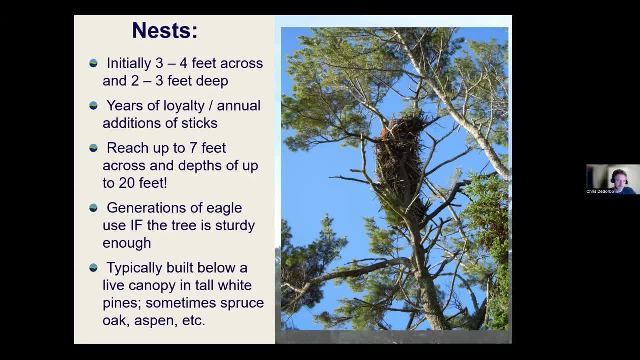 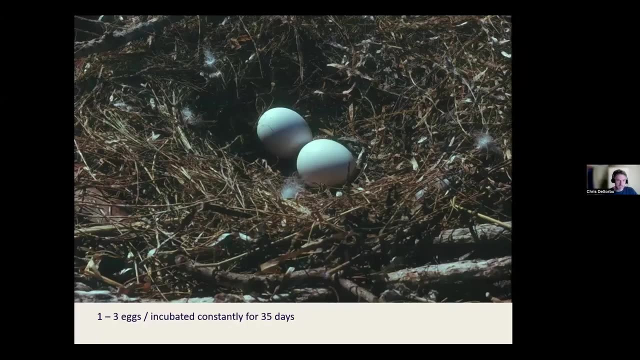 typically white pines are the preferred nest tree of choice, but on the coast is just a lot of birds and spruce trees. uh, in some of the river corridors, like the Penobscot, they're in Oaks and popples and things like that. um, and of course, the- uh, the thing that I found surprising the first time I got into up to an. 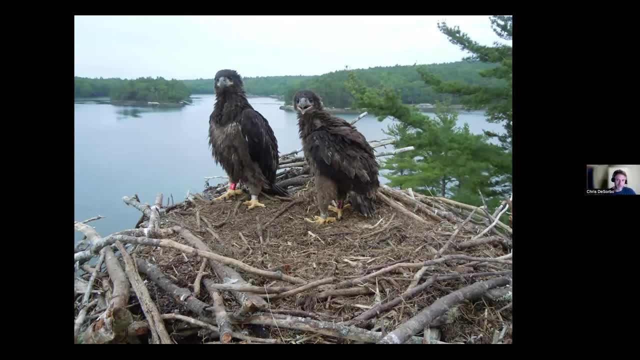 Eagle nest was just how flat it was. you tend to think from the ground that this is a a big, giant bowl and the birds are sitting down in it. it's not really the case. it's pretty flat up there and they just tend to line sticks around the outside and then softer nesting material in the 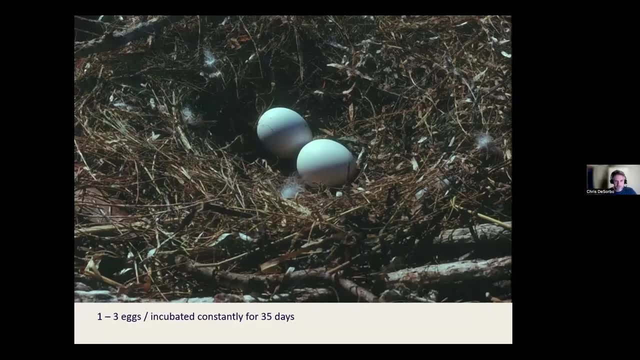 middle. one to three eggs is typical. so two is the typical. um much smaller um. did you think two was the typical? um much smaller bays in general versus more common eggs in general. What do you think of this at the beginning of January? the pretty suggestive timing because I did like the bird- Can we move on? we're getting on to the next question. 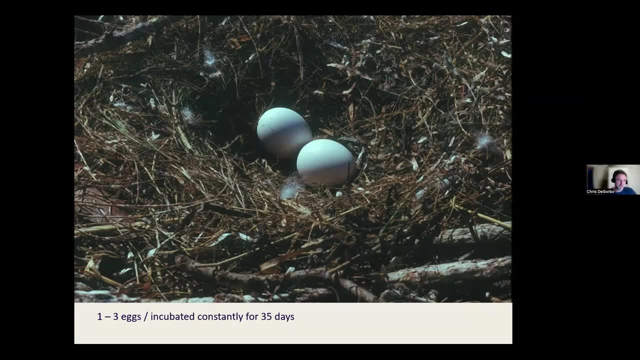 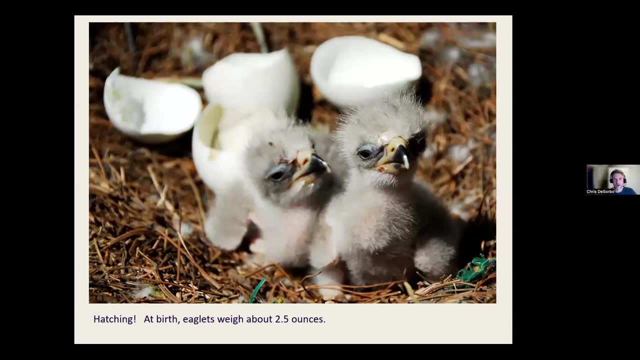 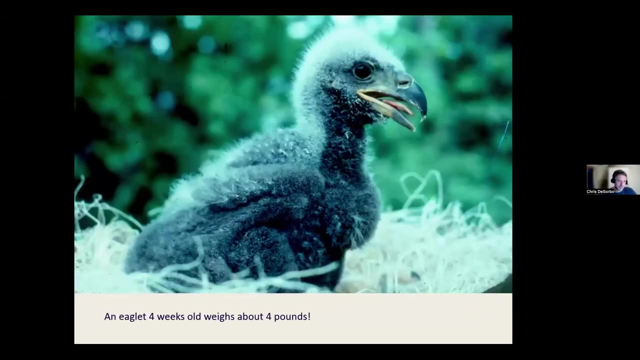 I did like the bird. Can we move on? we're getting on to the next question. smaller proportion are three-egg clutches and one-egg clutches incubated for about 35 days. The chicks are the first coat of feathers. are these little white downy feathers which eventually 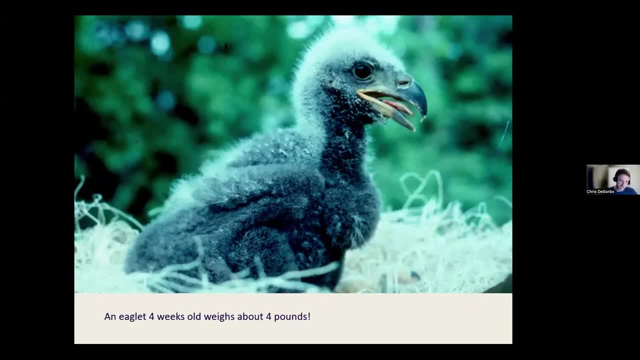 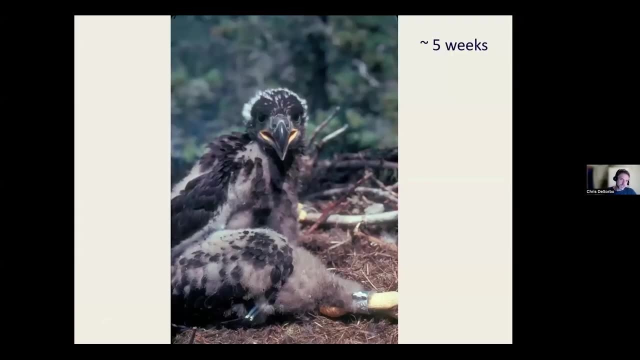 kind of turn into this little Don King haircut and these gray feathers come in and then, about just after four weeks, these chocolate brown feathers start coming in. You can see in the in the lower part of that slide. there, if people aren't familiar, there's some feathers and sheath. 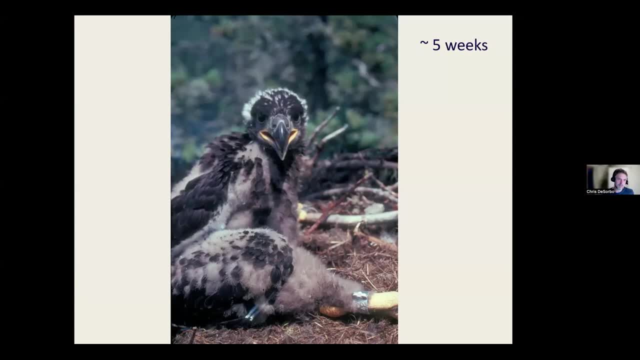 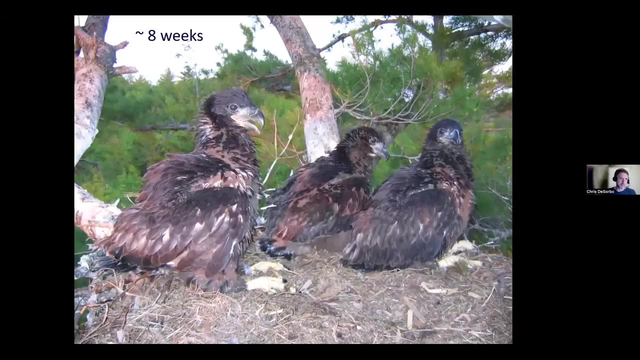 they look like they're. it's a little waxy coating and the feathers are. there's blood going to that feather and the feathers growing and that's what that little waxy sheath is About eight weeks or so they're largely covered in these kind of chocolate brown feathers and then full grown at about nine or ten weeks. but they 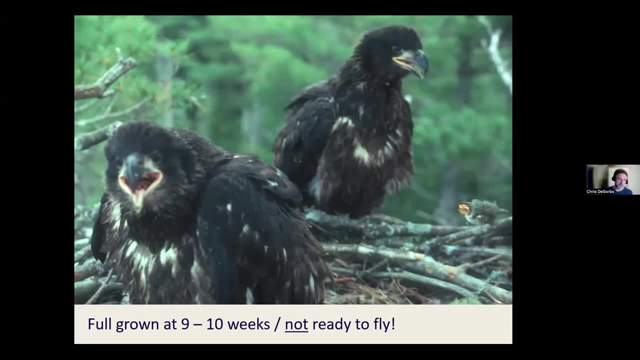 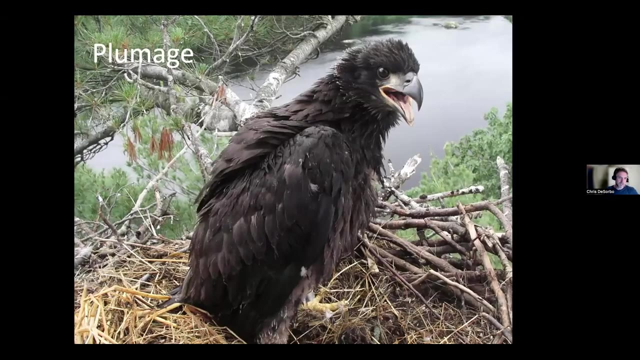 still can't fly And in fact, even after they fledge at, say, 12 or 13 weeks, their feathers are not fully grown on their wings. So it's a really interesting strategy. So how do you get from this? you know, chocolate brown standard bald eagle nestling to this? uh, i feel like maine is. 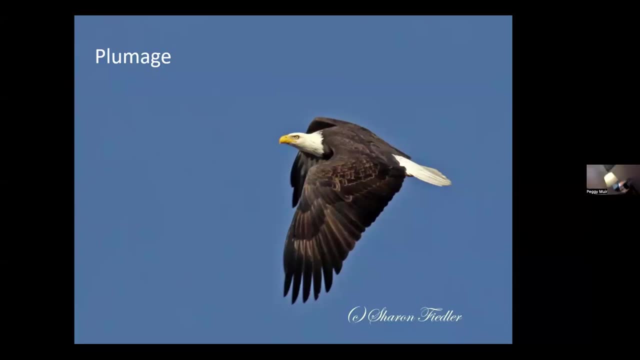 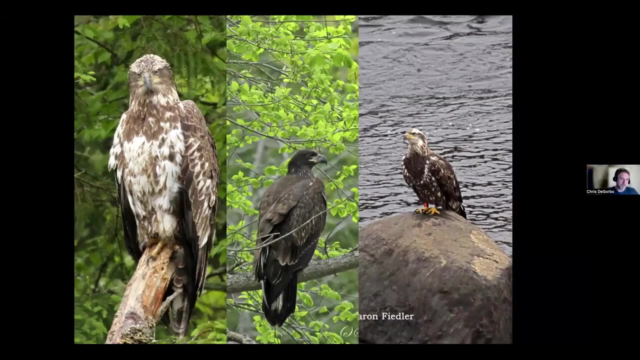 interesting in that probably the no doubt the cornerstone study on this was conducted in maine by mark mccullough. so you have all these other plumage variants right, and so at some point, um, we're all wondering: hey, how, how do you, you know, how can we figure this out? 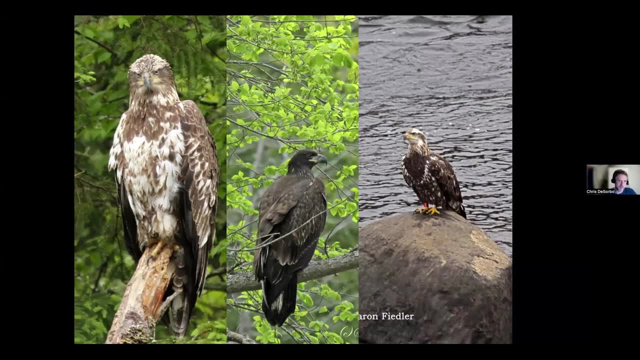 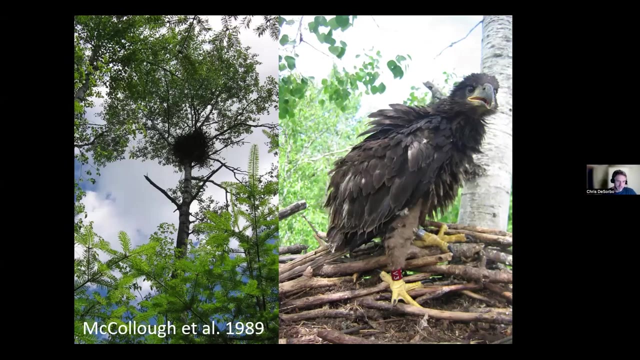 so mark, who is a retired us official wildlife service biologist, focused on eagles um, sought to figure this out, and so if you think about how one might achieve such a thing, similar kind of story: climbed a bunch of trees, banded a bunch of nestlings with field. 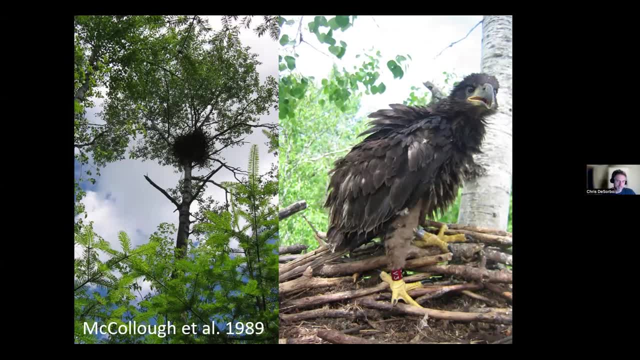 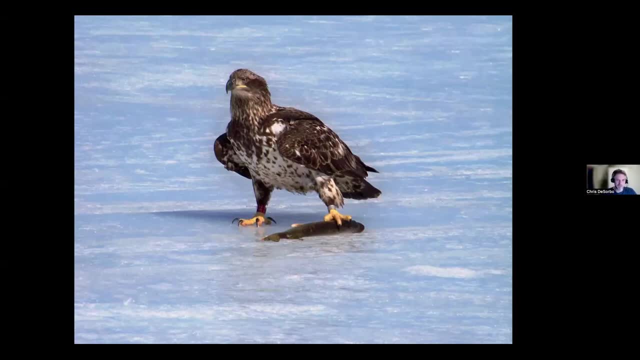 readable codes. and then, um, guess what? he sat and waited the ice in the winter time for multiple years. uh, this is a picture of a banded eagle out on the ice. um, with a, you know, with a fish, but in mark's study they just put piles of. 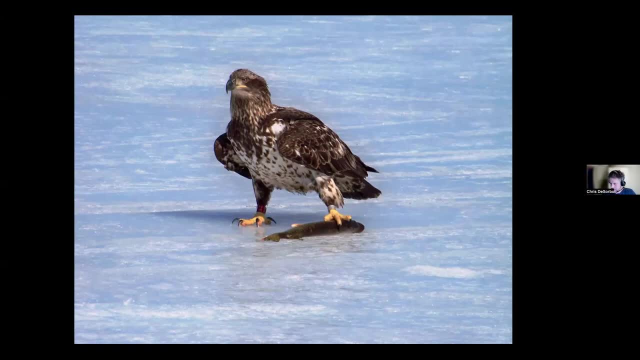 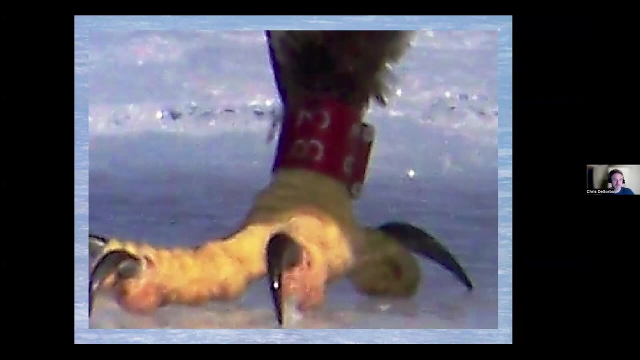 uh prey out there and just froze them into the ice, and so you know many uh winters spent in a blind. eventually, you get a look at the band. you say, okay, i know who that is. that's b3. you can identify that bird. and then it's also an artist. 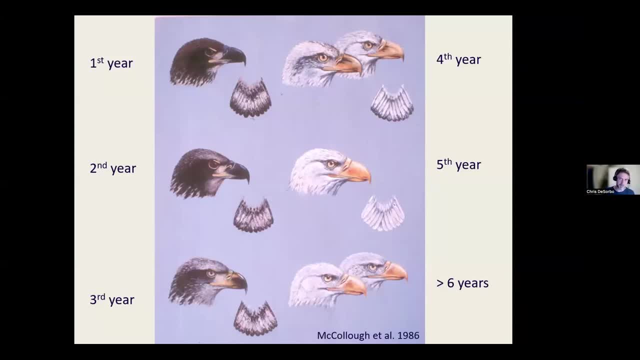 so this is basically what came out of that, and it previously was not known before. so you don't have to get too stuck in the details of this. but uh, the key is that in the first three years um really plumage- is the most wszystkich под driven sex worldwide- okay, um, and then um. 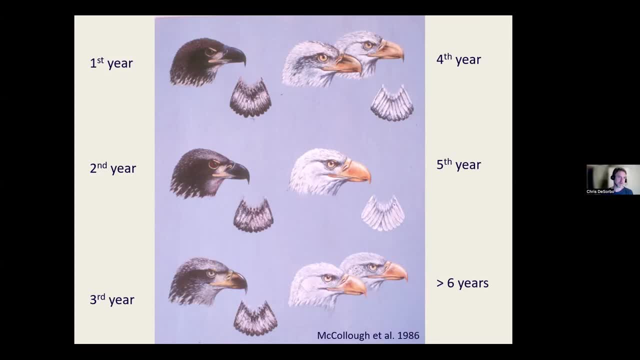 Plumage is not a terribly useful way to age them, as most people think it is. The more useful indicators are the bill color and you see the eye changes color over time And so the base of the bill basically goes from black to yellow. to this the third year. is this sort of bruised banana look? 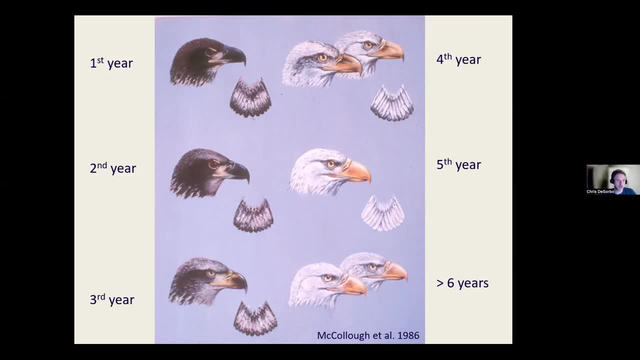 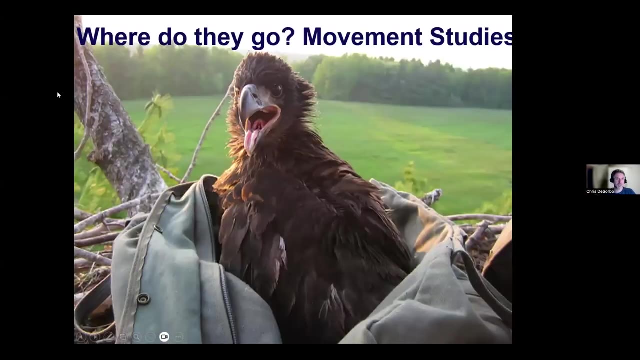 And then you know, from the fourth, fifth year out you get the whitehead- Breeding typically starts around five years- And other things you can do with banded birds, which we've done a lot of in Maine, which Ed mentioned. 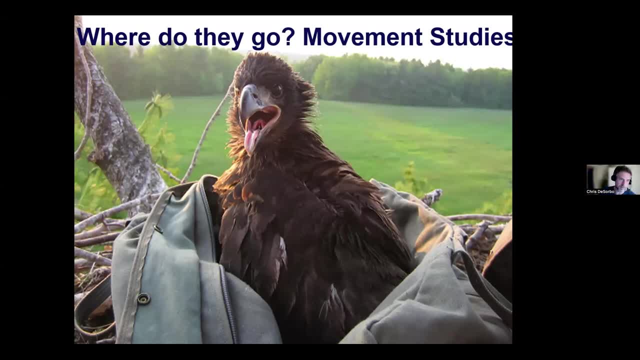 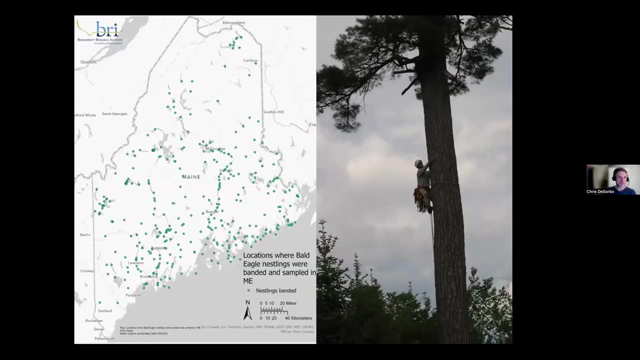 is. you can just really start to understand where birds live, Where birds go, where you know once they fledge from the nest where do they end up going, And that has a lot of management and conservation implications. So this is a map we actually just very recently finished that shows where we banded eagles. 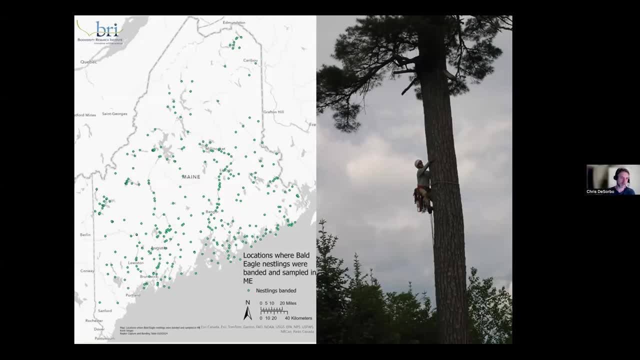 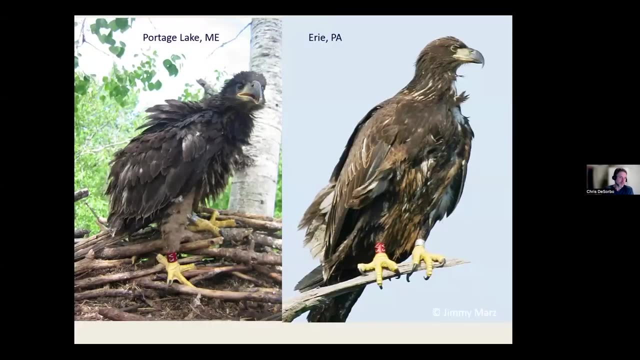 This is over a, you know, roughly 20-year period throughout Maine, And what you end up with is, you know, a marked bird like this one on the left at Portage Lake up in northern Maine, And then, just a few months later, a photographer takes, you know, a whole series of amazing photos of this bird. 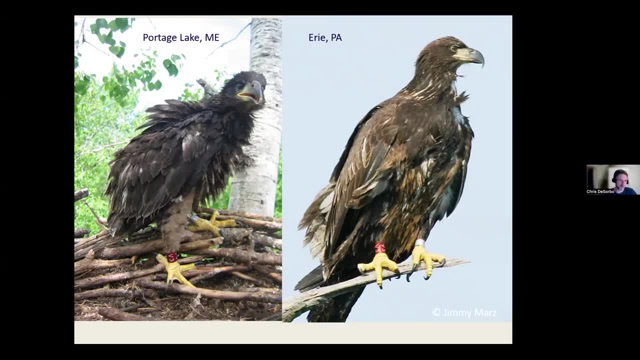 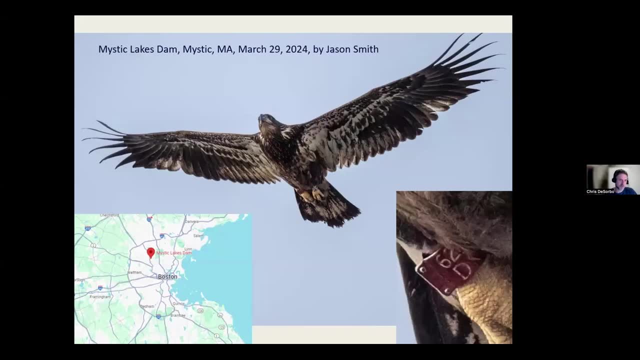 So now we have one piece of information about their movements. This one actually just came in on March 29th And it's relevant to you guys because this- so this bird, was seen at the Mystic Lakes Dam in Mystic Mass And you can read that 62D on the band. 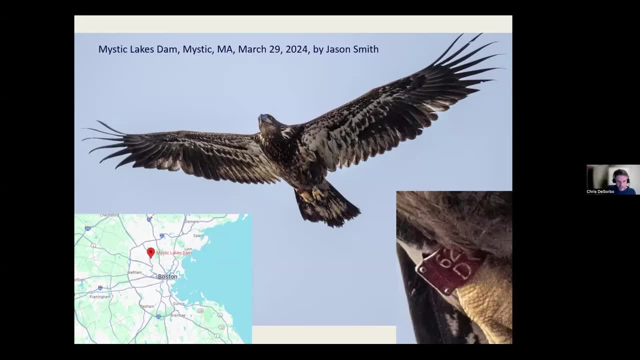 There's also- I didn't mention there's- a silver band that we put on the birds as well, So you can see the one next to it. It's a USGS band that basically has a social security number for the bird, So if it dies, we can. 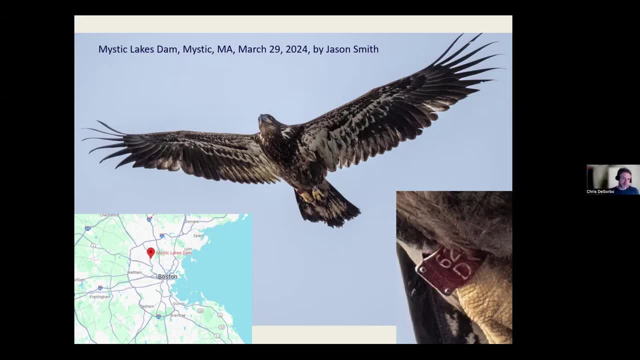 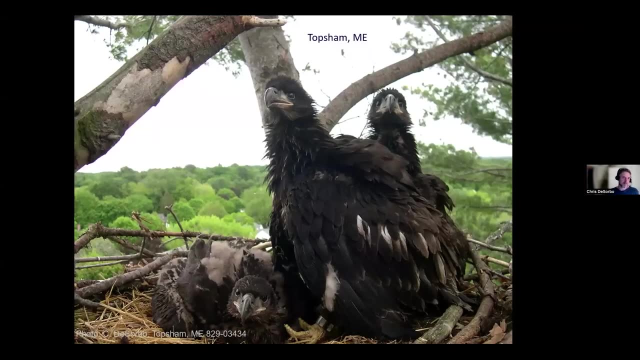 Get a look at that band, And so that 62B bird ended up, was it B or D? 62D ended up being the topsum nest that we visited just this year, And so, as I looked through the photos, I was trying to figure out which one it was. 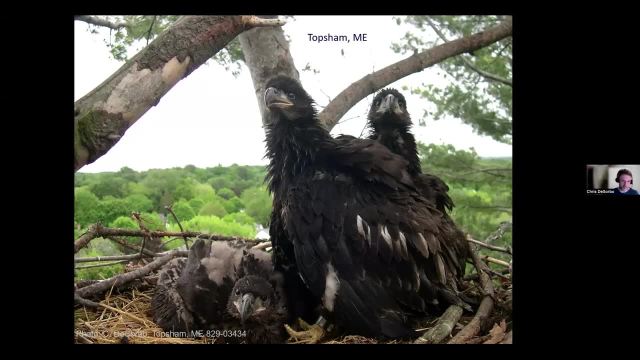 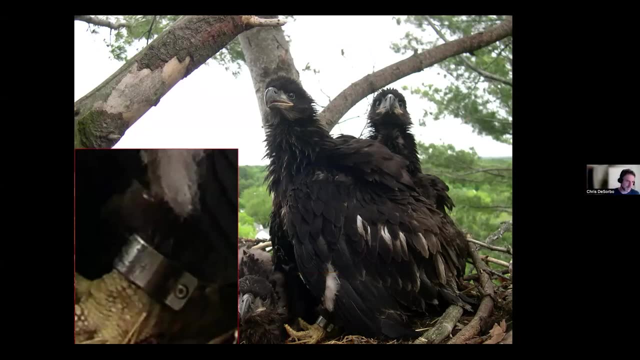 And I was like, ah, Jesus, too bad, I don't have a photo with the band showing, which is unfortunate, But it was pretty great. And it turns out that silver band you can read the last two digits And that lines up with 62D. 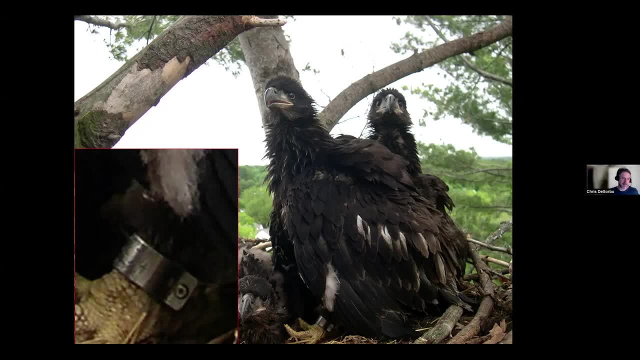 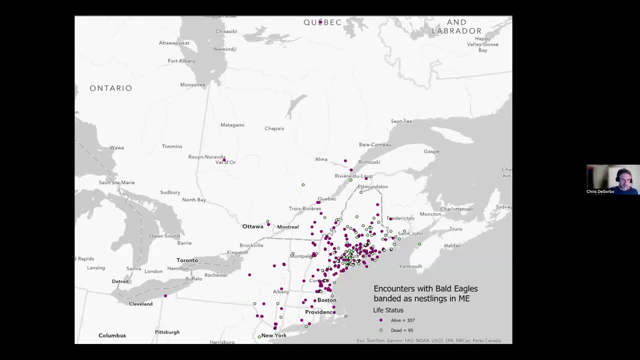 So there it is is the biggest chick in that nest and topsum by the retirement community. And if you pile all those up onto a map, we call them encounters. You get some encounters of live birds, some encounters of dead birds. This is basically what you get. 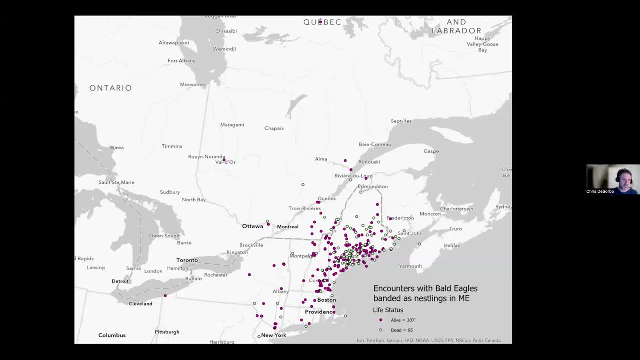 So you have a distribution throughout all the New England states. There's a dot way up at the top here in Quebec. Some of them have been detected over in New Brunswick, Nova Scotia, down in New York, et cetera. Far more encounters with live birds than dead birds. 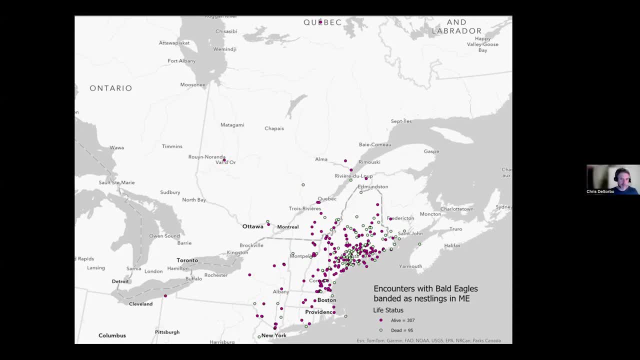 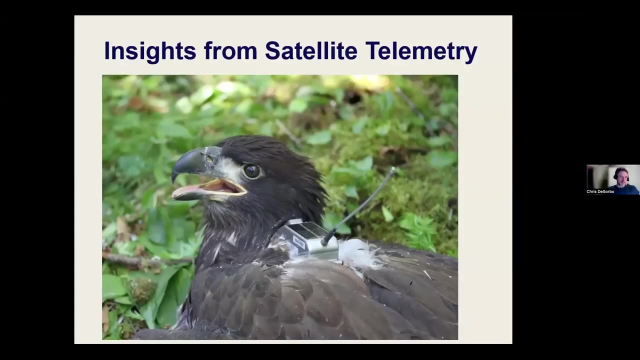 But of course, this is a function of where people are and the fact that people have amazing digital photography today, And so we get so many of these that I have a very hard time keeping up with them. actually, Another way you can look at movement patterns of any animal at this point is to use tracking devices. 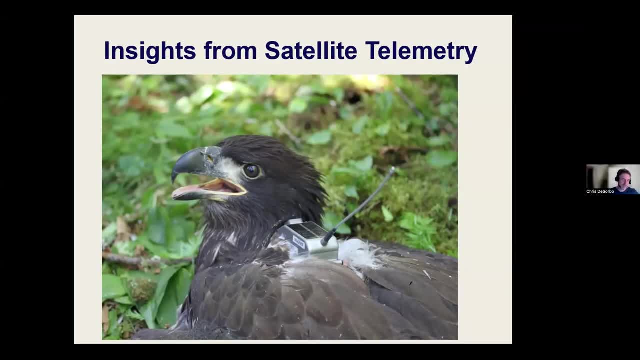 And one of those types of tracking devices is satellite telemetry. So transmitters that are fitted to bird are relaying location information up to satellites, which then send it to the bird And then send it down to a server that I can access and find the location of that individual. 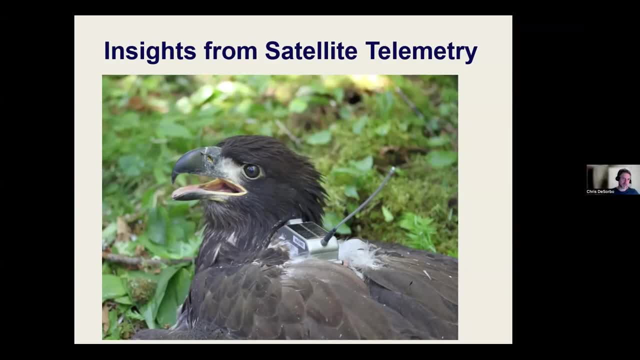 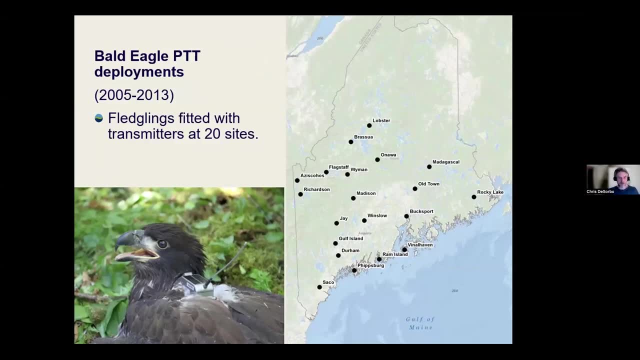 Nowadays there's all kinds of other technologies using cellular networks and all kinds of other things, But we were specifically interested in trying to address this. you know what I thought of as like the black hole of the ecology of eagles in Maine and a lot of places. 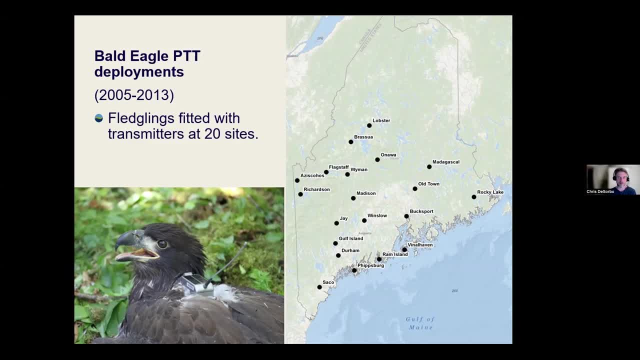 After they fledge it's pretty hard to really know, know anything about them, and all of those band encounters we got are starting to tell the story. but there's still a lot we don't know about seasonality: uh, how far do they go? there's those. 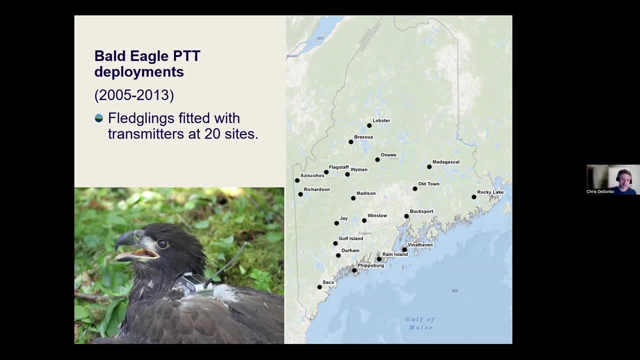 those are two points on a map. there's so many questions that were still unanswered and again, these have a lot of conservation and management applications. so from about 2005 to 2013, we climbed trees at all of these locations and fitted a single fledgling with uh satellite. 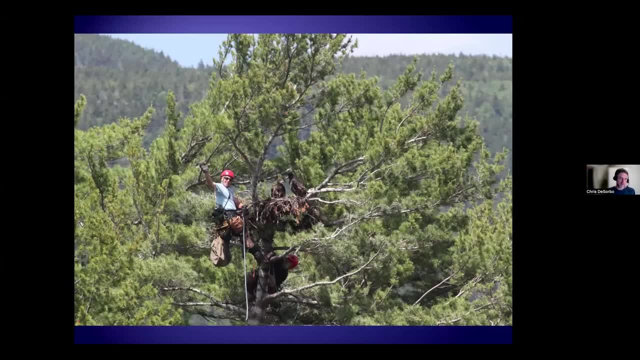 transmitters and the way we do. sometimes we do that a little differently. we might get an age on birds beforehand. uh, in a few cases we would actually send two bird, two climbers up. uh, this is bill hansen, who's worked for power company and for us for a bunch of years. 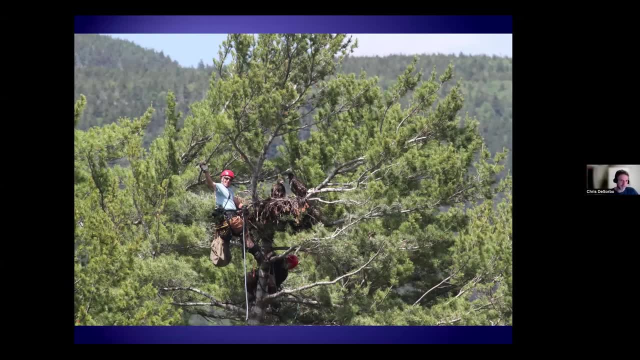 years and also just retired, And in some cases it's just really helpful to have two climbers because you can have one person go out the back and make sure that the bigger chicks don't fall out. It actually very rarely has happened that a bird falls out or jumps out, But if you're going 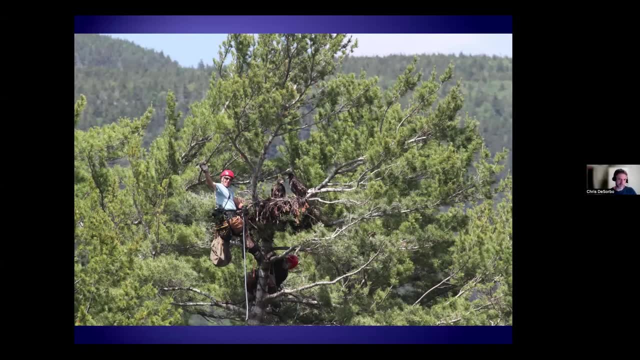 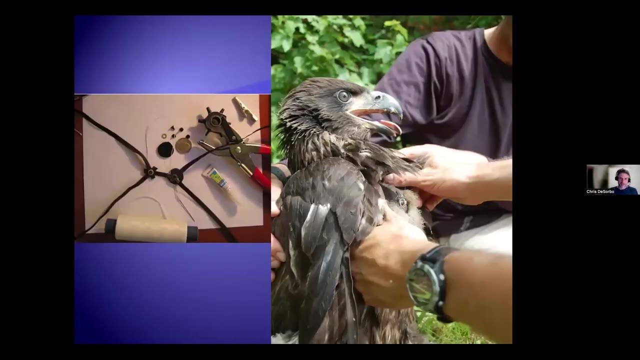 to be putting tags on these larger fledglings. we want them at, like you know, eight and a half to nine weeks of age, as opposed to like six. when we're doing nestling, banding work and sampling work, There's just a much higher possibility that they come out. So once we bring them down to the 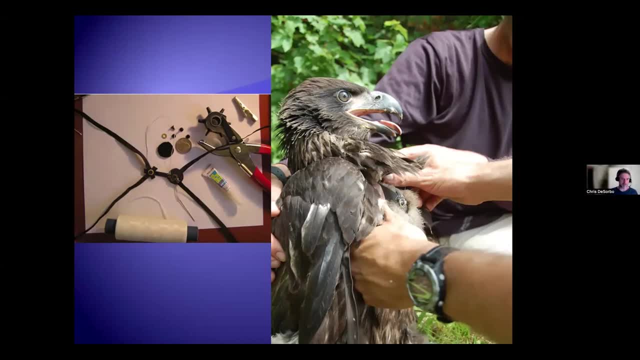 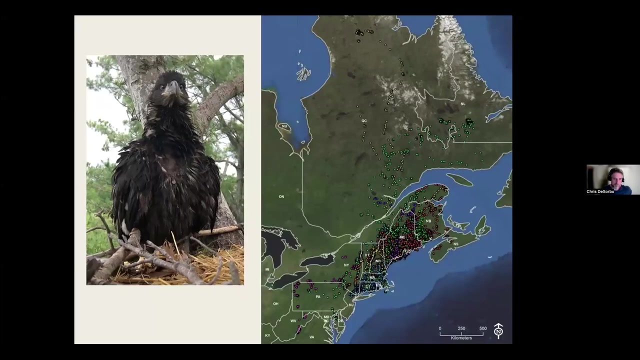 ground. we would fit them with, essentially, a backpack harness. The tools on the left are how we used to do things. Now we just sew it on, But it's essentially wearing a backpack, just like you would, between the shoulder, The shoulder blades essentially behind the head, And so, if you remember the map of the encounters, 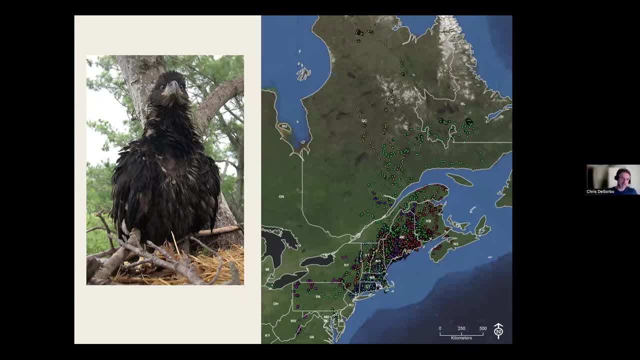 as a comparison, this is kind of the scale of what you might get from satellite telemetry of those 20 individuals, And this is still actually with technology that isn't nearly, as you know, high resolution as some of the newer technologies. So this is probably something like 100,000 points as opposed to. I think it was over, you know, 400. 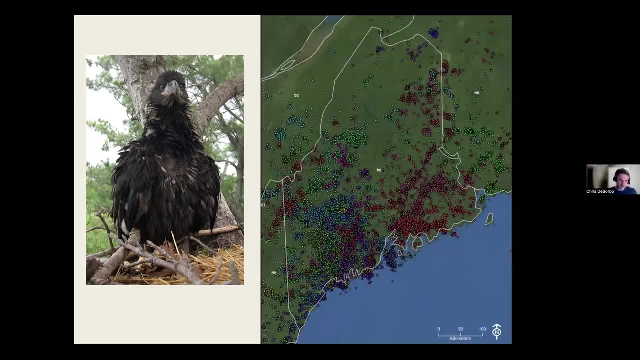 encounters with bald eagle nestlings. So as you start zooming in, each color that you see here is a different individual And you can start to see- yeah, there's clearly patterns to you know, to some of the areas that birds are spending time. 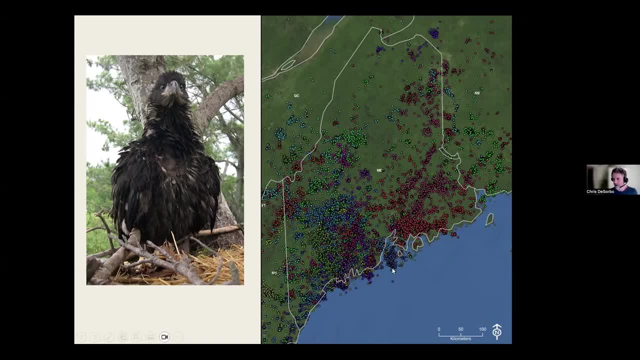 You could notice this. you know this area right around central Maine. there's a ton of birds that are visiting that area. So we were interested in really just starting to characterize what birds are doing during their subadult years. And so are there seasonal differences. What about differences between their first year, their second year, their third year? 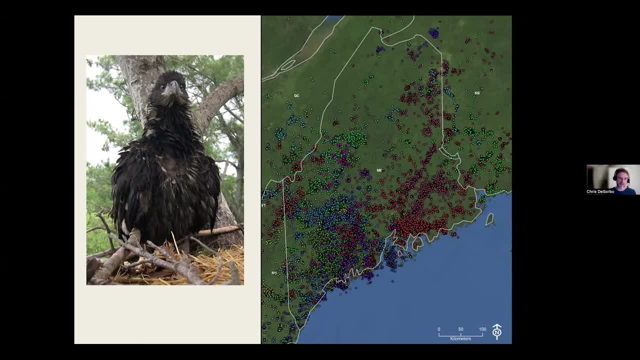 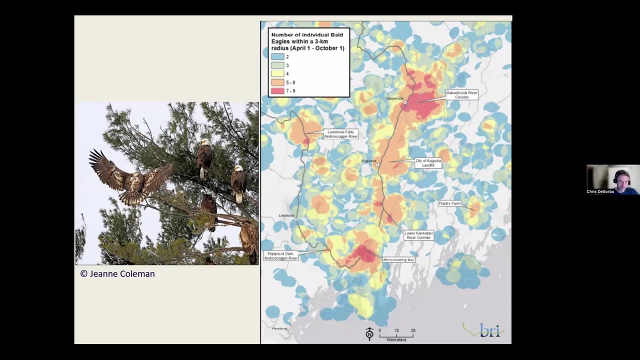 Is there a shift over time. Eventually we know that they come back relatively close to their natal area and settle in, but that might be four, five, six years. So if you picture laying a grid over the last map, this is a really probably the most crude approach we took. 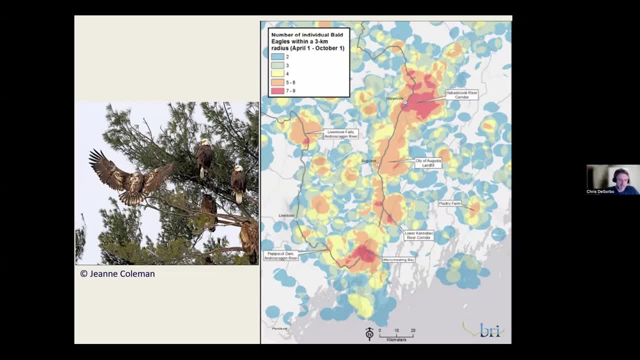 But the first one to just take a look at where what we can learn about areas of importance to Maine's subadult bald eagle population, And that I think is really important Because basically a sec here, okay, just checking my time. 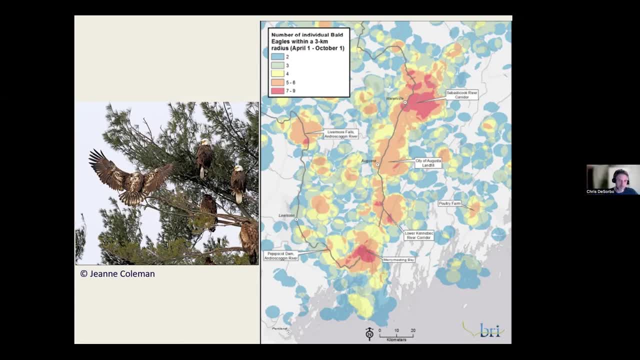 So it's important because it plays a huge role in population stability. So if we can find out areas that are important to eagles, then we can start targeting conservation efforts or management efforts on those areas. So this is basically a heat map that shows. 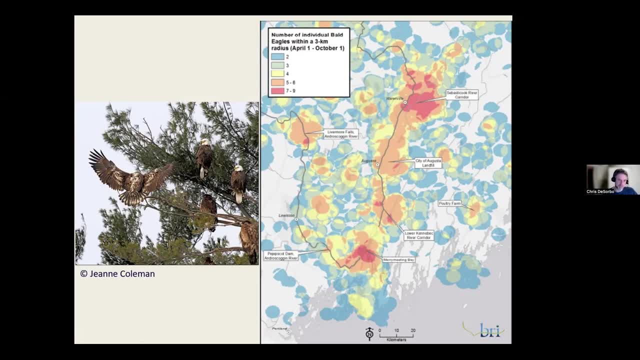 hotter areas are essentially the areas that are most important to eagles. So this is actually pixel, basically squares where more individuals have coincided over time, And then the colder temperatures on the map, so to speak, are where fewer birds have. So what pops out is kind of interesting. 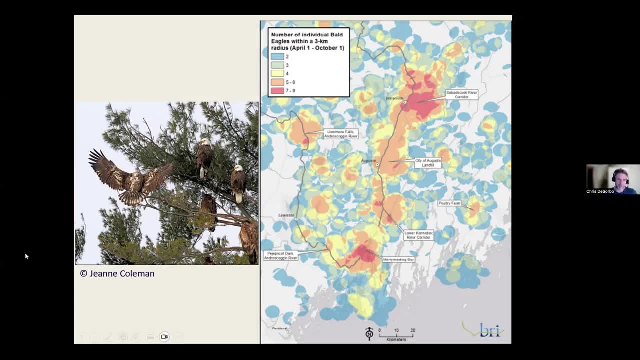 You see, some areas that we know to be important. Marrimeeting Bay is in there, And so you know, somewhere between seven and nine eagles of that, 20 all happen to go there, And same with the Sebastakook River. 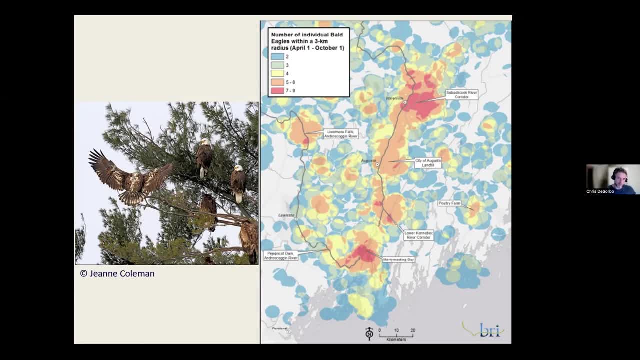 the lower Sebastakook River. We've done a fair amount of work there. It's one of the biggest fish runs for river herring. So that's, you know, a further justification for, you know, targeting conservation efforts in that area. 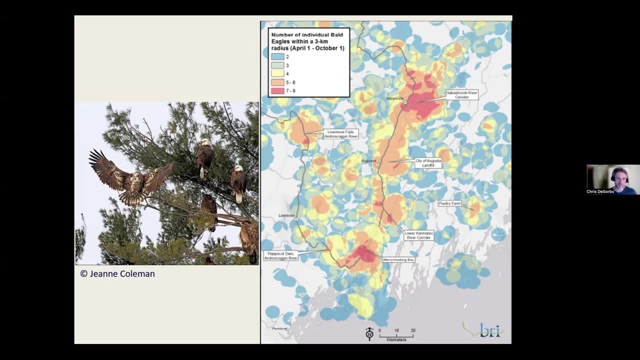 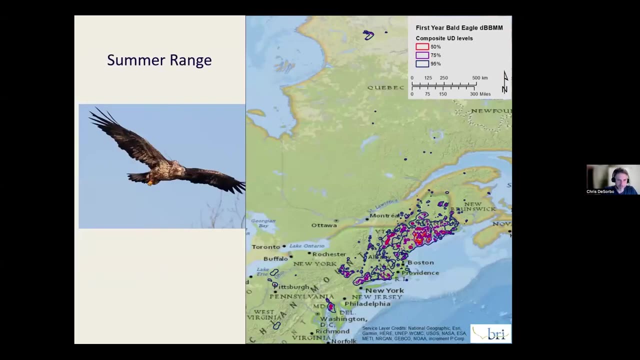 Then you also have some surprises to some of us, like the City of Augusta landfill. You see a few dams, We're open water And fish probably pile up. But basically that is a pretty crude way to do it And if you really want to start, 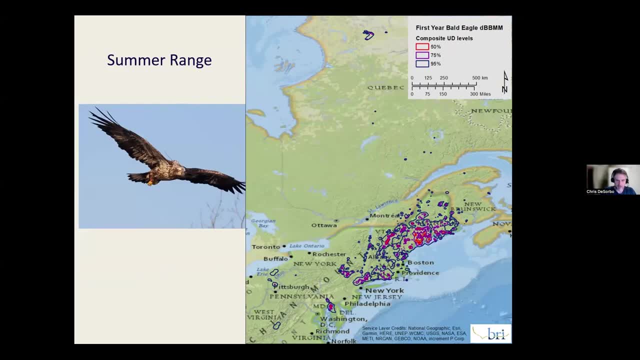 getting a better sense of what the movement patterns of these birds are, we now use what people call movement models, And so this map is basically a composite of all the individuals averaged together from fledging to early winter, And these are their first few months of their lives post-fledging. 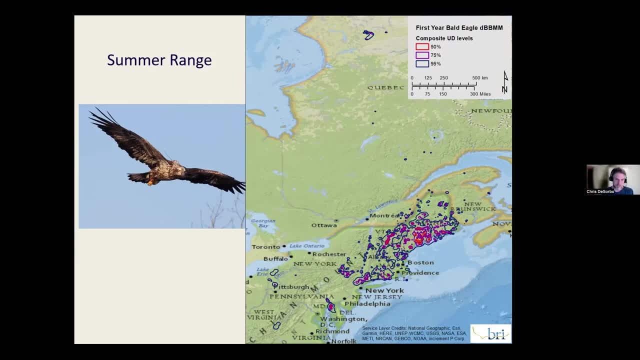 So the red areas are areas they really spend a lot more time. to put it really simply, The blue lines around that is just capturing 95% of the use, And so now we have a fairly decent idea of what Maine Eagles use patterns look like. 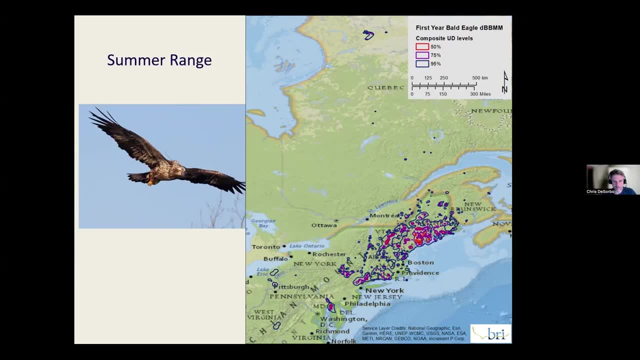 You can see the Connecticut River corridor pretty clearly delineated there between Vermont and New Hampshire, And then of course you know the whole central Maine area overlapping with the Kennebec River. There's just a lot of things going on in there. 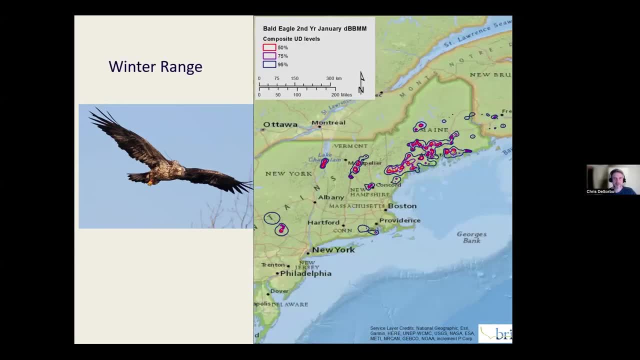 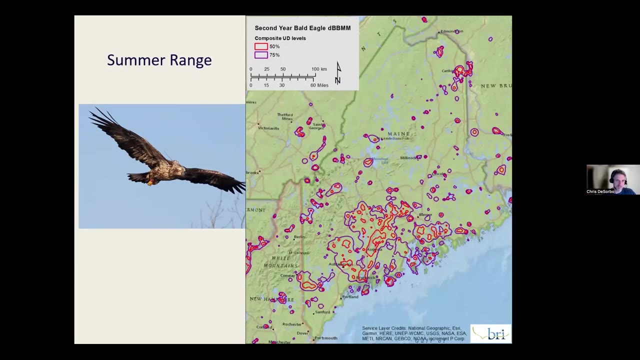 If you picture that last one, it shows what birds are doing during the winter months. So you see this huge contraction of their range. They're really just keying in on a few areas during the wintertime, for obvious reasons. This is just kind of zooming in on that in the summertime. 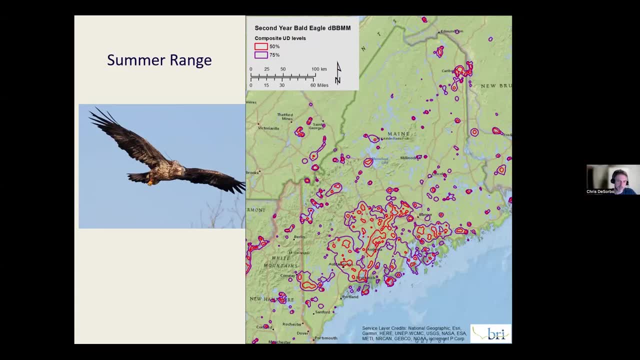 So here you go, You can see. you know the red areas are really the areas they're spending the most time. And you have. you know, we didn't tag birds this far north, up here, up in Caribou, But in the summertime 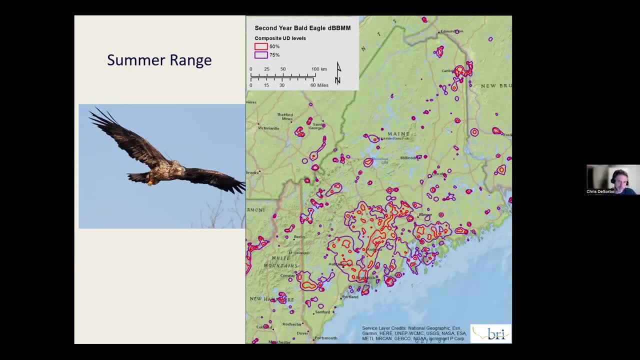 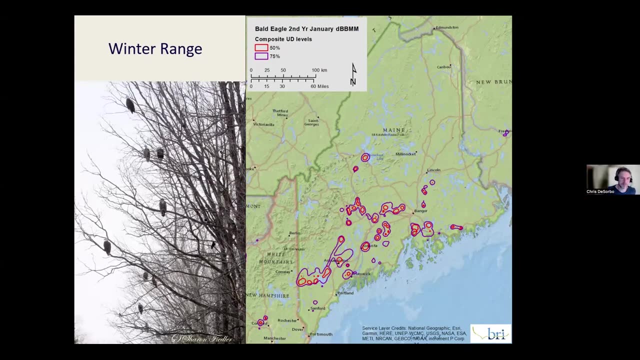 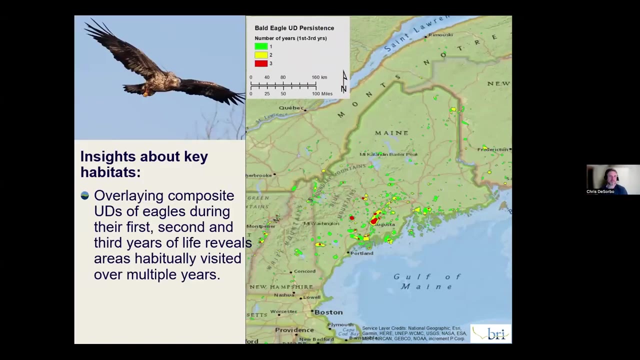 there's all kinds of use patterns that start to pop out Winter range again in Maine, just really refined down to a few key areas. And then this is an approach that we took, that you don't have to worry too much about the details. 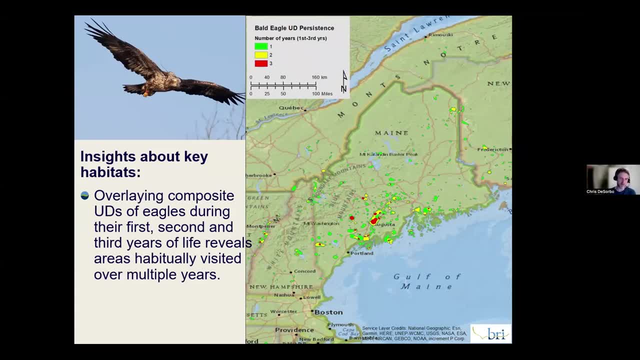 But essentially, if you overlay the use patterns of birds in their first year with birds during their second year and then birds during their third year of life, it reveals areas that are habitually visited over time. So if they're visiting these areas habitually, 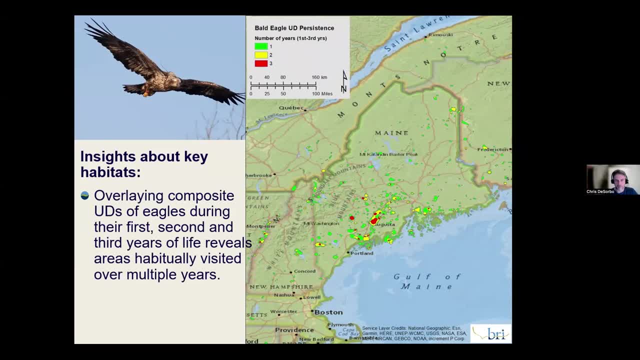 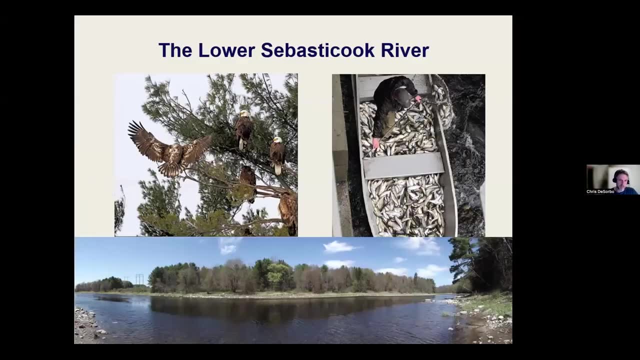 it's not a coincidence, right. There's important food roosting resources in those areas, And that's where we then focus our efforts, And so one of those areas that popped up, and I mentioned before, is the Lower Sebastakook River. 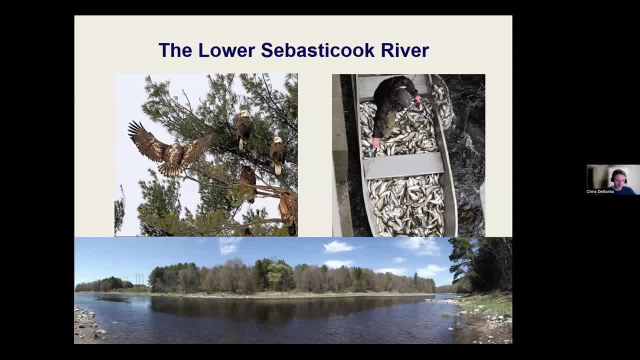 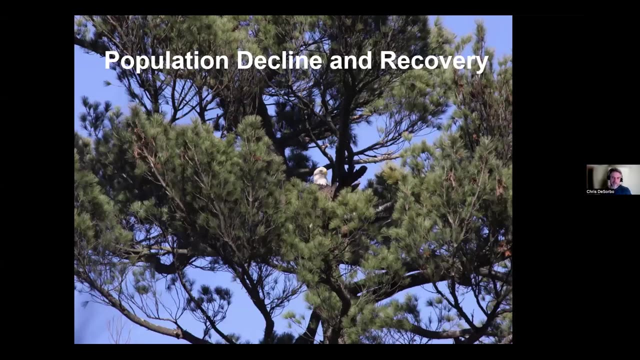 This is probably one of the more important areas to sub-adult eagles in the state We've had. you know roughly half of the eagles that we tagged just in that 20, that group of 20 basically found that spot. 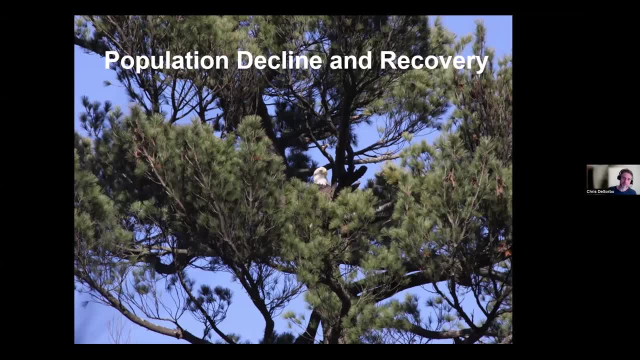 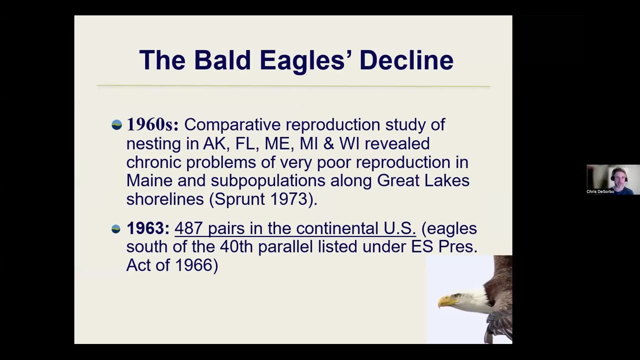 And so those areas are important when you have stresses on the population. So this is this is a pivot to talking about the decline and recovery for a little bit. So back in the 60s there was a study of looking at comparative reproduction. 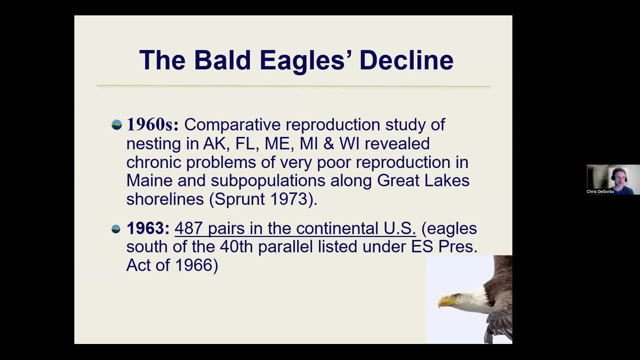 in bald eagle populations in a few key areas- Alaska, Florida, Maine, Michigan and Wisconsin- And so that revealed what people had already been noticing is that there's something going on with eagles. There's chronic problems, There's a lot of 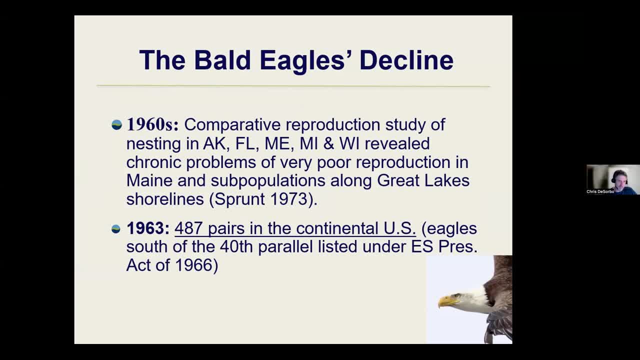 with their reproduction, especially in Maine and subpopulations along the Great Lakes. So in 1963, a broad survey was conducted in the whole continental US. Only 487 pairs of eagles were found during that survey. So what are the reasons for that? 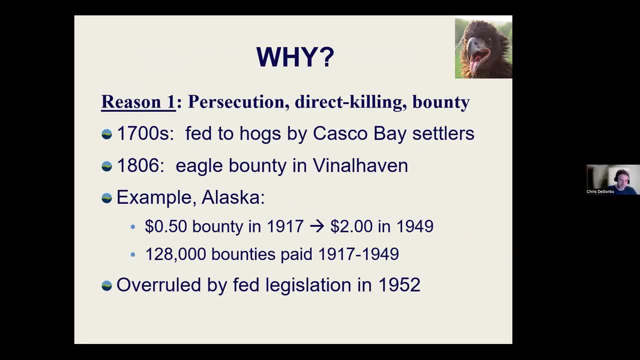 But one of the biggest reasons was just persecution. Eagles were killed. There were bounties on eagles In Maine. they were fed to fed to hogs. There's, you know, a bounty in Vinyl Haven in 1806.. 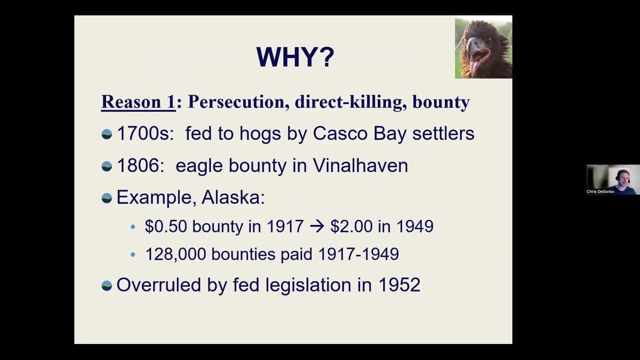 You can see these different numbers of how much you could get, or the, the claws were, the feet were really, I think, the desired item from the bounty, And so about 128,000 bounties were paid, paid out between 1917 and 1949. 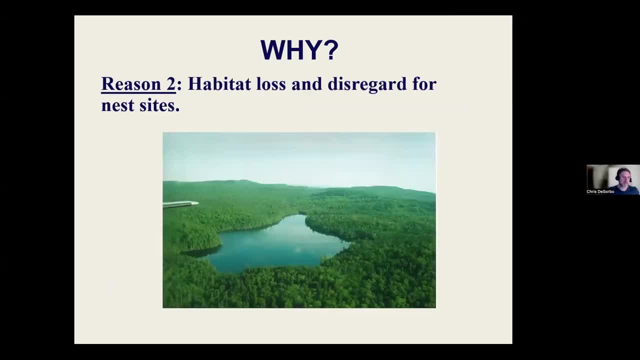 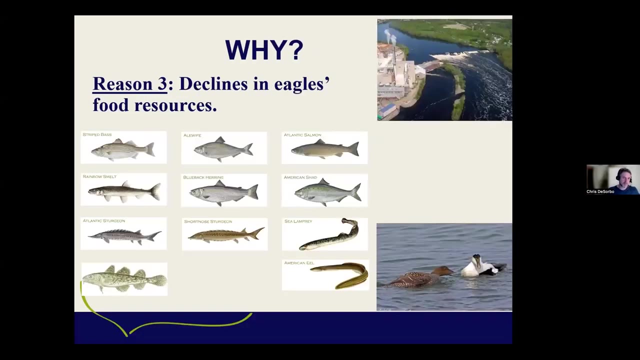 And then that was overruled by federal legislation. Then habitat loss and disregard for nest sites is a factor. People were basically, you know, disturbing, cutting down trees etc. We also were pretty significantly impacting the food resources of eagles at the same time. 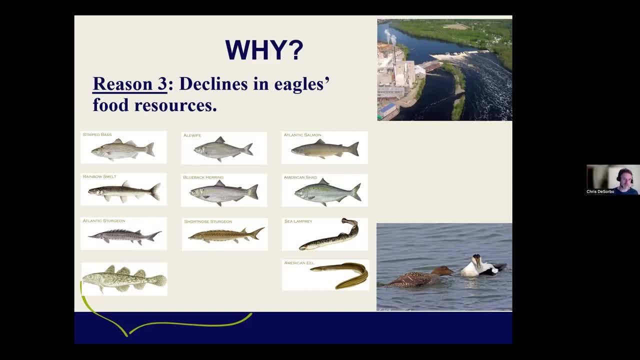 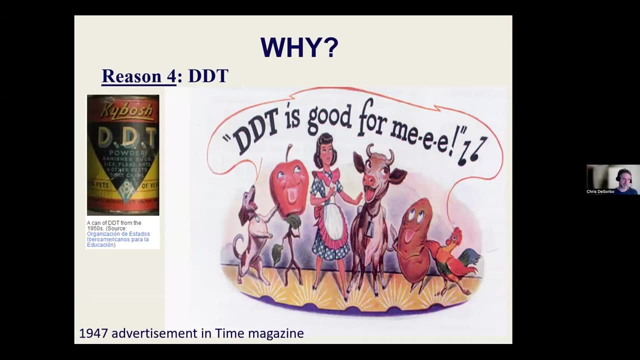 So a lot of the anadromous fisheries that, some of which we see recovering a bit today, were pretty decimated back in those years. But the reason that is overarching in everyone's mind and is critically important was DDT, which is a insecticide that was 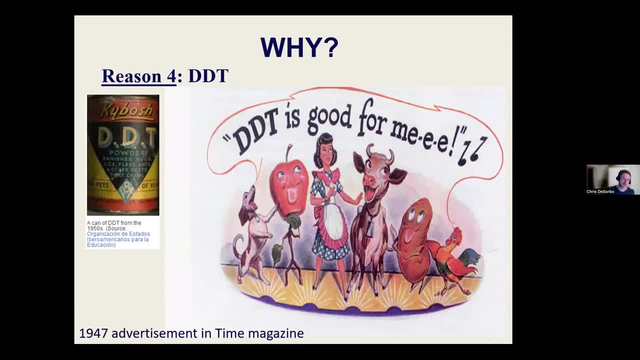 broadly distributed throughout throughout the country, And it's still actually used in some other countries today, And so I always like to show this slide as a reminder of you know, the the messaging around things you know is is just good to take note of. So this was in Time Magazine Turned out to be one of the most devastating environmental disasters that impacted all kinds of species, particularly the high trophic level species, and particularly raptors like eagles, ospreys, peregrine, falcons. 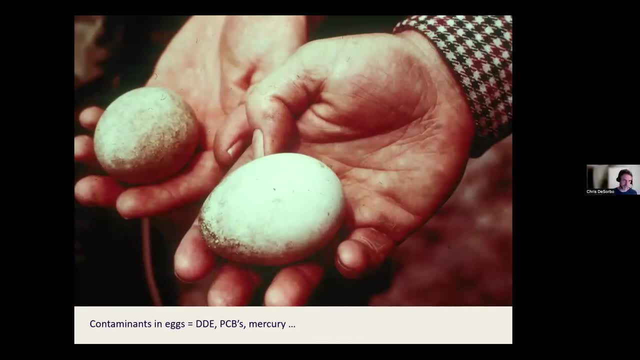 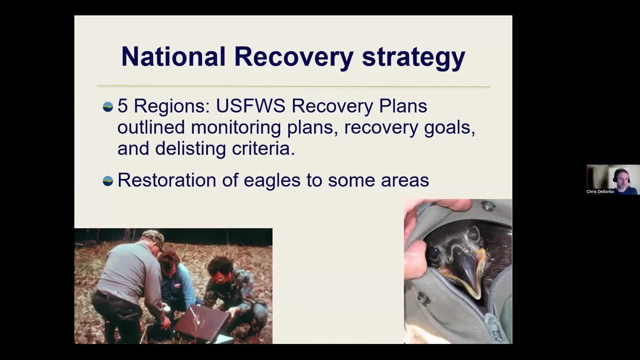 Once a bird had depurated DDT, which broke down into this other compound, DDE or PCB, into eggs, then it weakened the eggshells. The birds would sit on the eggs and they would break. PCBs were also a concern and mercury was also known. 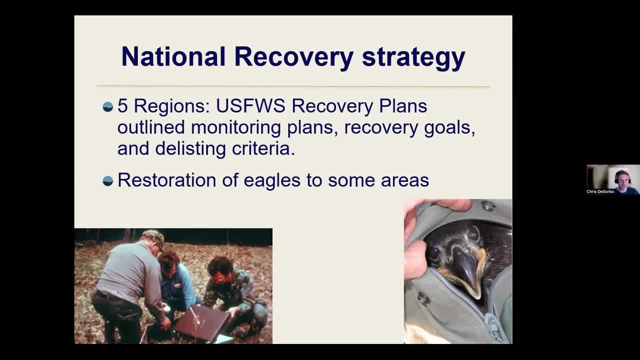 and noticed back in those early days as well, So a national recovery strategy was devised. The US is broken up into five regions, which each had their own monitoring plans, recovery goals, delisting criteria And eagles were restored to some areas through hacking. 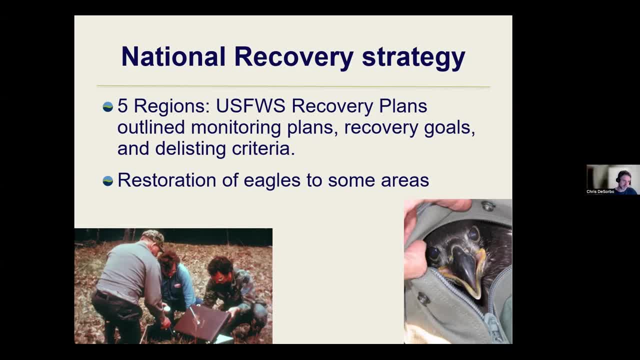 So chicks were taken from some clean quote unquote areas and brought and hacked out in towers in some areas. So New York State is really famous for this work. In some cases, eggs were taken from clean sites and transplanted into nests in places like Maine. 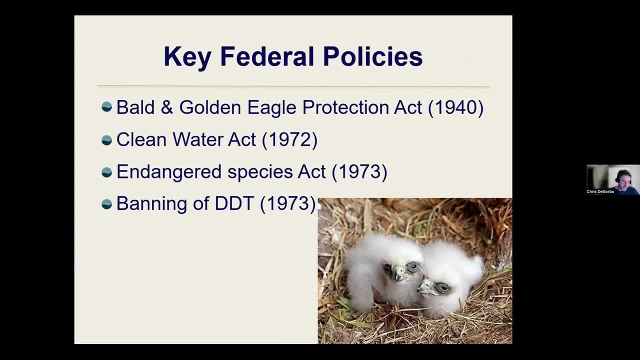 The key thing about the history of bald eagles, I think, is just it really demonstrates effective environmental policies: The Bald and Golden Eagle Protection Act, the Clean Water Act, Endangered Species Act and the eventual ban of DDT- And all of these things were remarkably important. 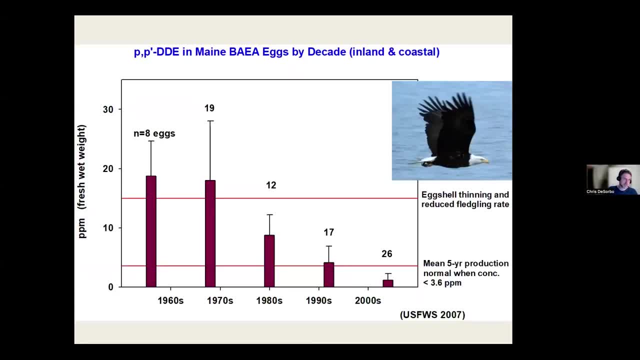 in the recovery of bald eagles. So this graph shows DDT, which again, DDE and DDT are essentially the same thing for this conversation, But it just shows the decline in DDE over time, Back in the 1960s all the way through the 2000s. 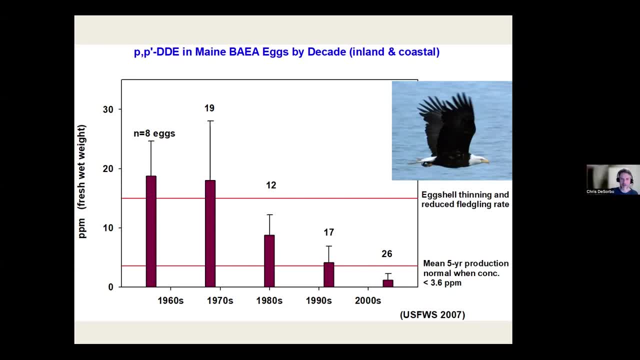 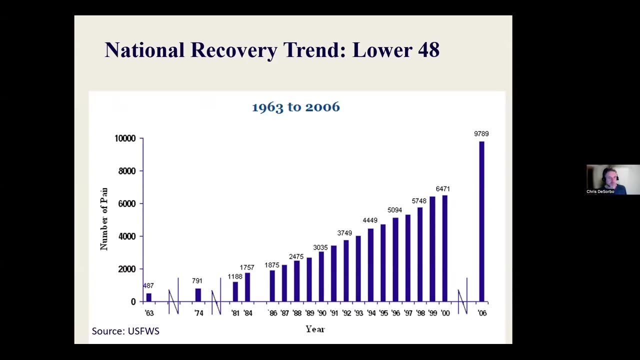 that bottom line is a line associated with normal productivity, essentially, And the upper line is associated with eggshell thinning. Some areas, like the Great Lakes, experienced deformities and things far worse than what we experienced here. So this is a graph out of a US Fish and Wildlife Service. 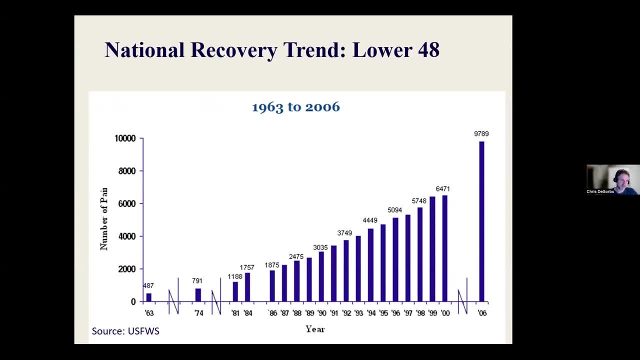 report showing the number of pairs nationally over time. So you have back in 1963, there's 487 pairs in the lower 48, up to 2006 where they had 10,000.. I actually don't have the current number. 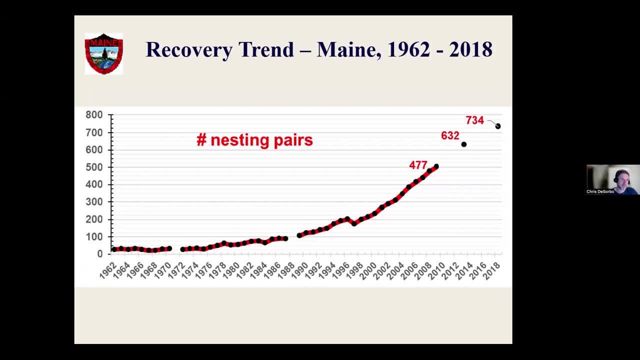 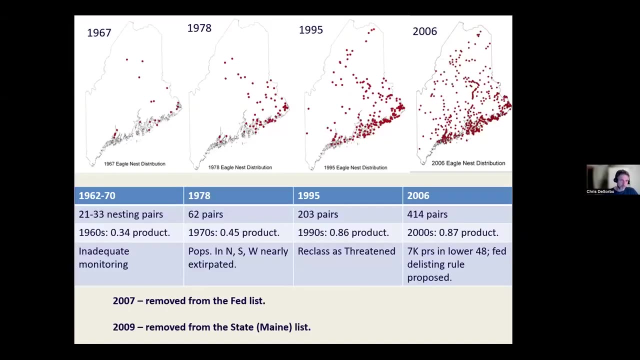 nor do I have a graph showing it, But this was the trend in Maine's population from 1962 up to the very last statewide survey, conducted in 2018.. So you had 734 pairs- Far more now. This just kind of shows the distribution. 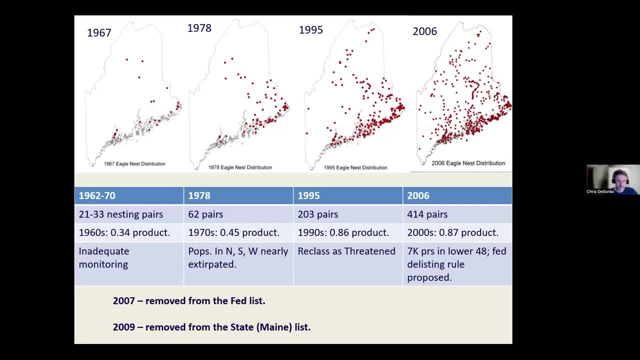 of those pairs over time. So you can see, you know eventually you see the whole Penobscot River corridor getting you know, traced here Coastal Maine, especially down east Maine, are pretty important And you can see productivity, which is the chicks. 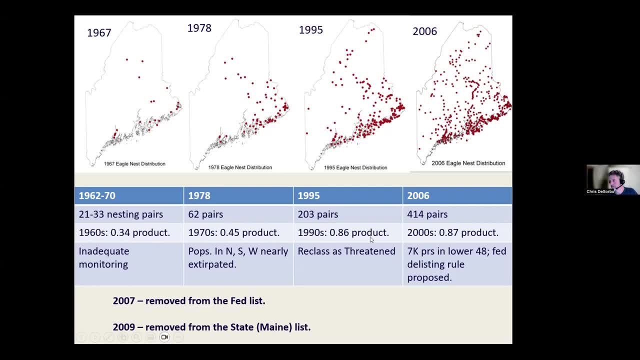 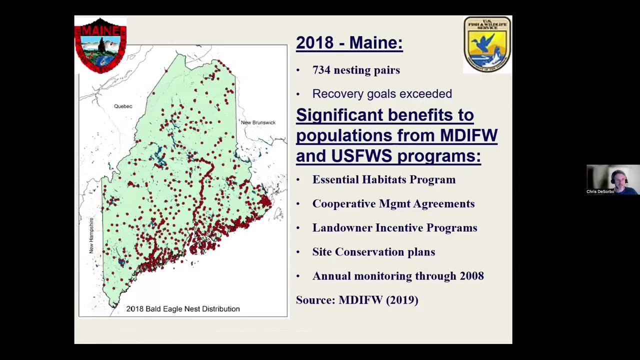 produced per occupied nest steadily improves over time. So the population stabilizes. It's continuing to expand. 2007, it's removed from the endangered species list In 2009, it's removed from the state list And this is the current. 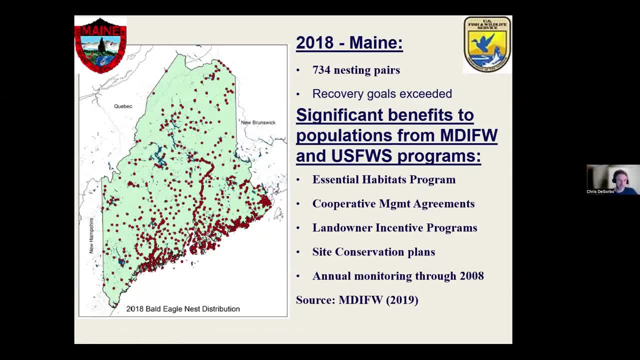 the last snapshot of the distribution that we had. There's still some monitoring going on, but nowhere near the monitoring that was going on all the way through 2008 and then incrementally beyond. So it's an important demonstration of a bunch of programs too. 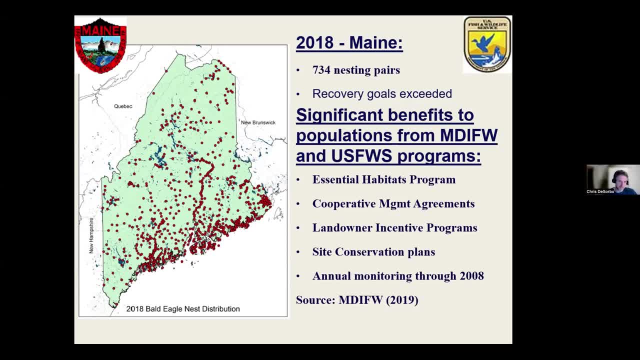 like the Essential Habitats Program that IF&W has Cooperative Management Agreements, Landowner Incentive Programs. Landowners play a huge part in this story And there's a bunch of recovery goals that are outlined in IF&W's report on the recovery. 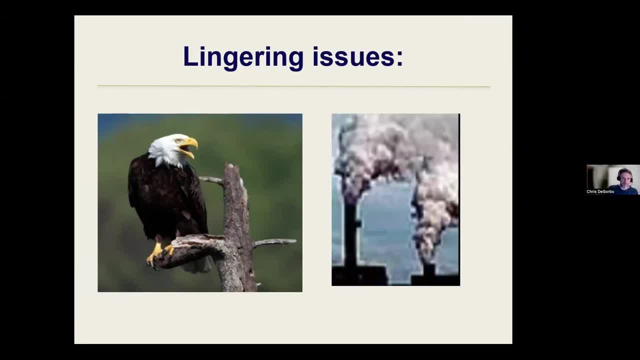 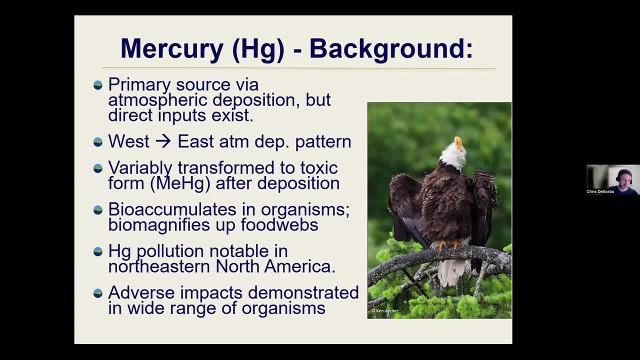 So lingering issues. I felt it would be worthwhile to at least touch very quickly on some of the things that are still of concern for eagles, One of them that we've focused on a lot. So this is going to be basically three quick segments. 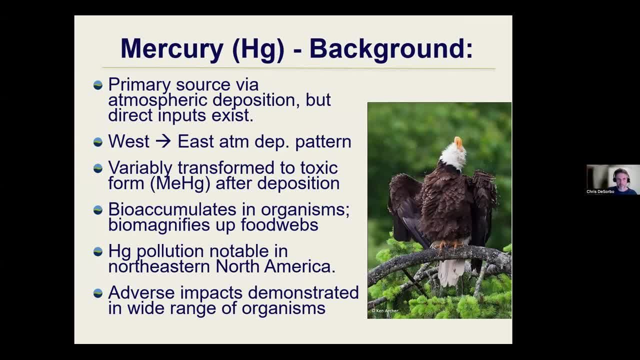 on mercury-lead PFAS. So mercury, for those who don't know, is atmospherically deposited, But there's still places like the Penobscot, the lower Penobscot River, where historic direct mercury inputs occurred, And we're still studying that today. 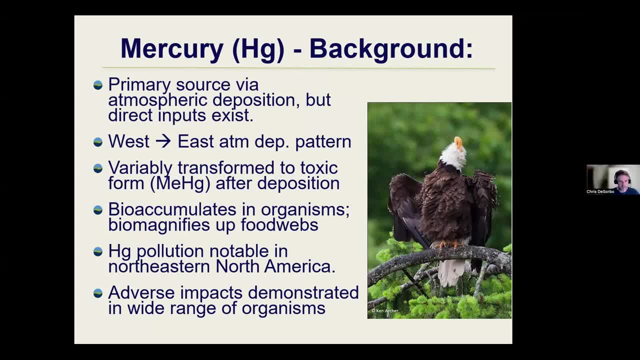 But there's a west to east trend in deposition And that mercury landing on the landscape gets transformed into a more toxic form And then it works its way into organisms and then builds up across the food web. It's called biomagnification, So that pollution is actually most significant. 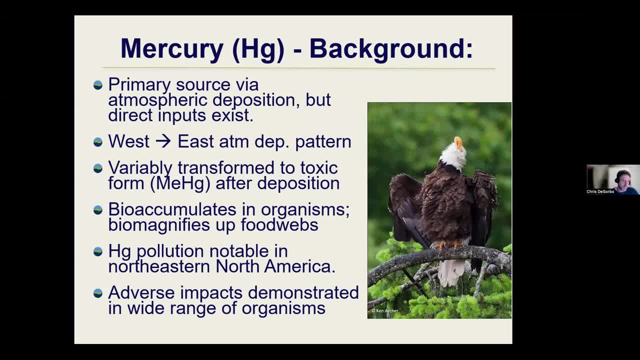 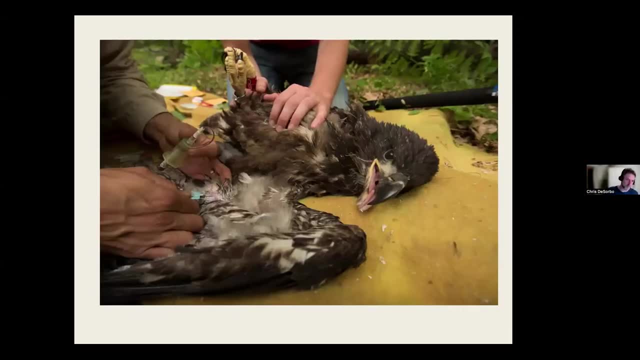 in northeastern North America And the impacts of mercury are basically demonstrated- negative neurological and other impacts demonstrated in a wide variety of organisms. So we would go out and when we're doing that banding work, we're really interested in collecting samples for these types of things. 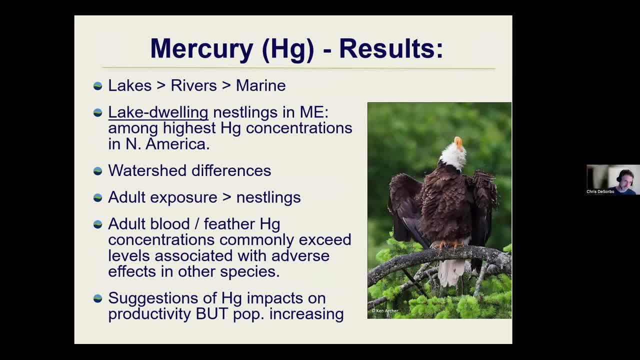 And the findings of that work to date are basically that mercury exposure in eagles is greater at lakes than rivers, greater at rivers than marine systems, But lake-dwelling bald eagle nestlings in Maine have some of the highest mercury concentrations in North America. 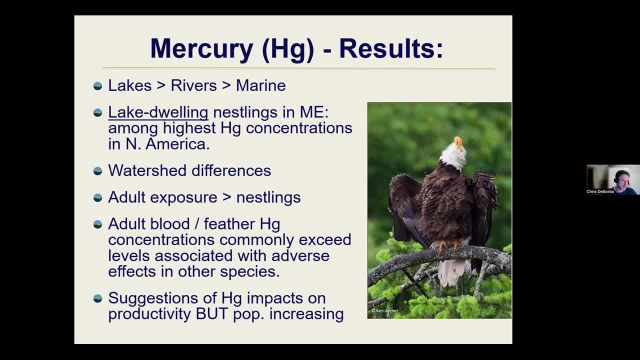 There's watershed differences. Adults have much higher exposure than nestlings due to growing feathers where they dump that mercury, And the levels of mercury in adult eagles and adult feathers commonly exceed levels associated with adverse effects in other species. Haven't really figured this out in eagles per se. 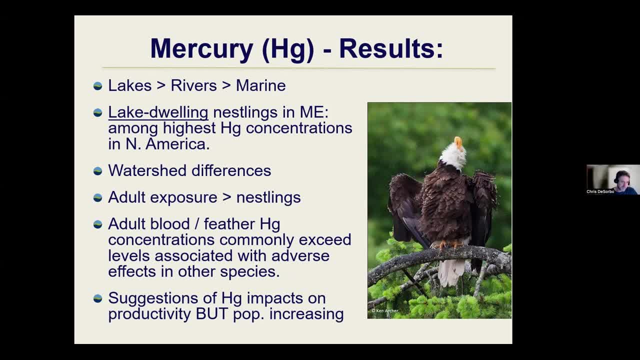 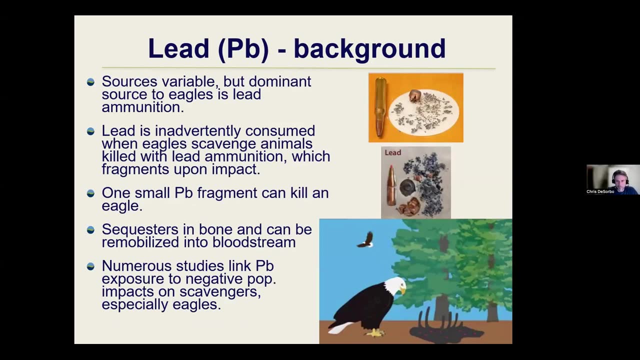 So, but our work to date suggests that there are some relationships between mercury exposure and productivity. but we're still working on just going through that analysis. Pivoting to lead really quickly. Lead poisoning has been an issue for bald eagles and other scavengers for decades. 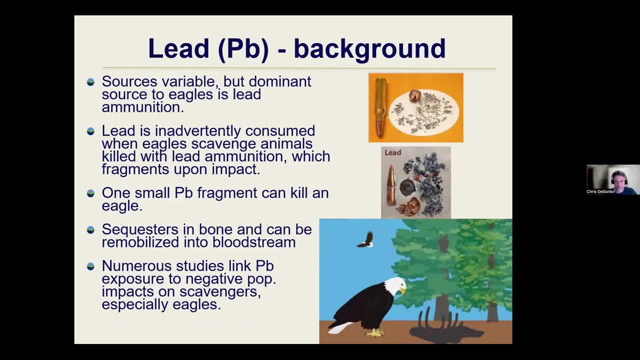 The problem is worldwide. This occurs in the US despite the fact that lead was banned for waterfowl hunting in 1991.. Sources are variable, but the dominant source to eagles is lead ammunition. Lead is inadvertently consumed when eagles scavenge animals. 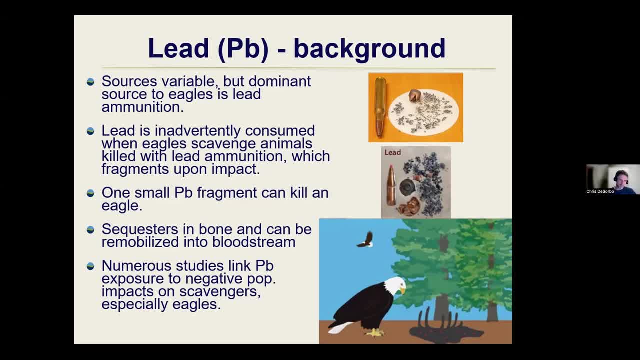 that are killed with lead ammunition. Lead ammunition fragments upon impact and then eagles will go in and eat the gut piles or animals left on the landscape, And one small fragment of lead can kill an eagle. Once it's in their bloodstream, it sequesters in bone and it can be remobilized. 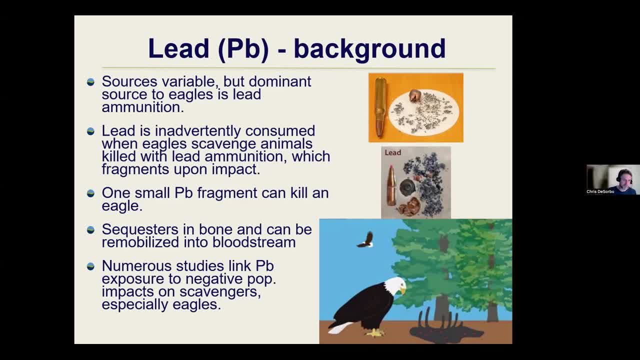 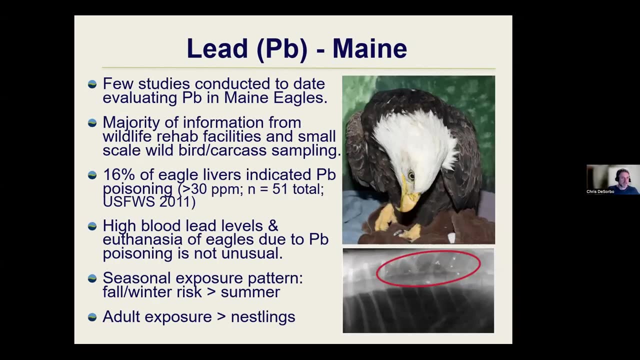 And there's a number of studies now that link lead exposure to basically reduced resilience of populations in populations of eagles impacts on other scavengers. So not much has been actually studied in terms of lead exposure in Maine, though, So the majority of information we have 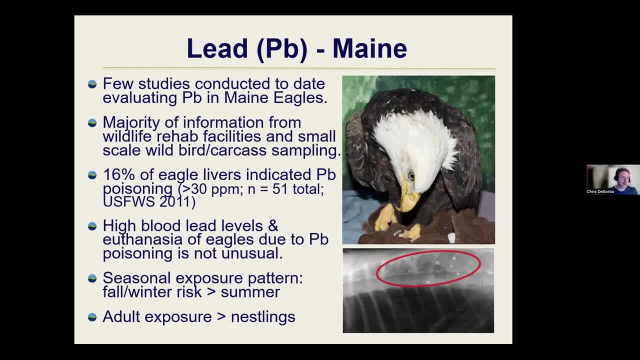 is from wildlife rehab facilities. If they get a bird in that got hit by a car, they'll test it for lead. Or if they get a bird in that's showing you know some neurological signs or interesting behaviors, they'll. I think they might routinely test them now. 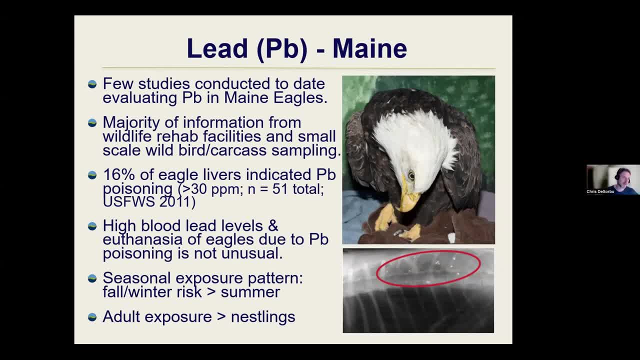 Back in 2011,, Steve Marzakowski from the US Fish and Wildlife Service did a study looking at lead concentrations in bald eagle livers And 16% of those indicated lead poisoning. We found, you know, high blood lead levels. 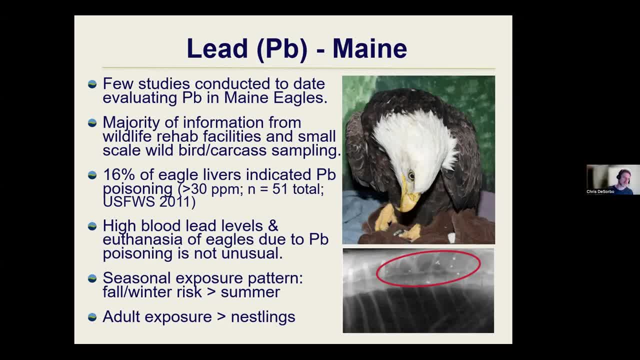 in some individuals at rehab facilities And I would say you know some of these birds are euthanized. It's not terribly unusual. There's a seasonal pattern where the cases tend to increase in the fall and winter, fewer cases in the summertime. 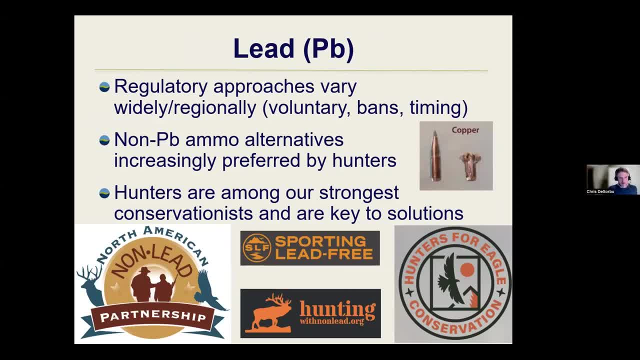 And so the regulatory approach is very widely and regionally. I'm not gonna get into it, but some are voluntary, some are bans, And now there are non-lead ammo alternatives that are increasingly preferred by hunters for just better ballistics, and the fact that you know. 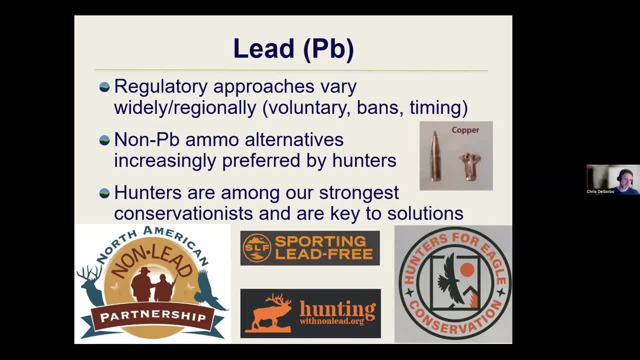 it's not contaminating the environment. So hunters tend to be some of our strongest conservationists and they are key to the solution. Now there are a lot of organizations out there, like the North American Lead Partnership run by the Peregrine Fund. 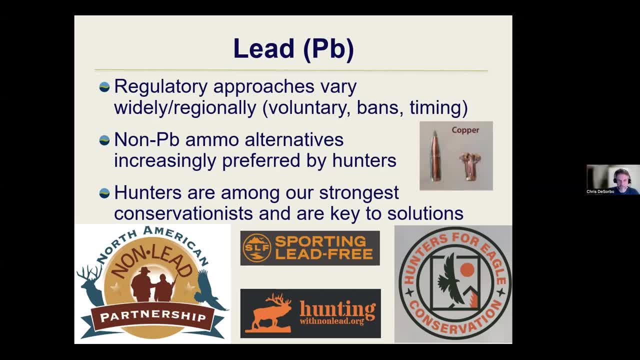 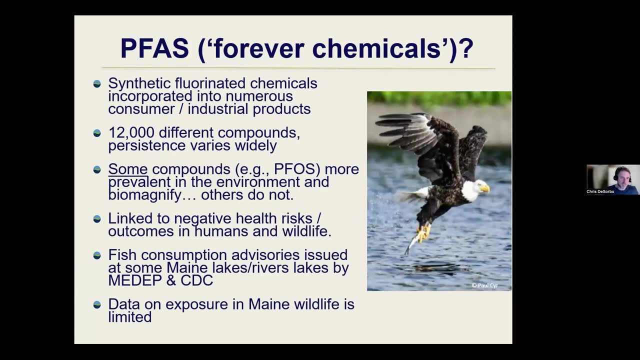 Sporting, Lead, Free Huntingwithnonleadorg and Hunters for Eagle Conservation and others that are taking this approach of trying to approach hunters, with hunters to talk about this problem. Last quick bit is that we're actually working on now is just a quick touch on PFAS. 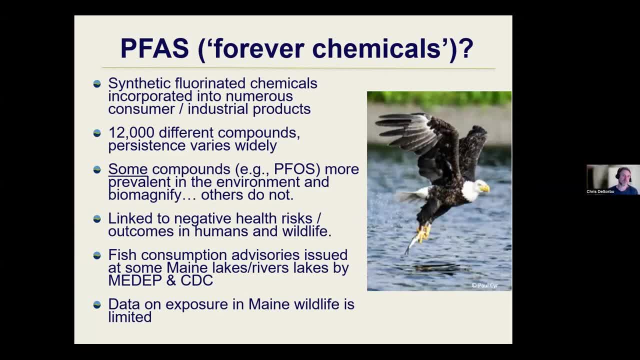 We've started broaching into this with not only eagles but loons and ospreys. PFAS are essentially these synthetic fluorinated chemicals that are incorporated into all kinds of consumer products, So firefighting foams sludge containing biosolids. 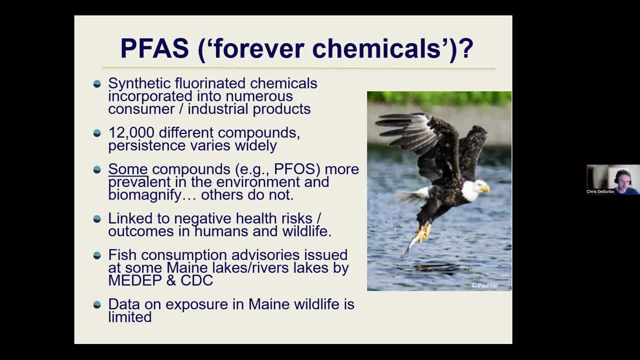 Everybody's probably heard, this is a big problem in Maine. Teflon coatings, water repellent treatments, food packaging- It's in basically all kinds of things around the world, All kinds of things around us. There are 12,000 different compounds of PFAS. 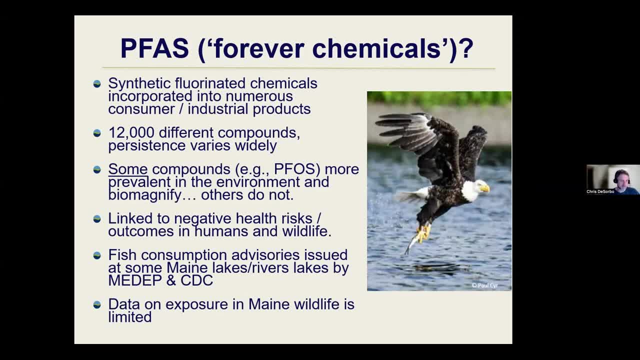 And some of them are more prevalent in the environment and bio magnify than others, And many of those compounds are linked to negative health outcomes in people or wildlife. So at some lakes waterways in Maine there have been fish consumption advisories issued. 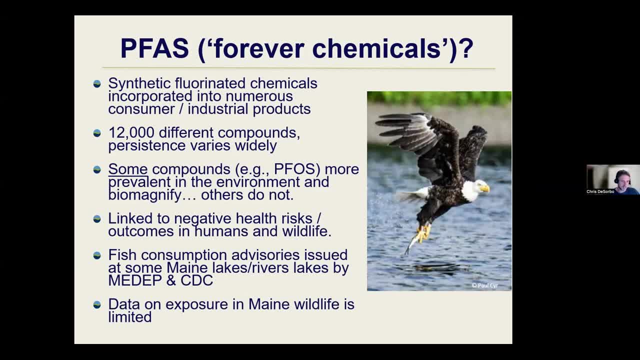 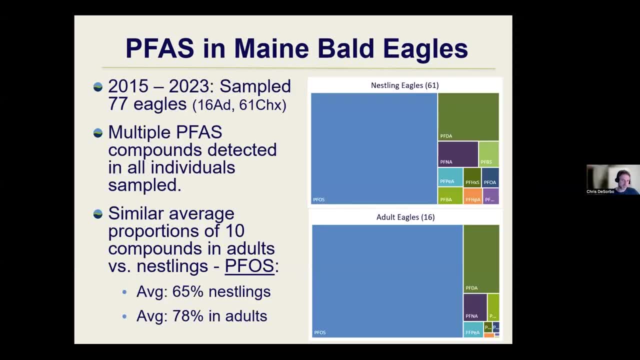 by the Maine CDC and the Maine DEP due to PFAS exposure in fish, And there's really been very little work done in Maine. So this is literally, you know, we've just barely finished the first look at some of this data. 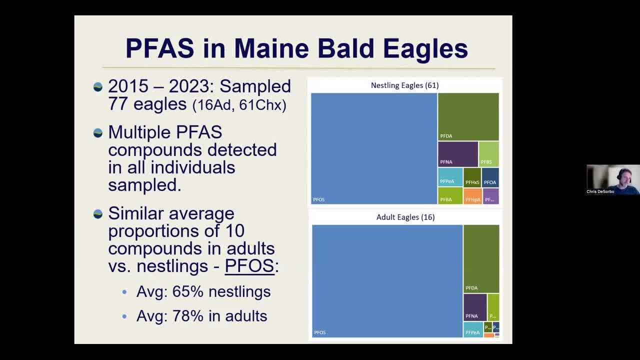 So I scrambled to actually put some of it in here, But we sampled 77 eagles, about 16 adults and 61 chicks for PFAS. Most of those samples were collected in recent years, but we used archive samples for a few. 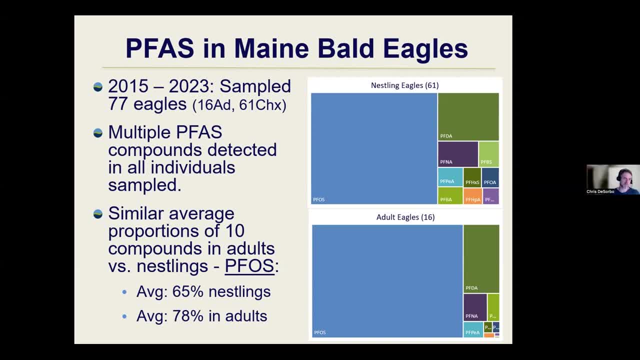 And basically multiple PFAS compounds were detected in all individual samples, So we analyzed 10.. This is just a summary of 10 different compounds And you can see essentially the blue box is just a proportional representation of this most prevalent compound, PFOS. 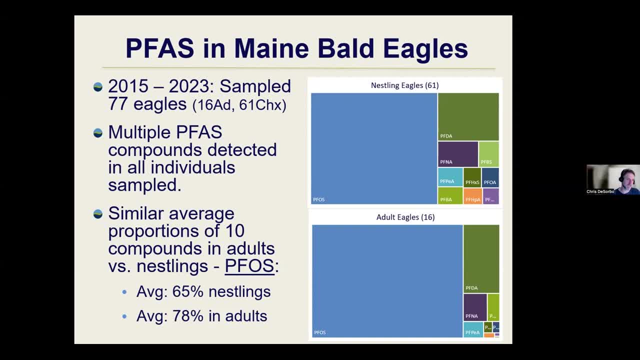 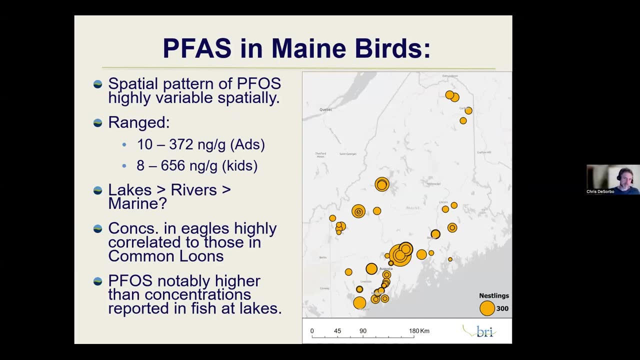 Then you have other ones like PFDA and PFNA, And all of these have a different chemical structure. Proportions are about similar between adults and nestlings. This is what the distribution of those spatial patterns look like in Maine. We're still trying to interpret what that means. 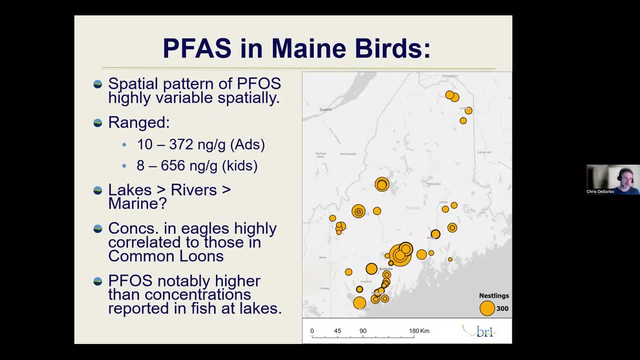 But you do see some reflection of higher PFAS concentrations, or PFOS in this case in central Maine that is known for some of these problems. It appears that lakes are higher than rivers, but we really haven't sampled rivers And we've also learned that concentrations in eagles 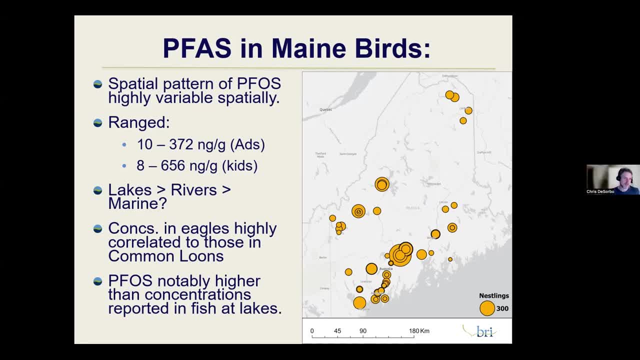 seem to be pretty well correlated to what we found in common loons. There's a different story for ospreys that I won't go into, but it does seem like there's just different patterns in all these species, depending on what habitat and what region you're in. 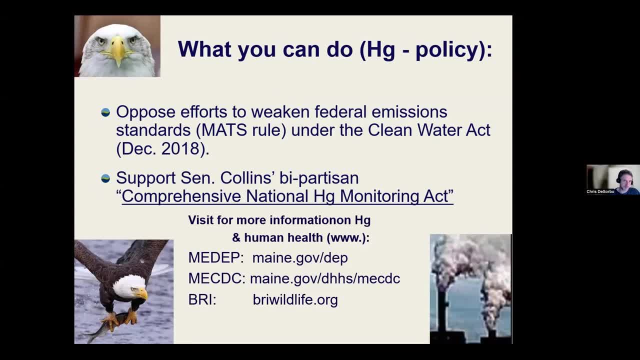 And so off to the what you can do things. I know I'm kind of running over here. The two things I put in terms of what people can do about mercury is just be aware of some of the politics going on occasionally about mercury: The Matz rule, which is the mercury and air toxics standards. 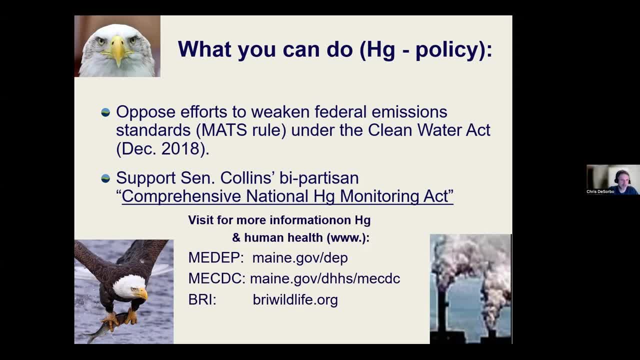 has been under some fire for a while. So I feel like if people can just keep an eye on that and support, oppose efforts to weaken that rule. that's important for environmental health And Senator Collins put in a comprehensive National Mercury Monitoring Act as well. 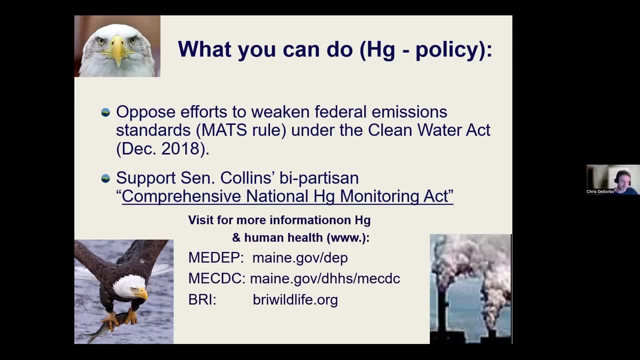 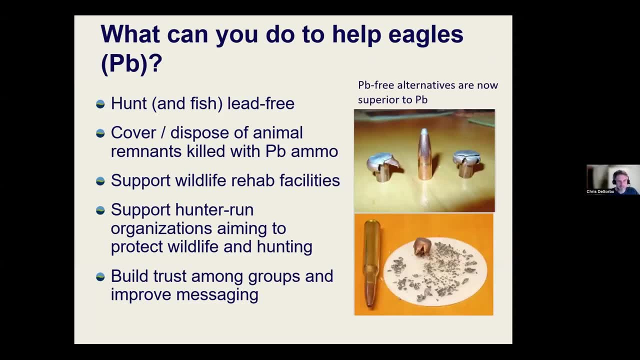 I put some websites there. if people want to learn more about mercury, There's a ton of information on DEP's website, Maine CDC and ours On the eagle front. it's kind of obvious: hunt and fish lead free. People can change their practices about what they do with gut piles. 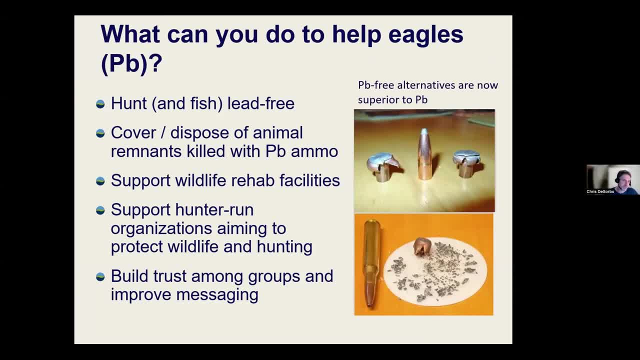 Wildlife rehab facilities actually are playing an important role here and support some of those hunter-run organizations that I mentioned before, And I feel like this last point is kind of important on that topic- just to build trust among groups and improve messaging. That's kind of the part of the problem on this. 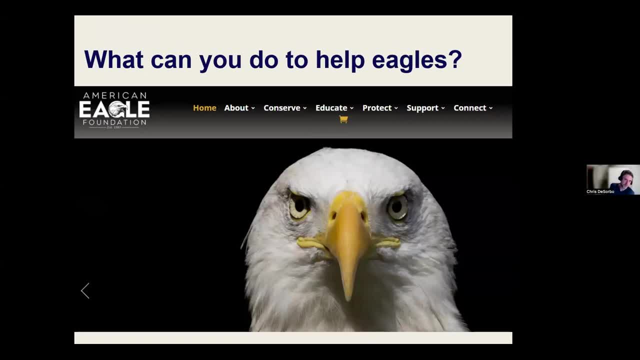 Another group that I just have to a couple last shout outs is the American Eagle Foundation does great work supporting not only bald eagle work but golden eagles. They've supported a bunch of the work that we've done over the years and I'm grateful to them. 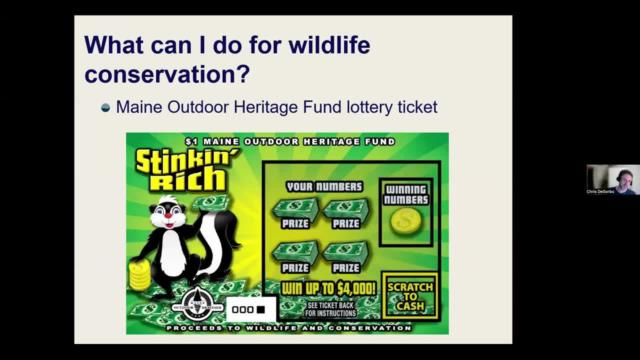 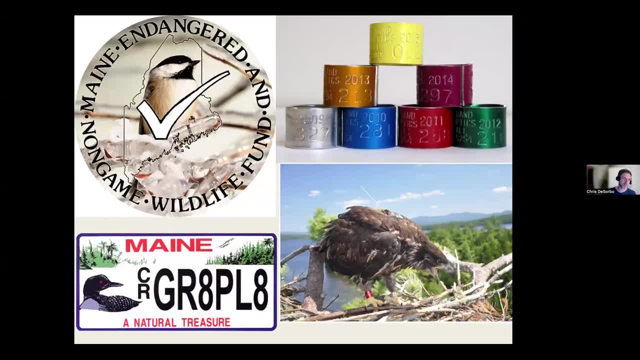 The Maine Outdoor Heritage Fund has funded a ton of. I think of them as seed projects that have gotten all kinds of research up and going, including work with eagles and other projects at BRI. And then there's the Maine Endangered and Non-Game Wildlife Fund. 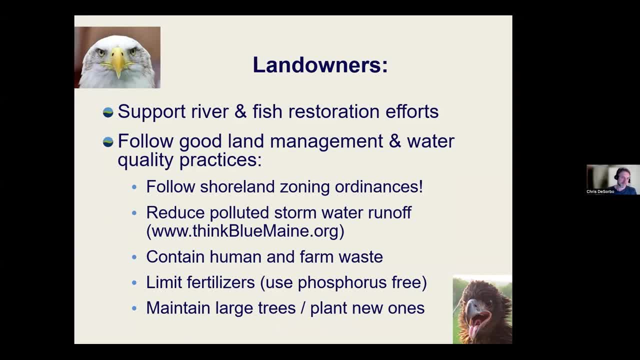 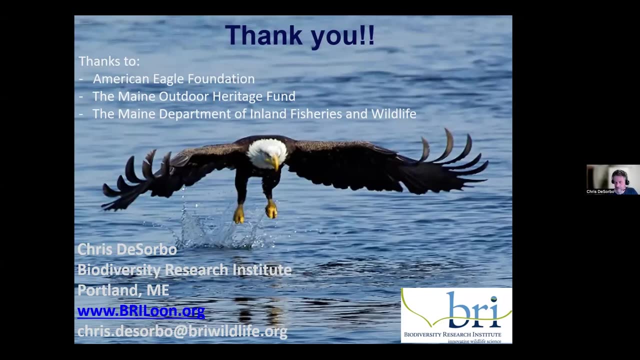 IFNW has been a great partner. All the kind of typical things that people should probably already know in this group about landowners. Excuse me So I won't go into that. Anyway, yeah, I'll leave it there. Yeah, I'll take any questions. 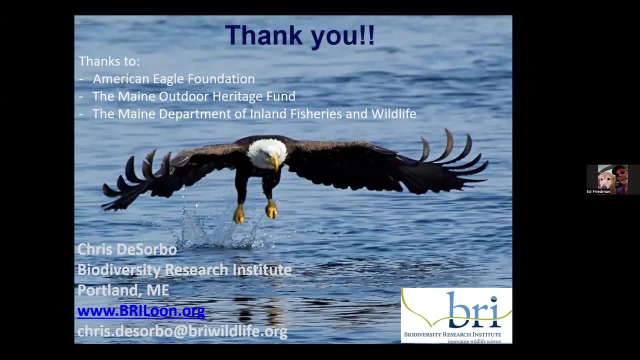 Great. Thanks so much, Chris. That was great. I have a few questions and there's also a couple of things in the chat room. Let me ask just first if I heard it correctly when we were looking at some pictures of young eaglets? 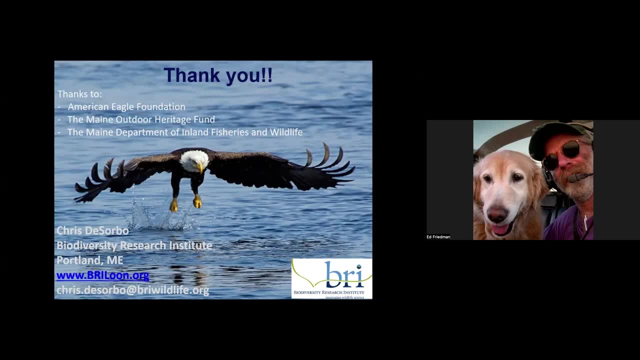 you talked about the plumage not being ready when the time came to fledge. Yeah, And I didn't quite get that. I mean, they're not going to have a hard time learning to fly, Why would they be fledging earlier than they are ready? 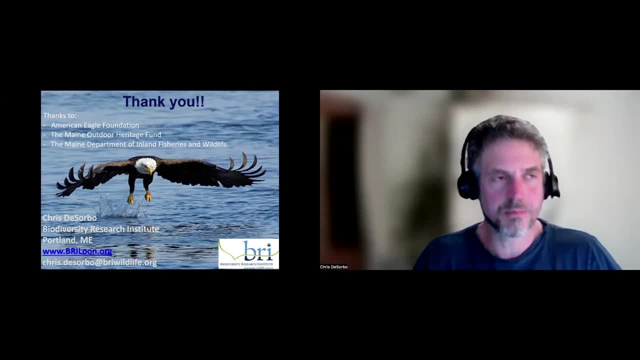 Yeah, So I pointed out the feather sheath on that one picture of the nestling And so basically, if you caught an eagle the week that it fledged, there'll still be part of that. Part of that feather is still in sheath. 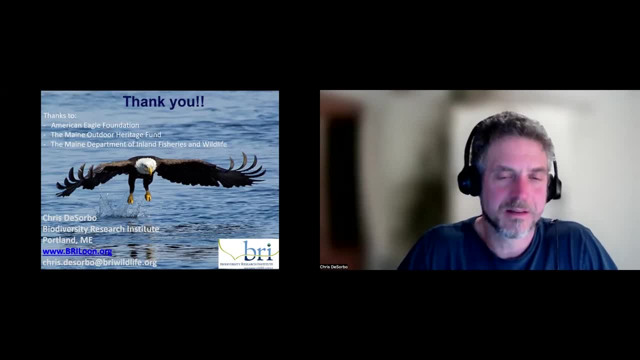 This great bunch of studies by this guy. Gary Bortolotti went up documented a lot of these things. But basically, why it's that way? I guess it's just beneficial to them to get out of the nest. They have enough feather material to fly. 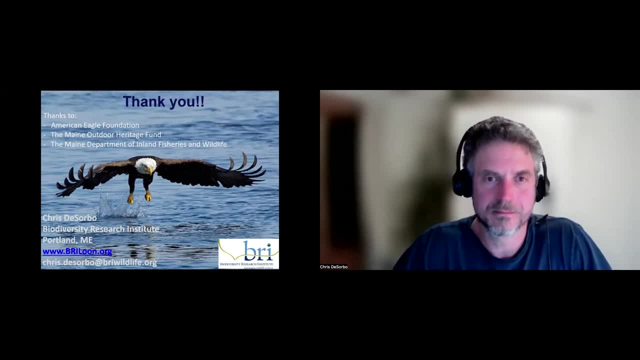 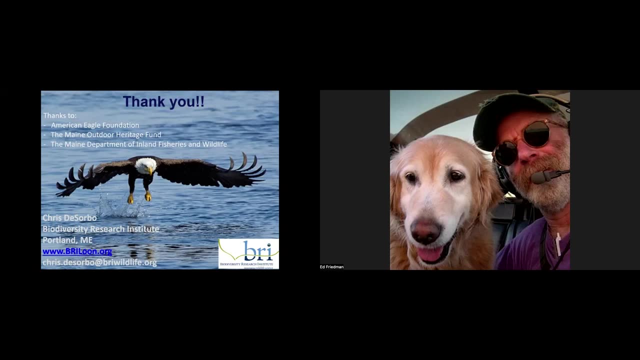 but their feathers are still growing, Yeah, And, as I recall, actually, even once they fledge, they're still being fed for quite a while by their parents, Right? Yeah, So it may be a real estate issue in part, right? 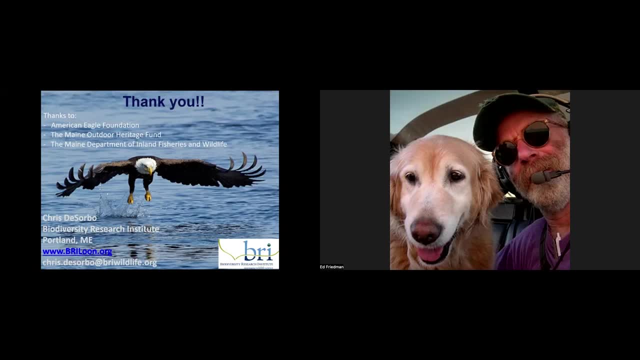 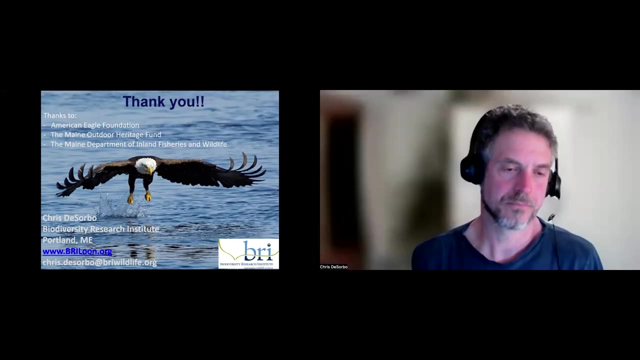 Because they can push each other out once they get you know at any time. Yeah, Yeah, Okay. And then there were a couple of acronyms. I saw There was the acronym UD, used in some of those population slides, but I don't know what that meant. 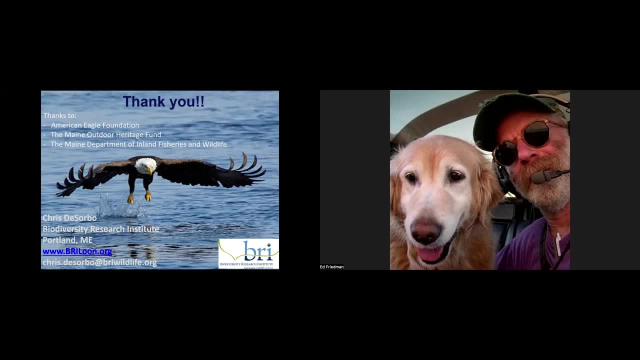 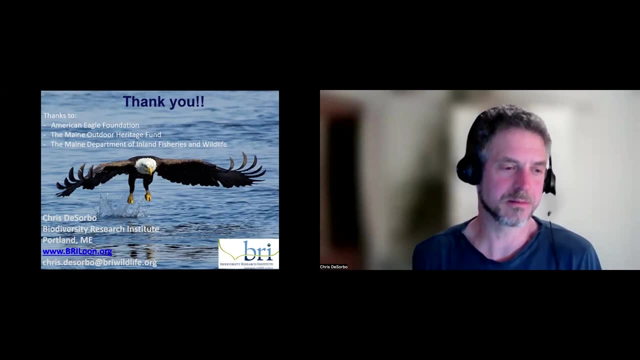 And then there's a BAEA used. What is it Gotcha? Yeah, Some of that stuff was on some maps that we had in some reports And that was probably explained in the captions. But UD stands for utilization, distribution. It's essentially 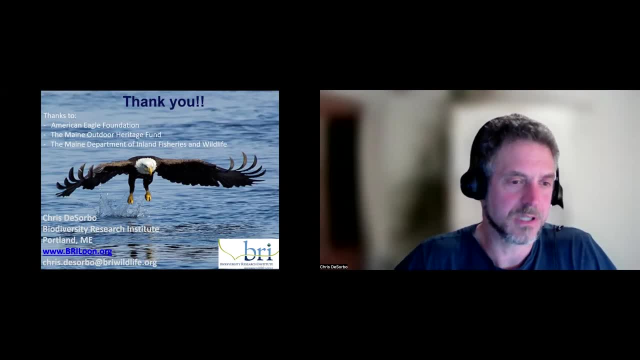 just a representation of use that takes into account for the models we did Kind of space and time use. So utilization distribution is basically: you could just shorten it to a use area if you wanted to. BAEA was just the AOU or the 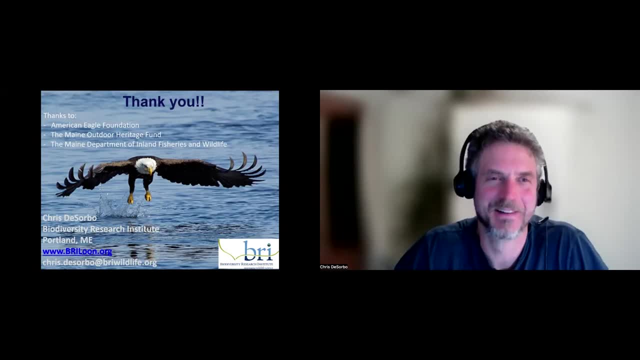 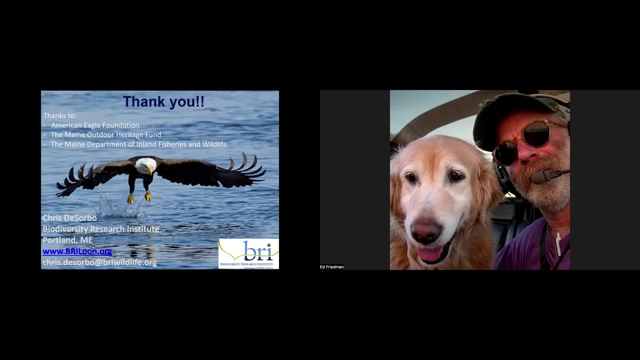 the bird abbreviation for bald Eagle. Sorry, Okay, All right, Thanks. Nick is asking here: What about lens from fishing tackles? Is that a problem too? We know it is with loons. I'm going to guess: Yeah, It's a good question. 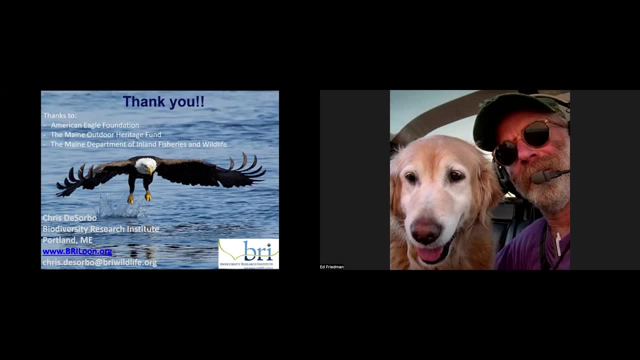 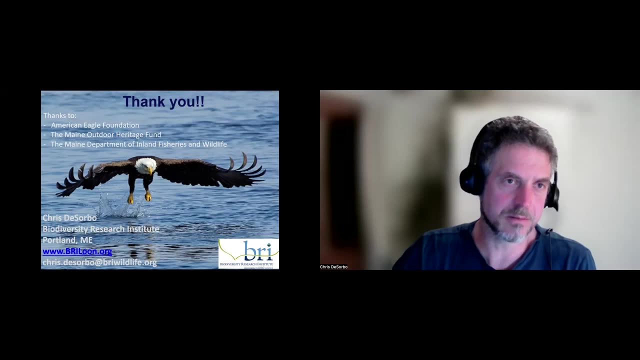 I didn't get into lead for loons and other water birds, But there's this. Yeah, there are. That is obviously a big issue for for those Species. As far as I understand, Very few lead sinkers from fishing tackle or found in. 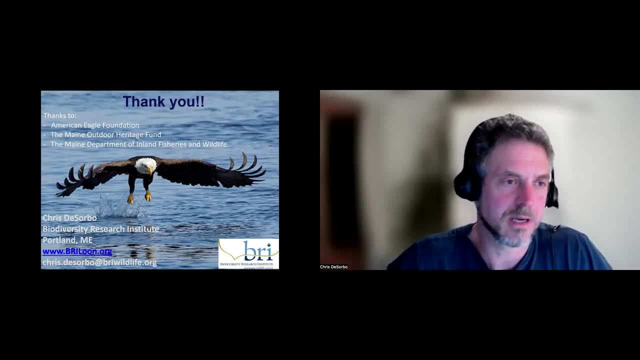 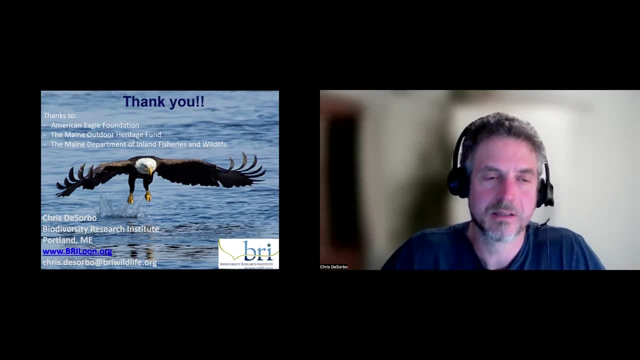 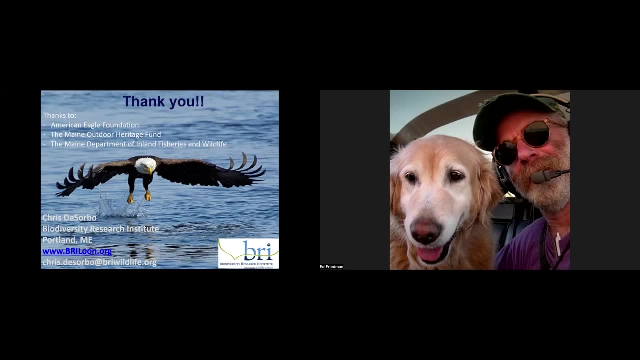 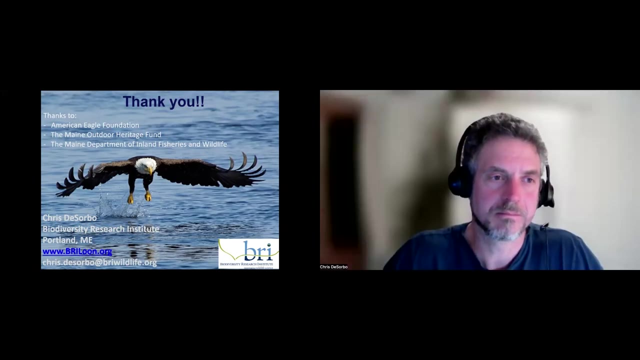 I just don't think there's actually as many cases of it. Okay, And Nick also said it'd be interesting to overlay the toxin geo data with the maps you showed earlier for preferred roosting. Yeah, Yeah, There's. there's increasing number of studies now. 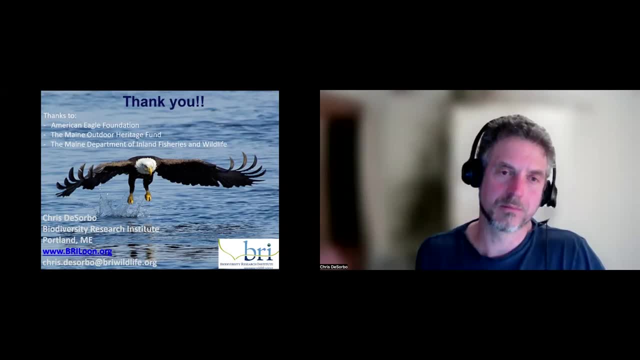 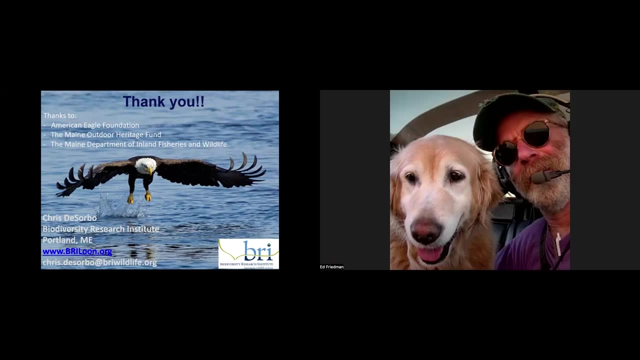 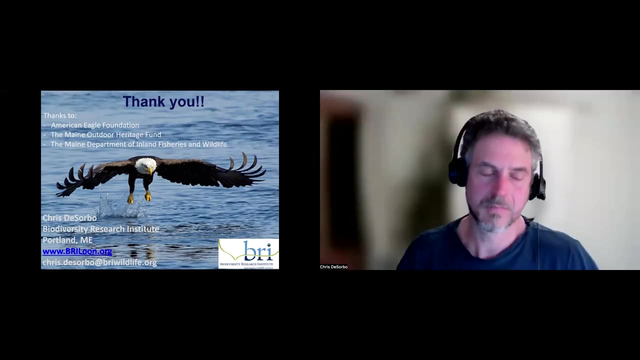 Or, um, people are using movement data to look at exposure to contaminants and risk and things. christine asks: how is climate change affecting food resources and general evil patterns that you might be seeing? yeah, for for a species like eagles they're relatively opportunistic, you know. sadly, you could refer to eagles as a glorified scavenger. 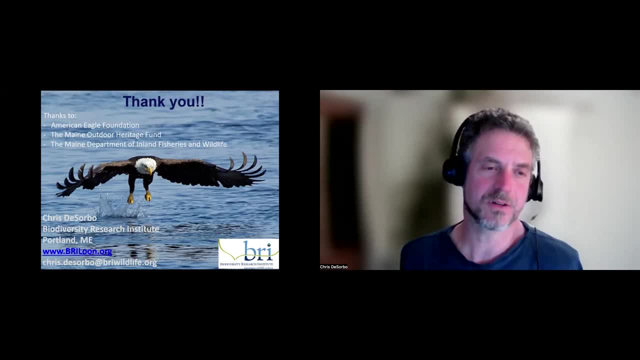 so, um, so, if, if there's, you know, for a lot of species, the the key is in the food, if they have adequate food resources. you know, that's the number one important thing: how climate change is going to affect the food web in all of these different areas. 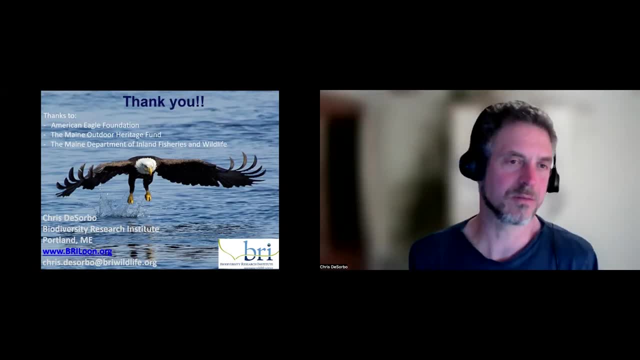 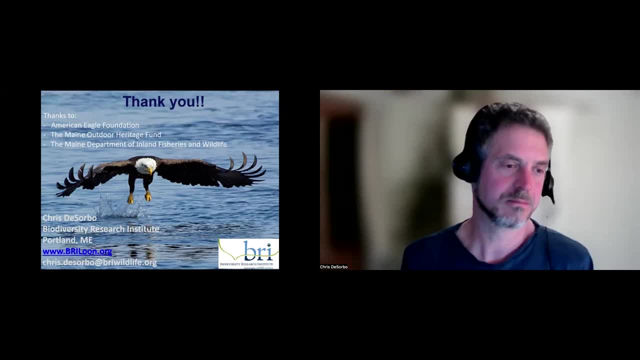 of one of the fastest warming, if not the fastest warming, uh, pocket of water in the world. uh, so there are likely cascading effects, but, um, it's probably on a case-by-case basis. and, yeah, i, i don't know, i think, if i would much rather be an eagle than a bicknell's thrush. 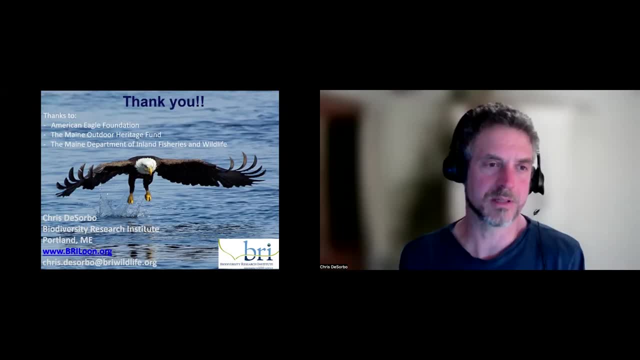 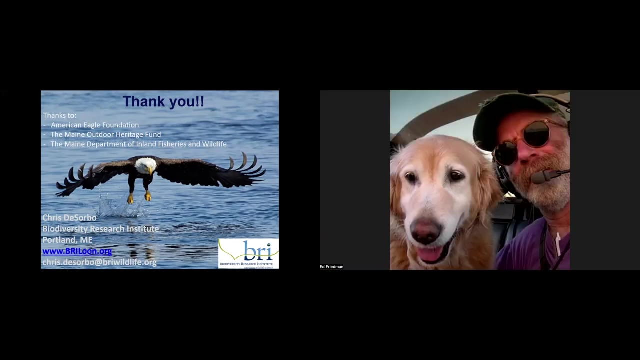 whose you know habitat is gonna go off the top of the mountain and they have nowhere to go. eagles will probably be better off than a lot of species, but you know it probably wouldn't take me long to come up with some impacts. but yeah, i really don't know. um lorraine has an. 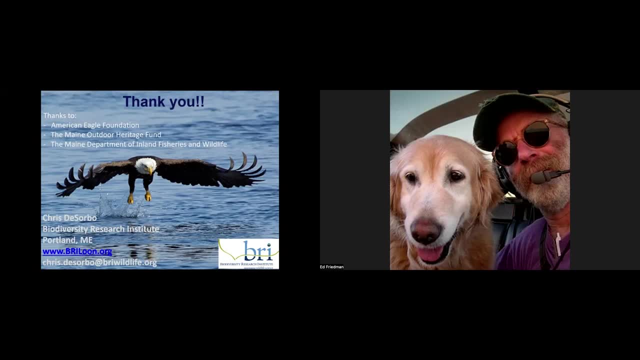 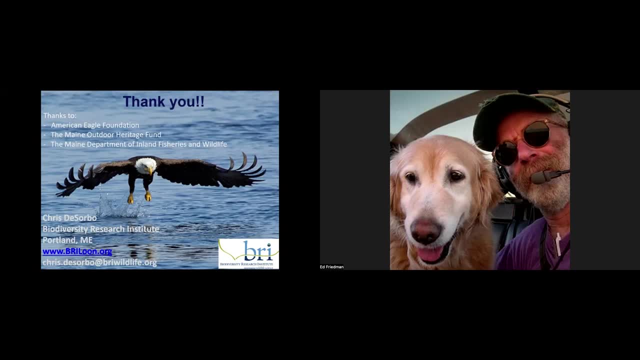 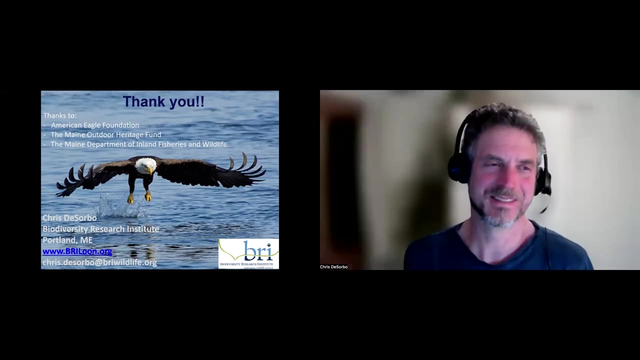 through the chops, um, where the vamp is out, you know, into the comeback and fast, fast flowing water, going downstream, standing on a piece of ice and then leaving that, flying back up river, getting on another piece of ice and going back down again for trolling, for- uh, trolling for food, or both do. 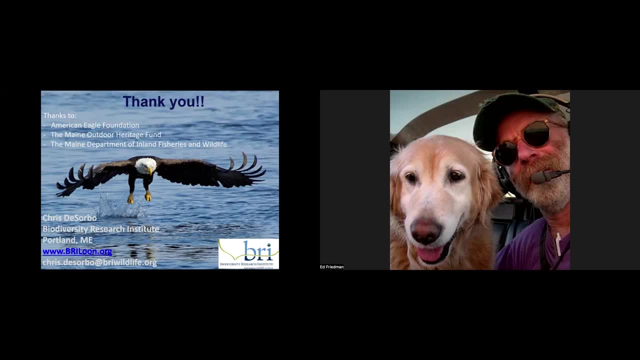 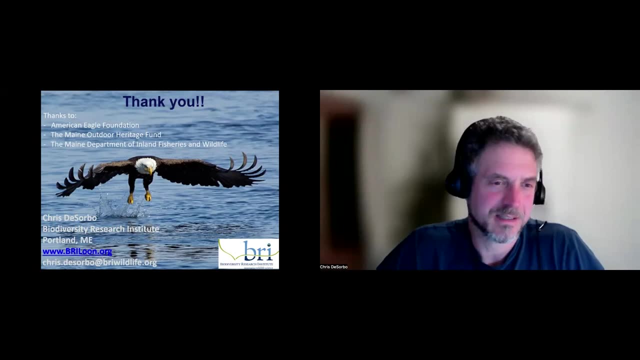 you think she didn't. she didn't see any any obvious, you know, hunting or fishing, uh activity going on. but uh, yeah, that's a cool observation. i wouldn't be surprised if the bird was sitting there waiting, but um, it, it's a little more of a. 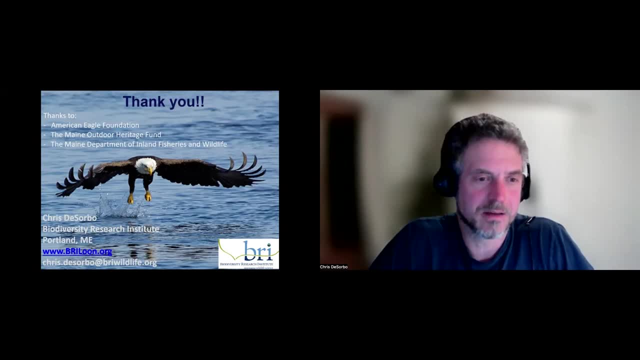 difficult spot for an eagle to to grab prey from a ice flow. uh, they can, you know, they can go in the water, but they, they might have to swim to shore, you know. um, whereas that so? that's why, you know, a lot of times you'll see eagles just perched up in the trees and coming down and whacking a fish. 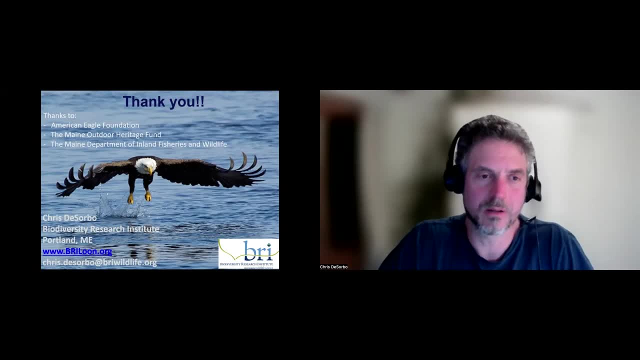 they can't really pull themselves out of the water like an osprey can, so but yeah, i would still feel like there's got to be something going on there. it's a really cool observation. um related to that a little bit. do you have any, you know? 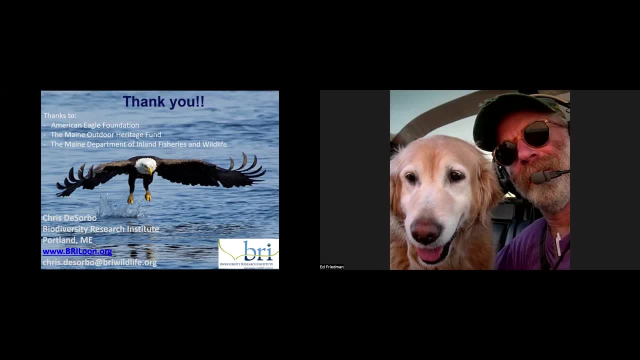 everyone is seeing eagles. you know. go harass osprey and get them to drop their fish right. you know they're good thieves. do you have any? anyone watch eagles enough to get a sense of you know if they're osprey in the area, you know is that like 80 percent of the time they're. 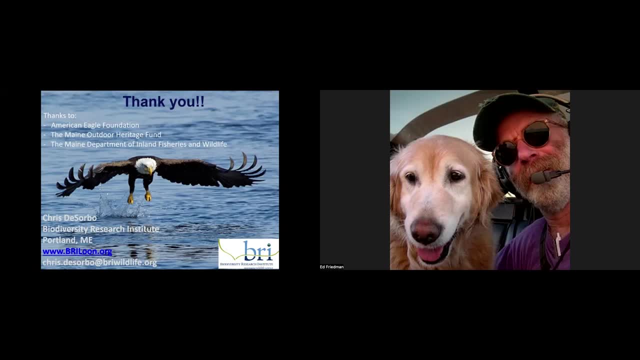 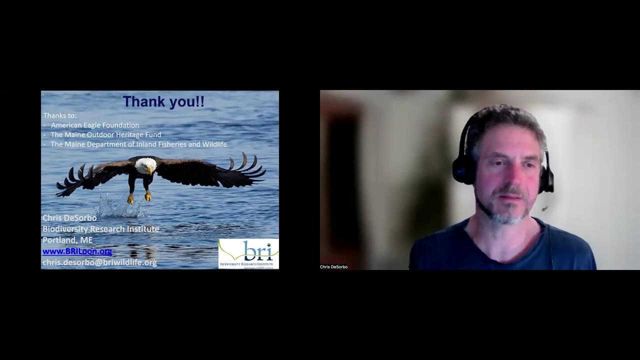 still in the area or is that like 80 percent of the time? they're still in the area, feeling fish versus you know, finding their own, or 50, 50 or you know, uh, any sense in the big picture, how much thievery goes on versus foraging on their own? um, yeah, i don't have any. i haven't. 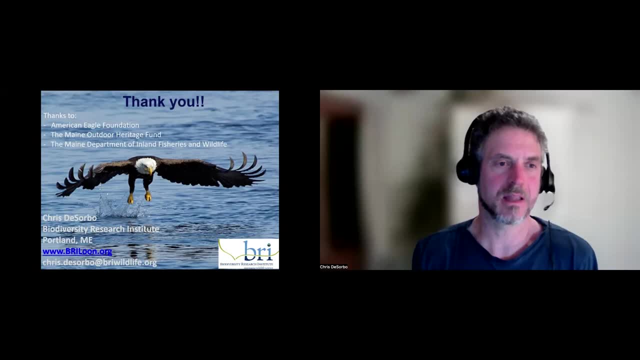 seen any quantification of that, but i will say that, like you are kind of alluding to, there's a- yeah, there's a real consistent pattern of eagles just just basically waiting for an osprey to catch a fish and then taking off after it and getting. 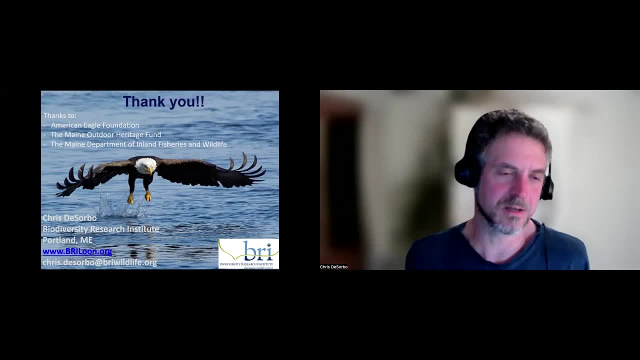 it to drop it um. and there's also, you know, clear cases like hog island um, osprey cam- that audubon runs in bremen area there, and miscungus bay is that um, yeah, i mean, the eagles will also come in and take young. so um they're. they're no doubt an adversary. 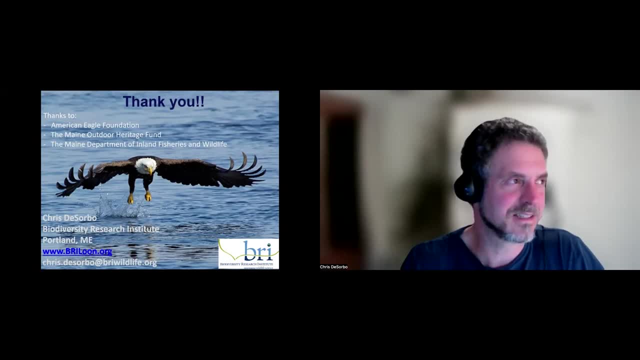 for sure how, how much it affects. you know how much of their time is spent. you know focusing on that versus other other approaches probably depends a lot on how abundant food is. if, if there's a huge fish run coming through and they can just stand and in the middle of a river and grab river herring, they probably might be less inclined to tangle. 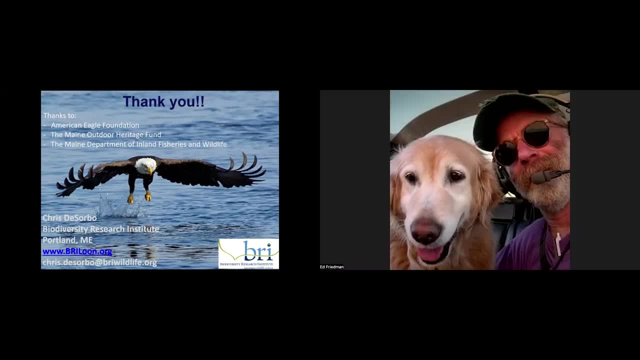 with an osprey, whatever. yeah, i think that's a very, very opportunistic. yeah, you know, i've seen over 300 eagles up there, you know, on the spas, when, when the fishing is good. but the seals are also there, and the great blue herons are there and the striped bass are there. so, um, it's a great picture of what. 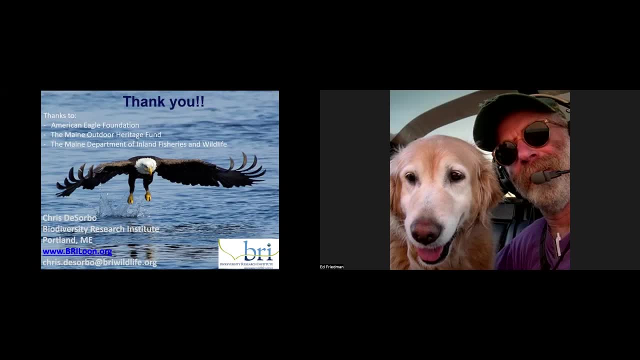 you know what wildlife could look like with river restoration? yeah, no doubt nick points out that you know, with the eagles frequenting landfills they must be getting a lot of uh toxic exposure and all sorts of you know household chemicals, other junk. any any thoughts on this? 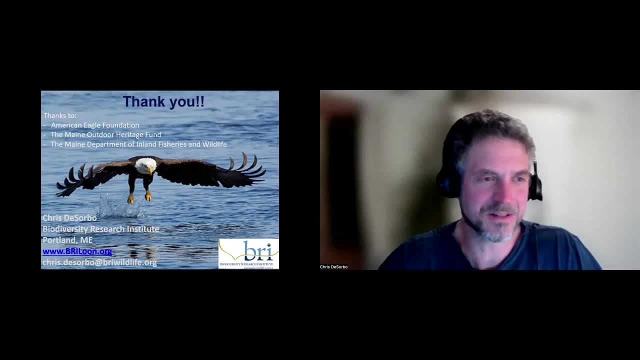 i would suspect that is the case. i would think there's all kinds of other risks in there too, of just ways to get hurt and exposure to all kinds of nasty stuff. um, yeah, there have been some great studies down in chesapeake bay that actually specifically looked at use. 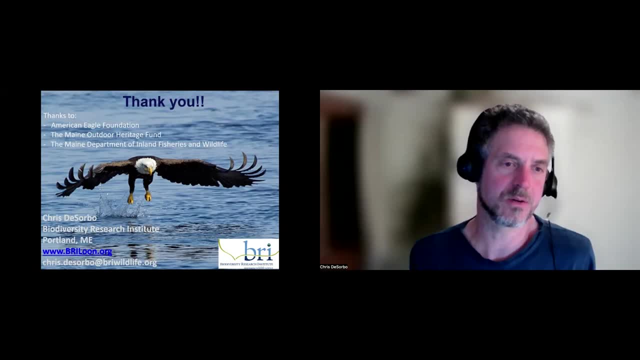 patterns relative to landfills, so it's not an unusual thing to do, but i think that's a great picture of what's going on in the world of fish, and i think that's a great picture of what's going on in the world of fish, and i think that's a great picture. 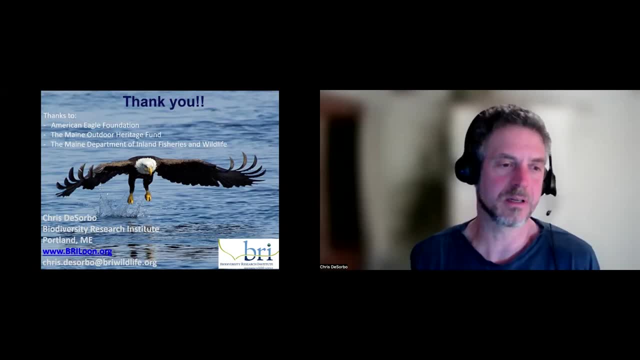 of what's going on in the world of fish, and i think that's a great picture thing. they're up at the press guile landfill and augusta. i don't know that anybody's ever captured those birds to sample them, though, so it really just becomes a practical challenge. 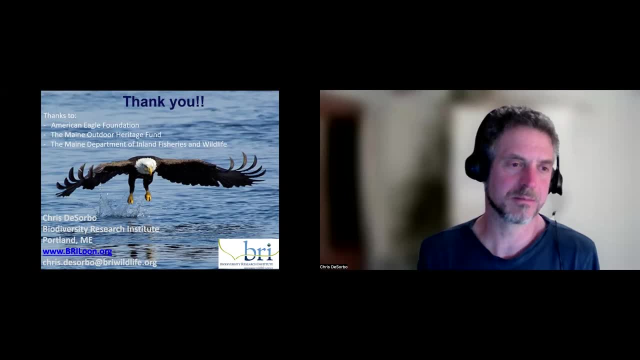 yeah, i know they're. they're in there and there's probably some clear management efforts we could take to lessen it. it's actually come up before william lea. what what about impacts on great blue herons in in the heron race for eagles? um, it happens for sure. um, yeah. 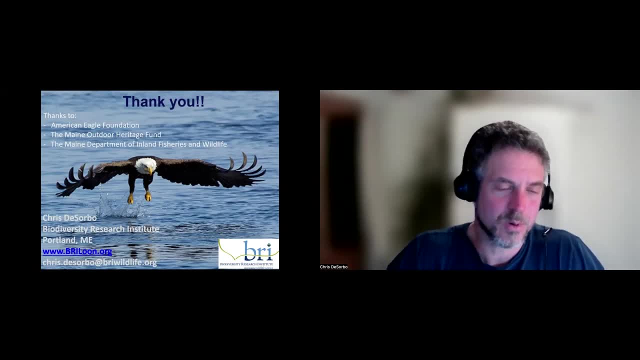 there's a a pretty concerted effort to survey great blue herons. that ifw runs and um, you guys probably know about that, but uh, yeah, eagles will have been known to cause full abandonment of some of the rickeries and i think some of the biggest rickeries in maine got splintered out, and one of 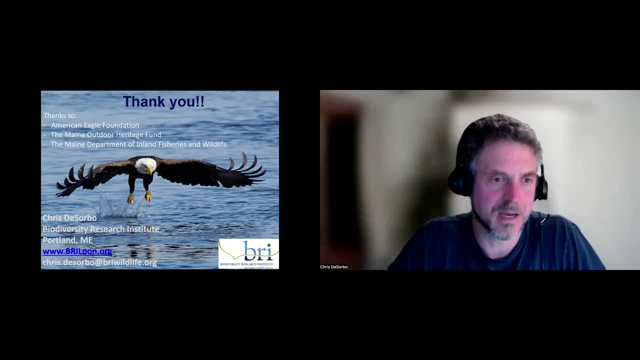 the reasons that were thrown out on that was that it was just eagle predation. over time that just was too much for them to bear, so now their nests are just scattered. but yeah, it's, it's probably significant same for you know, some, some of the seabirds there's a lot of, there's a lot of people. 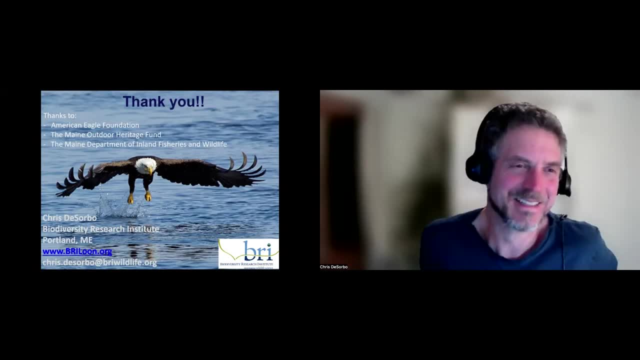 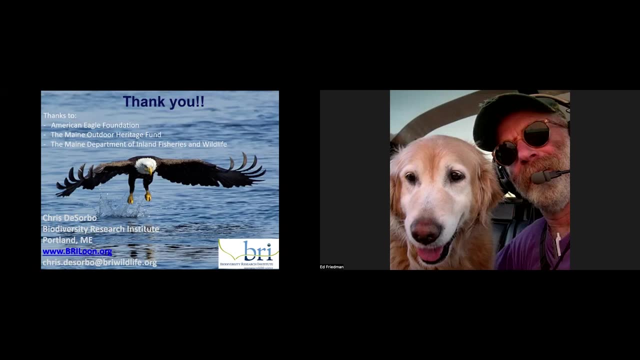 hating on loons, hating on eagles. the loon loon folks are among them too. a couple more questions. one um from michael watching eagles, you know. um cavort in the air very social, like um when they're doing their acrobatics, you know. 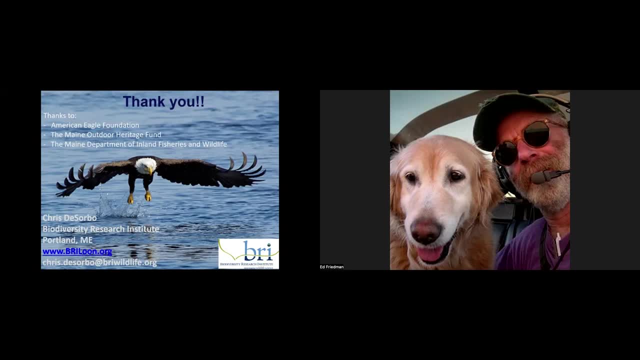 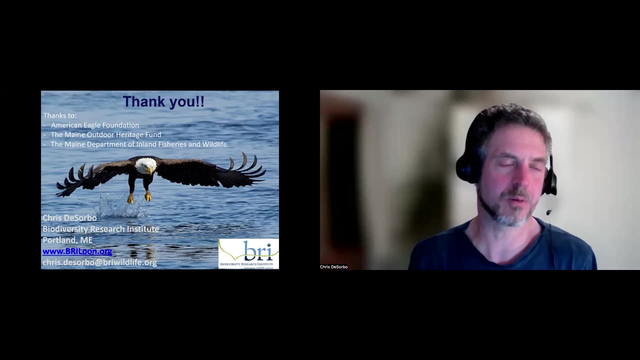 respond island or anywhere. um, can you elaborate on what they're doing? some of it's probably meeting, but are they just having fun learning, learning to fly? what's going on? uh, yeah, there's a pretty elaborate courtship, uh, that you, that people are probably seeing, if it's this time of year or a little earlier later on. 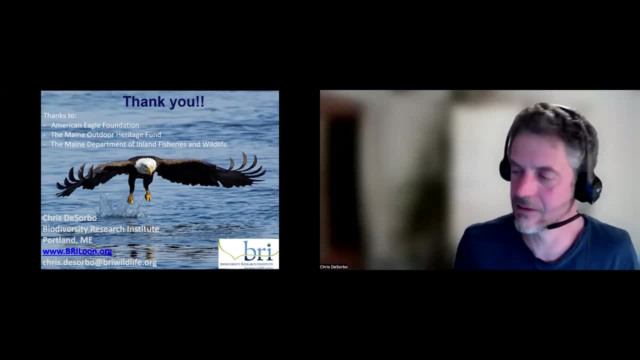 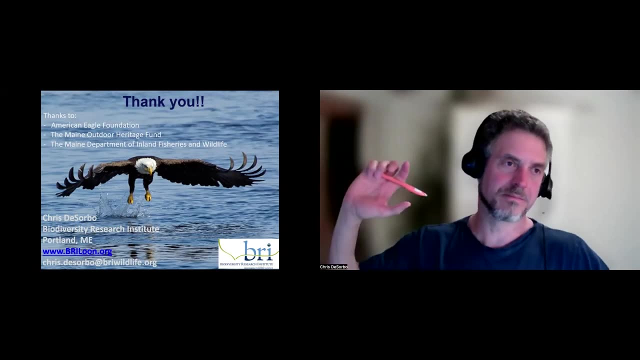 uh, i wouldn't be surprised if it's aggression. i think one of the things that people see in the wintertime is, you know, two eagles kind of locking talons in the air and just sort of tumbling through the air, um, out of aggression. but so you know the short answer: yeah, it's both. 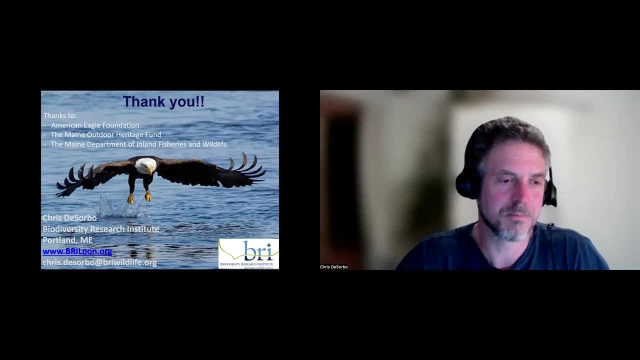 they're, these spectacular courtship displays, um, but there's also clearly some aggression going on, depending on what time of year as well. eagles are incredibly territorial over their, their turf, just like you know most birds, but they'll very aggressively fight it off from any intruders, and 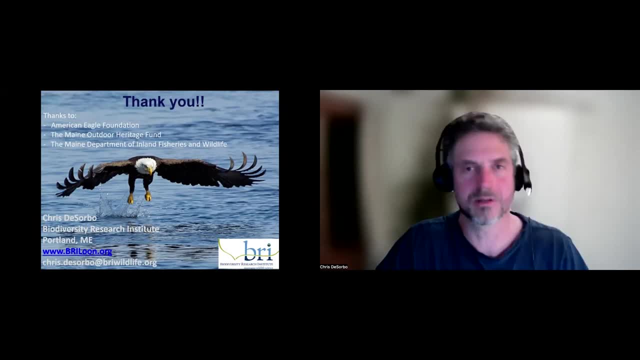 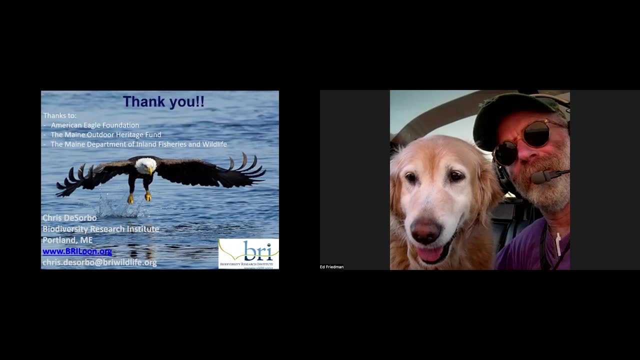 on occasion you'll probably see that kind of thing, although it usually just more looks like one chasing the other out. yeah, you know i'd have to agree with with uh michael, and that i've seen them so many times just flying next to each other and move for move, and you know, again it seems to. 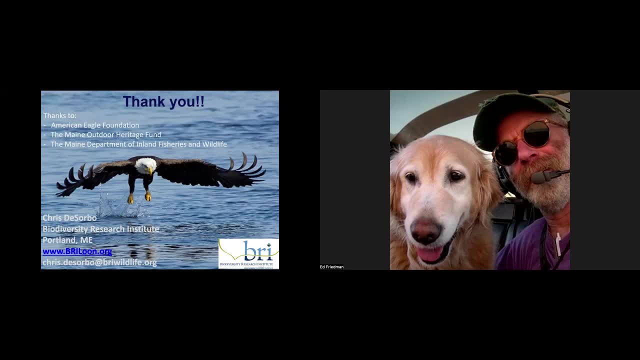 me more like a little bit of a flight training or just enjoying on a good windy day. you know, you see a lot of that stuff and i've seen all ages do it, so i'm not you'd have to convince me that it was aggression. you know territorial, you know um yeah, so anyway, um. last question, i think um. 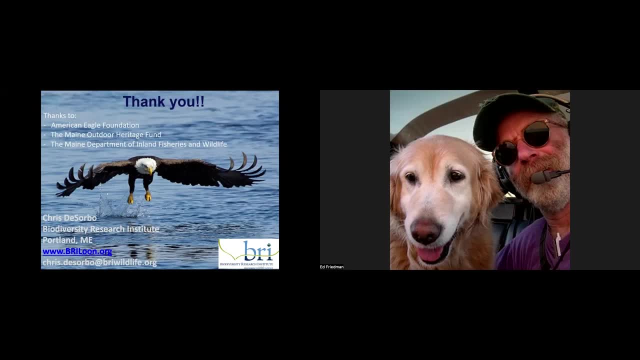 from my old friend john, who's in seattle now but used to live out the end of the road here, and why eagles tearing into fish from his bedroom window? uh, in pine trees? a good question here. um, if you could solve one or two remaining unknowns or mysteries. um, these are the eagles, of course. 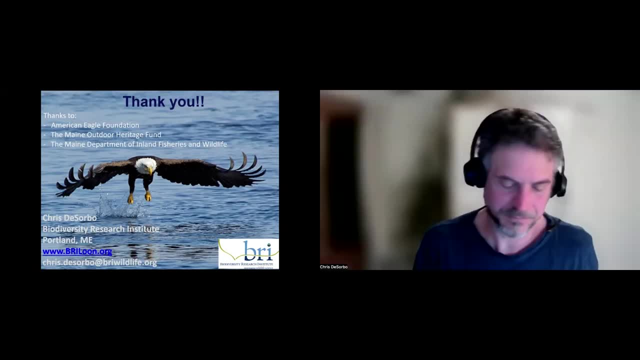 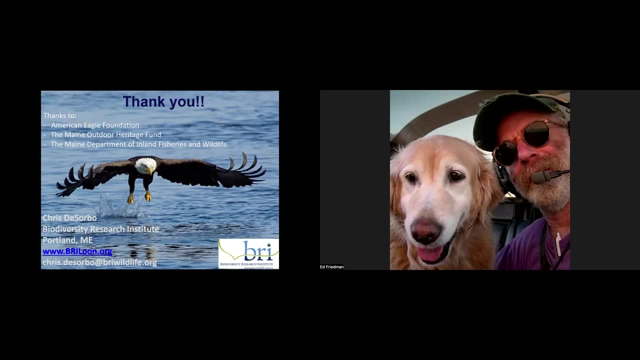 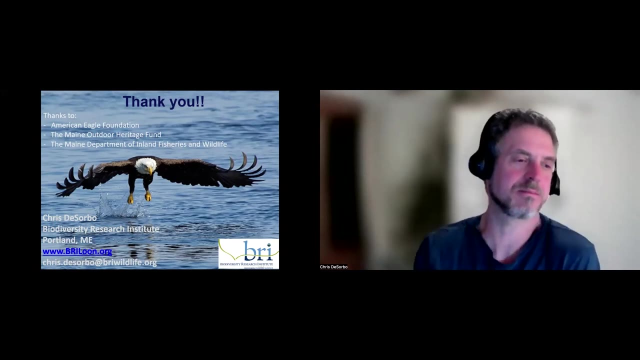 um, what would they be? boy, that's good question. um, well, i, i guess there's. you know, if you asked, you know somebody who's really steeped in the ecology of that particular species and the data gaps, like if you look at the birds of the world, account that, as far as just some. 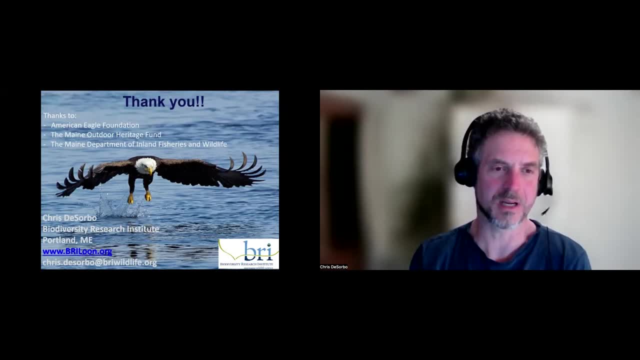 of the, you know, possibly esoteric but interesting questions. i think that's where i'd look to come up with some of those. um, personally, um, yeah, i feel like there's a lot that could be learned looking at um the incidence of diseases there. you know, we've actually started doing some of 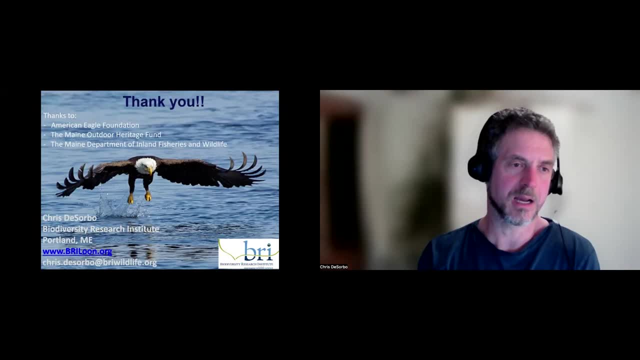 this work, looking at um, hpai- highly pathogenic avian influenza- um, and then a bunch of different blood-borne parasites. uh, i think there's a lot of interesting information in doing that kind of work. that is basically wide open. there's just so many unanswered questions. 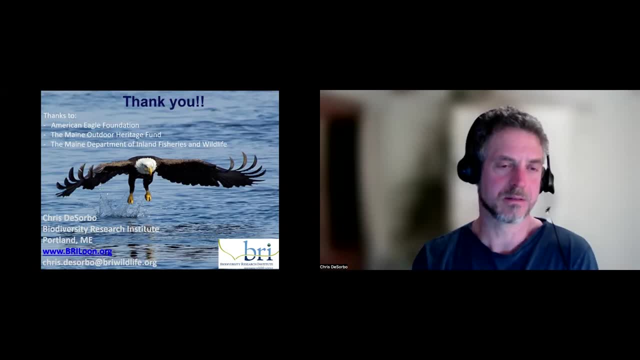 in that arena that have real relevance to to things. so i guess i would, i would throw that out there. um, yeah, i'd have to think on it. it is a very well studied species. i will say it. uh, you know a lot of the stuff that we focus on. 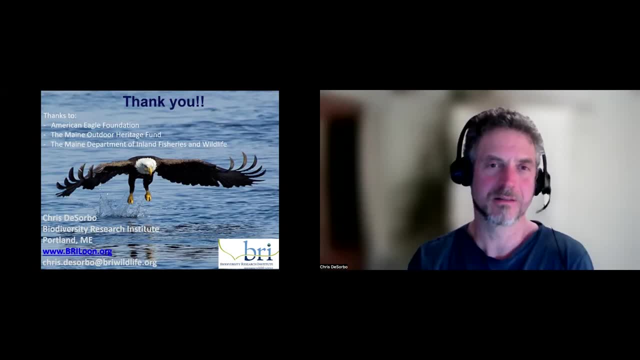 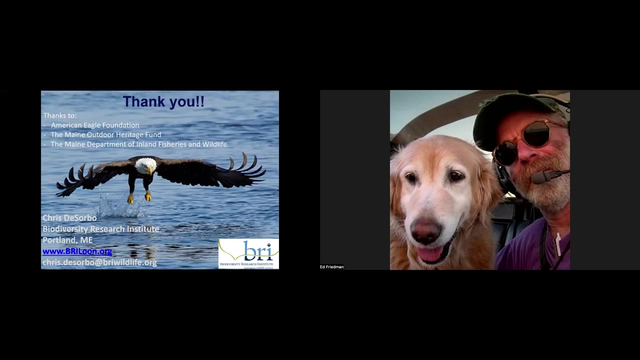 movement patterns and contaminants are, you know, low-hanging fruit for us, but um, but yeah that they're ecology. a lot of those questions have been pretty well established. okay, great, well, thank you so much, chris, i appreciate it and, uh, and that's a wonderful talk again for folks this will be. 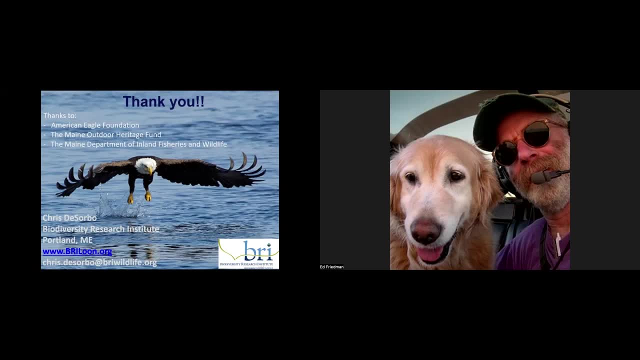 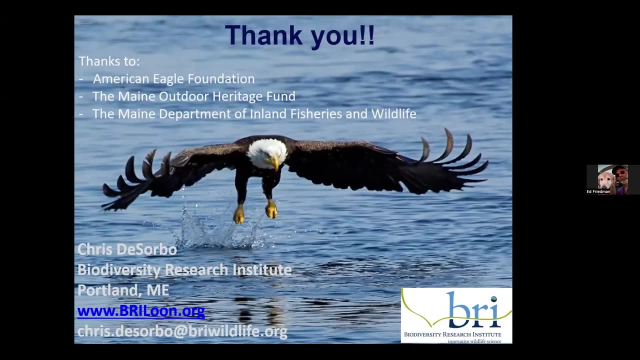 martin will have this uploaded to the website within a couple of few days or so and if you want to steer people to it, it'll be there down on the right hand column under education on our home page. so, chris, look forward to talking to you offline.